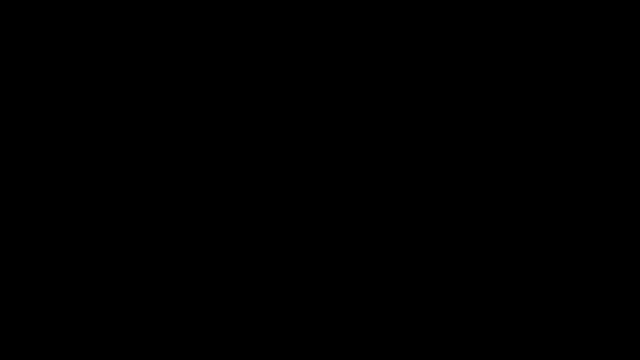 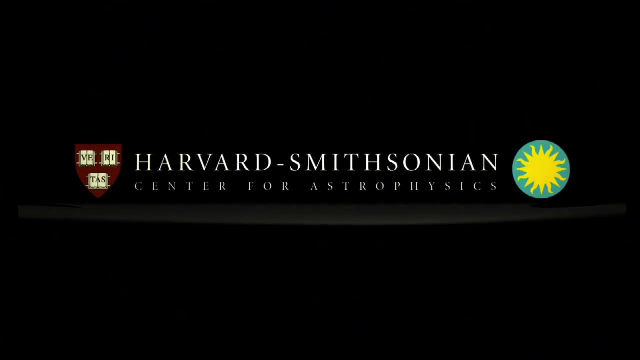 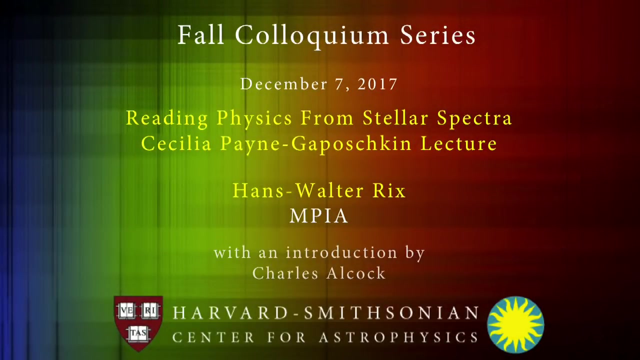 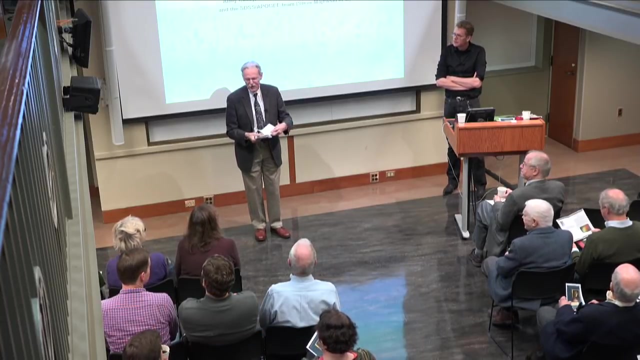 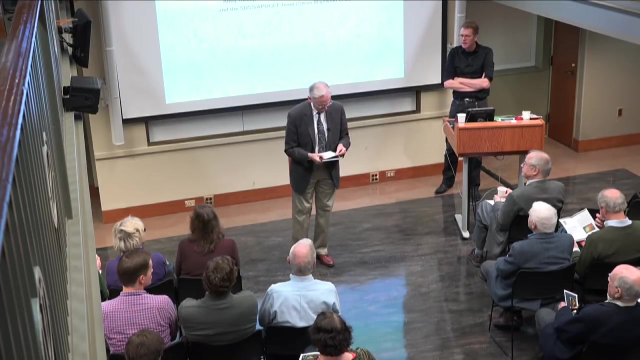 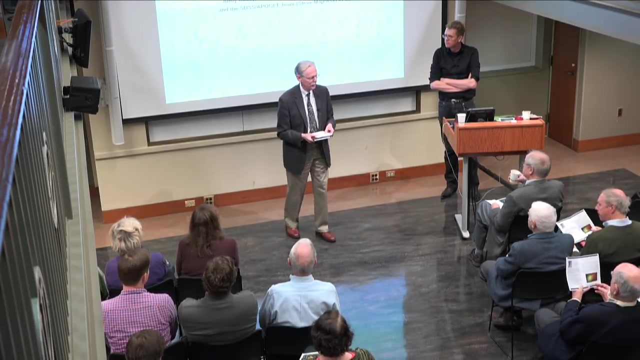 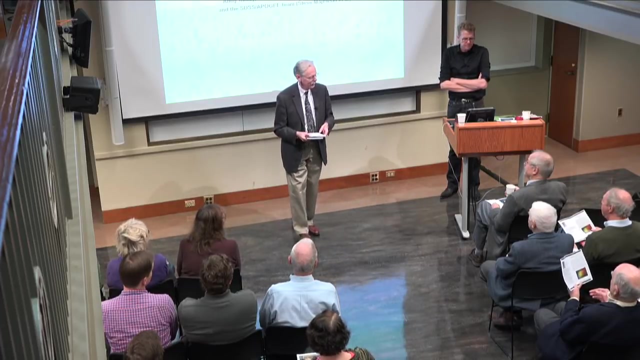 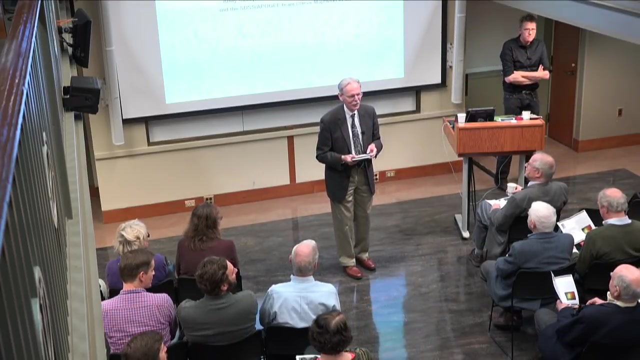 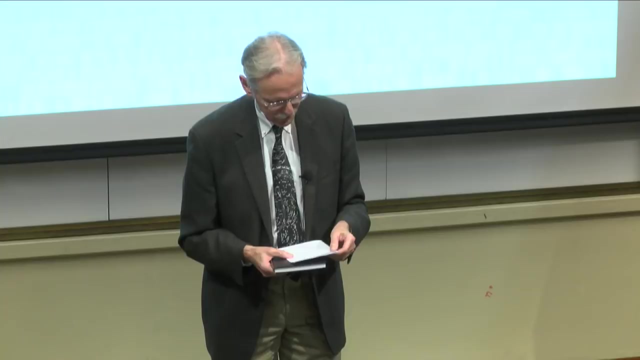 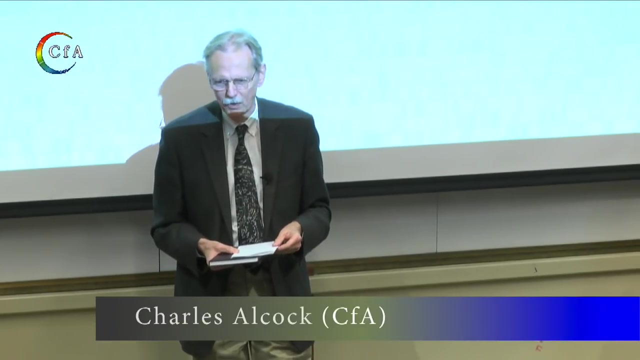 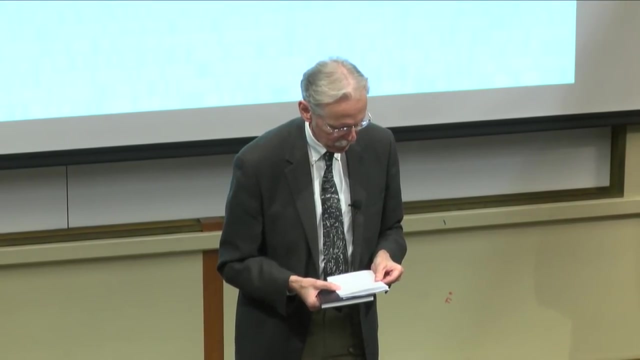 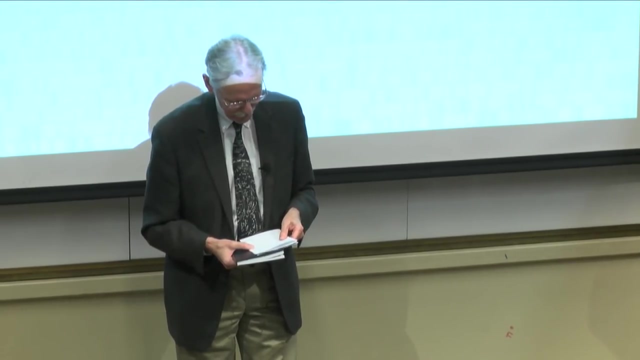 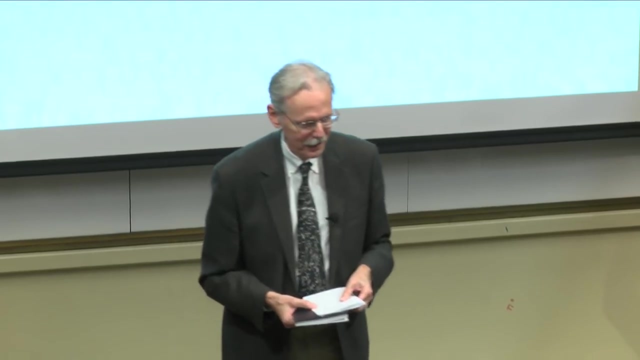 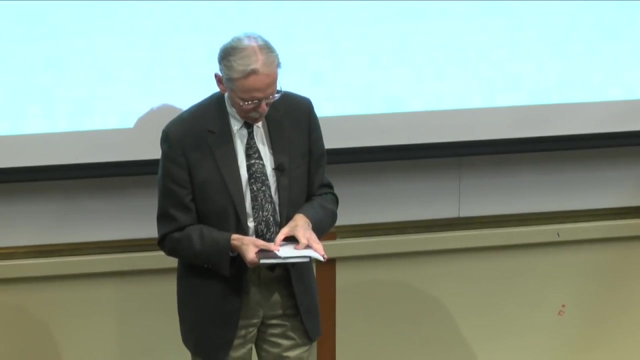 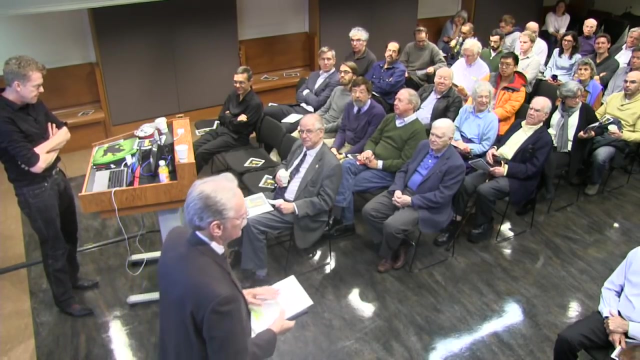 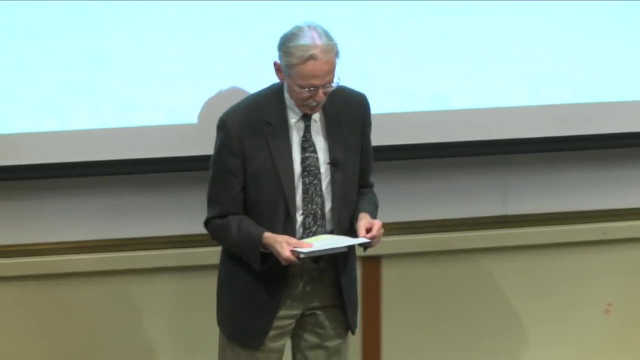 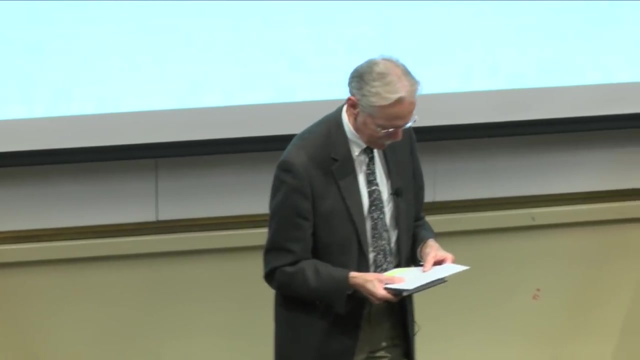 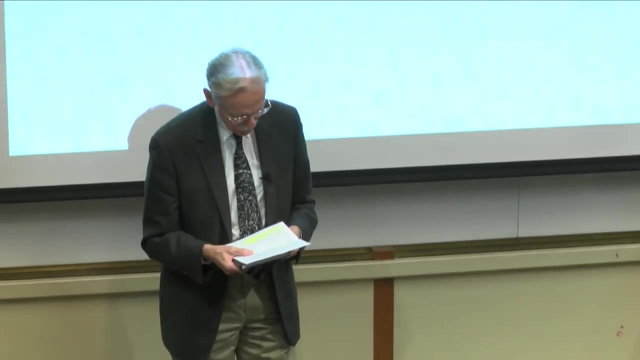 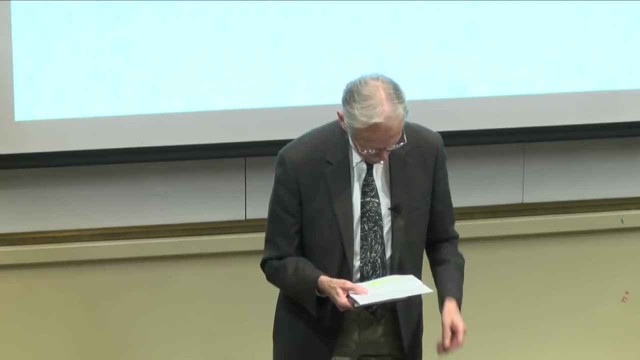 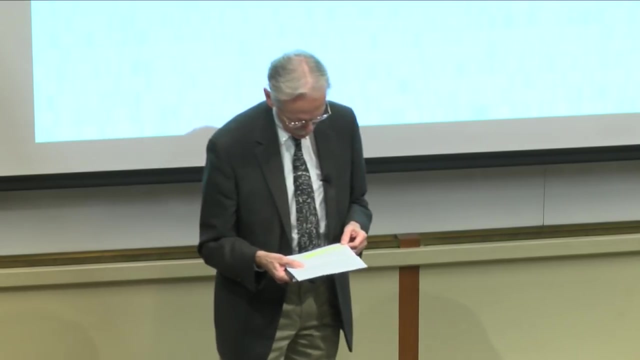 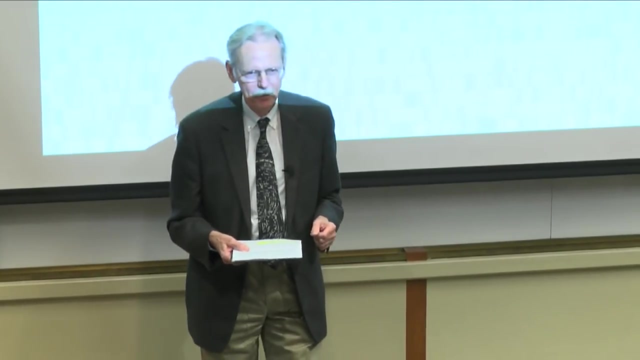 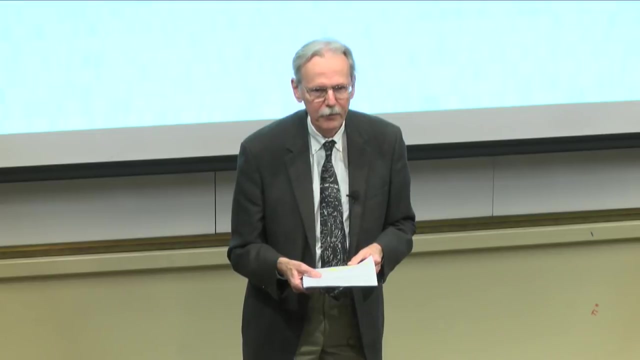 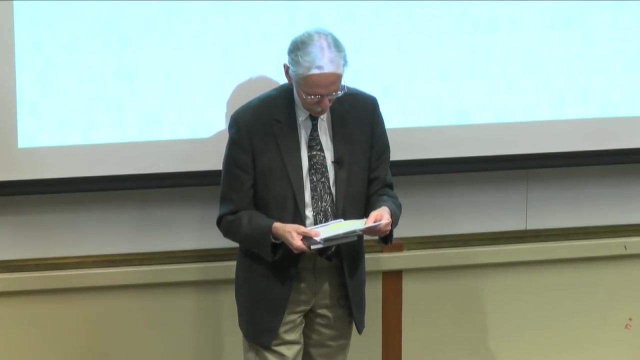 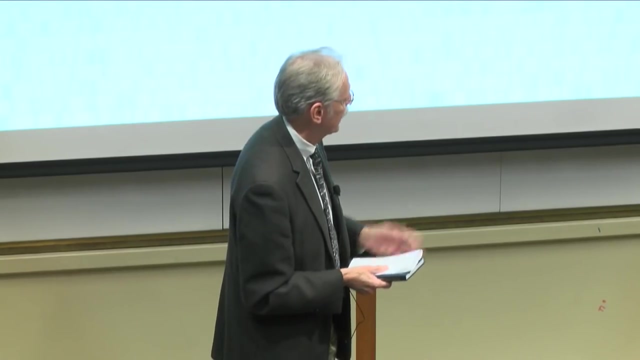 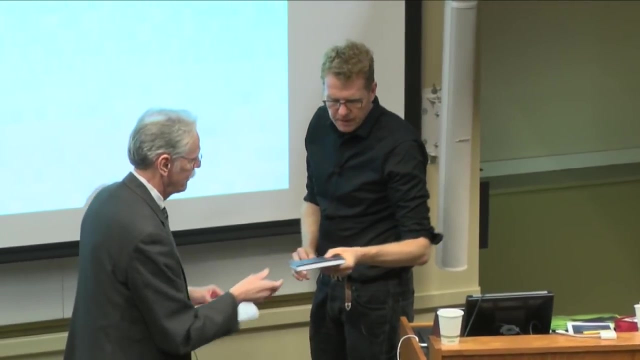 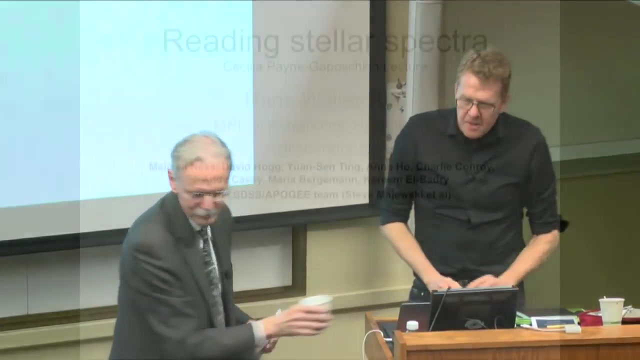 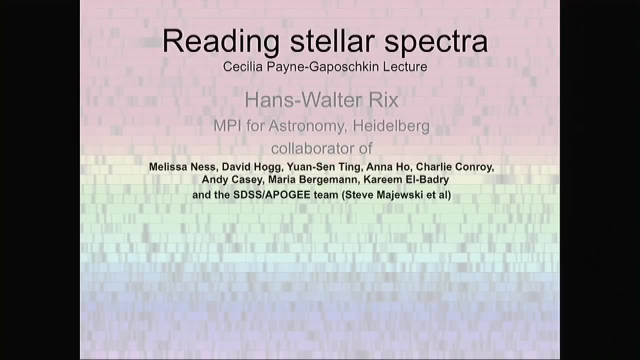 thanking you very much for this invitation. It is for me not only an obvious honor, it is also a real pleasure that it is a lecture named after Cecilia, because over the last few years I have grown very fondly of dealing with stellar spectra. 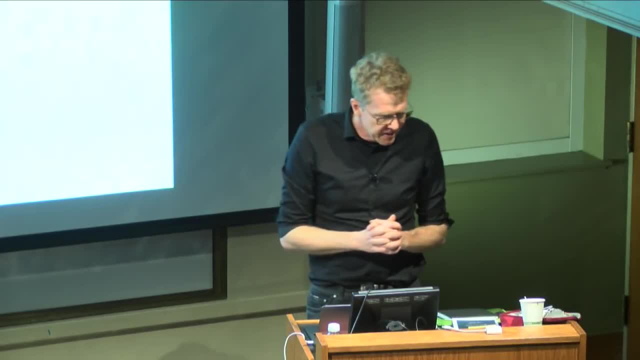 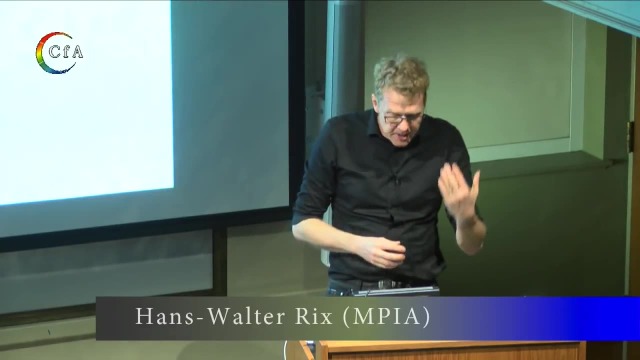 And so, while new to the field, I still think of myself as somebody who does it for the delight of it, a so-called dilettante. but now I can wear this, perhaps as a badge of honor, Before telling you my story. 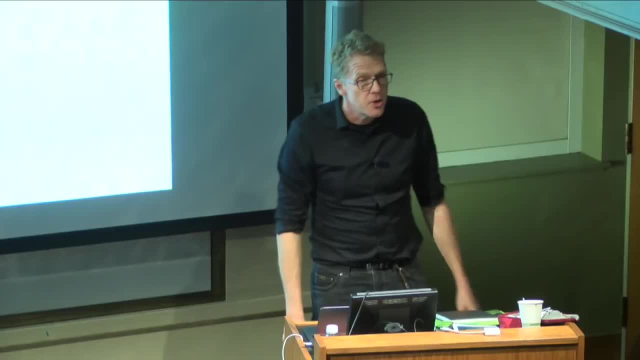 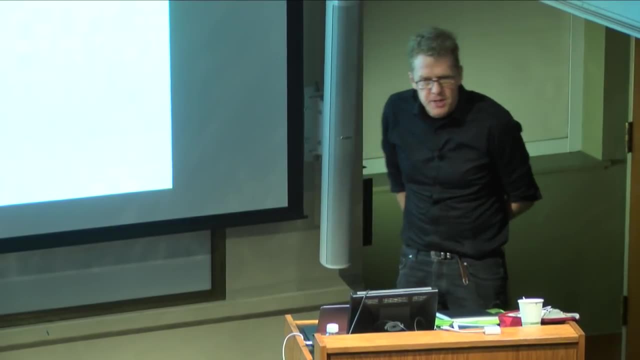 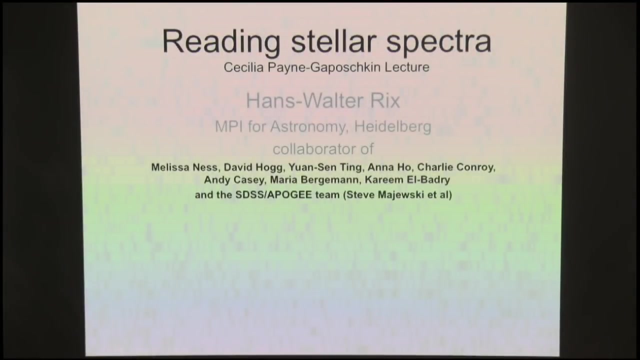 let me acknowledge that what I'm going to tell you, the work, but also the ideas, are in good part the product of my collaborators, my Heidelberg and New York collaborators, Melissa Ness and David Hogg, your local champions of the cause here. 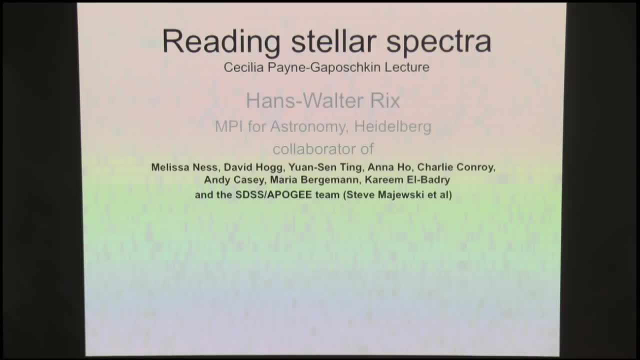 Yuanxin Ting and Charlie Conroy, and also Anna Ho, who is a grad student at Caltech now, And I also want to acknowledge the STSS Apogee team, who has produced a beautiful spectral data set which made what I'm going to tell you about. 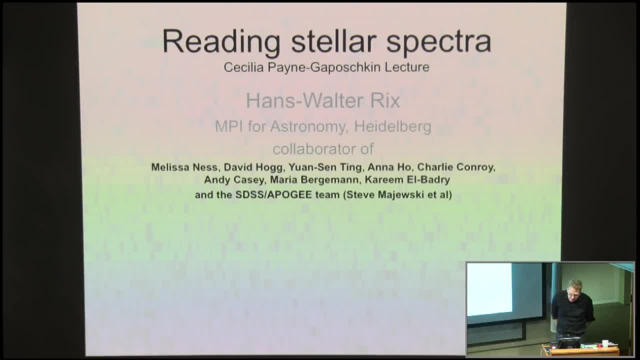 both the data set and the data set. So thank you very much. Thank you, Necessary and possible, So, but as somebody who spent most of his time working on galaxy dynamics and observational cosmology, I should perhaps say how I ended up dealing with spectra. 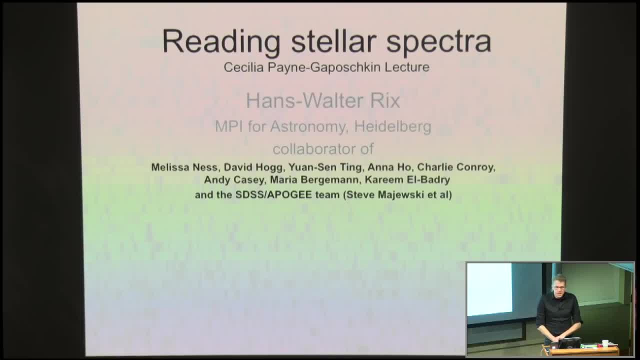 And I have two answers. The first one is by upbringing, The second by necessity, or perhaps even irritation. The upbringing is when I was a student, When I was an undergraduate in Munich. my world was simple. I thought there are two fields of astronomy. 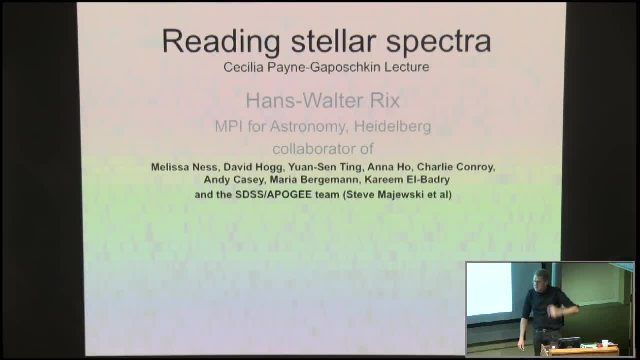 There is stellar evolution, which is Kippenhan and descendants. There's stellar spectra, which is Unseld and descendants. And so, as a Fulbright scholar, I was sent by Kudrytsky to Arizona to work with Jim Liebert on non-LTE stuff of hot stars. 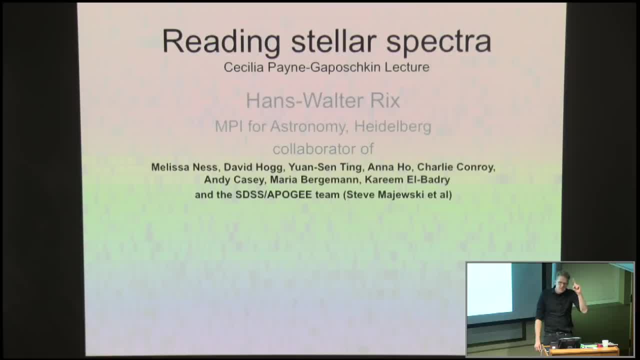 Jim said: now I don't really have time for a new student, but there's Simon White, this new faculty member. Perhaps you work with him. And so I was launched onto a 25-year arch away from stellar spectra. But the second answer, and why I say it was by necessity. 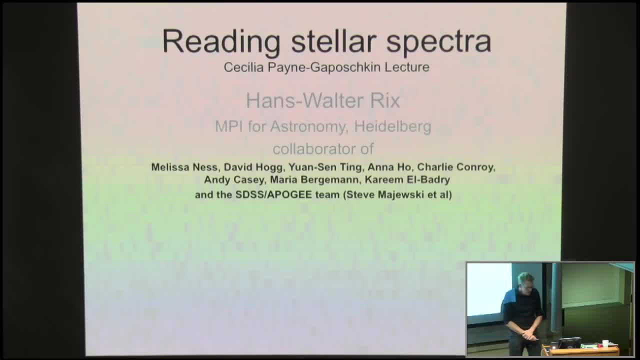 has to do with galaxy evolution. Right over the last decade and longer, there has been, in trying to understand galaxy formation in a cosmological context, an increase in focus or realization that many of the interesting and open issues lie on small scales, trying to understand really how galaxies work. 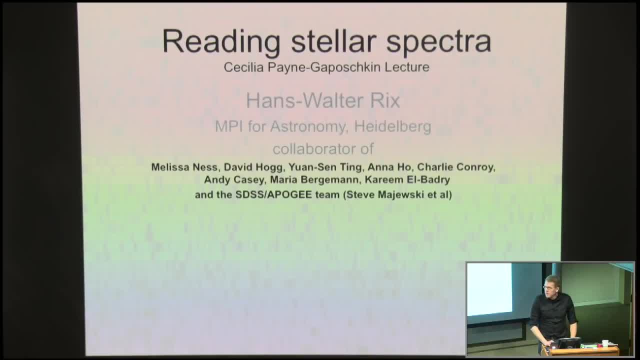 And there, of course, the Milky Way plays a special role. On the one hand, the obvious one, namely that it is beautifully resolved in its individual stars. Perhaps the other one also, that it is as I like to say. 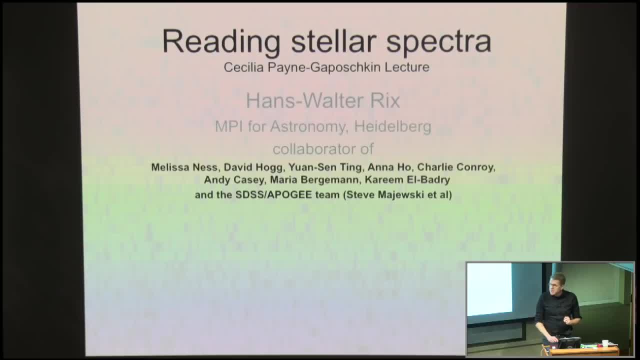 the Columbus Ohio of the galaxy world. It is really an atypically average galaxy in many ways, So we have the possibility, the possibility to learn from it things that are applicable to other things, And so it is said, the Milky Way in its stars. 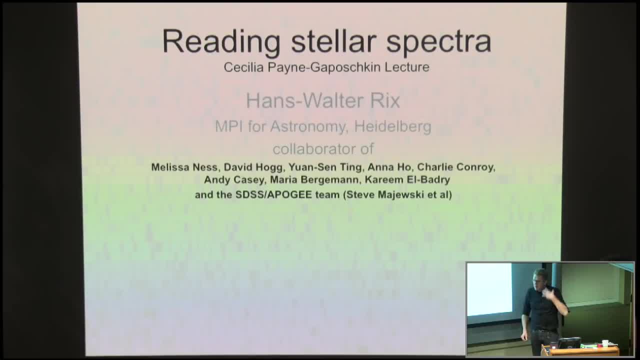 retains a formation record. If you could just figure out when stars were born, from what type of material, how enriched or polluted, depending on your point of view, and on which orbit, that would give you an imperative, a critical basis to see. 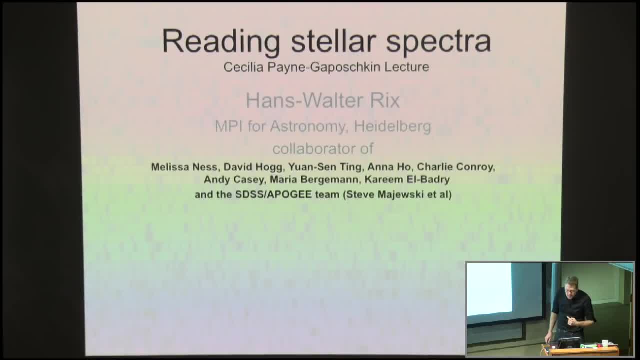 to just describe the formation of a galaxy and to perhaps understand it. And so really naively, getting into this first, I thought really all one needs to do is, all across the galaxy, construct and interpret the joint distribution of ages, orbits, composition of stars. 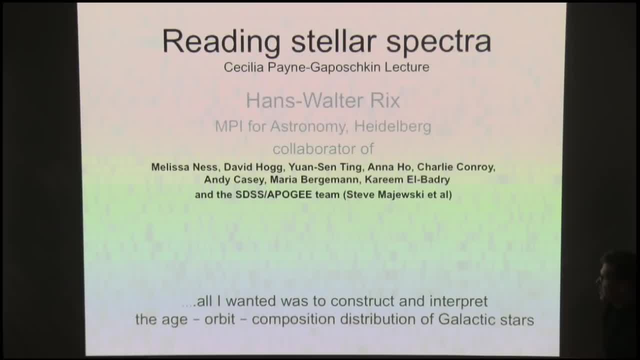 birth material composition of stars. And that is in some sense, if you had this, the ultimate observable which to interpret, Because, remember, while gas quickly forgets its prehistory stars, certainly their age is a lifelong tag. 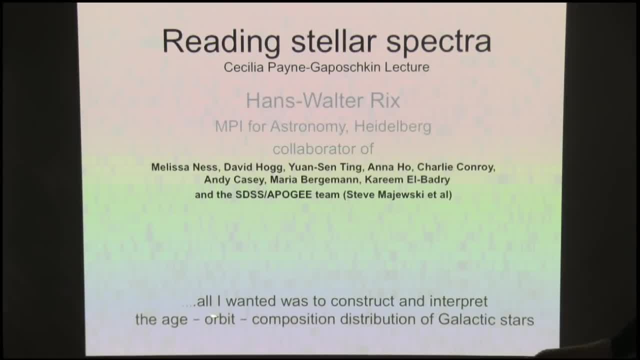 their surface composition, with exceptions also, And if orbits didn't change, then knowing that would be knowing the formation of the Milky Way. Of course, in practice it turns out there are many interesting things that change the orbits. So then the next thing. 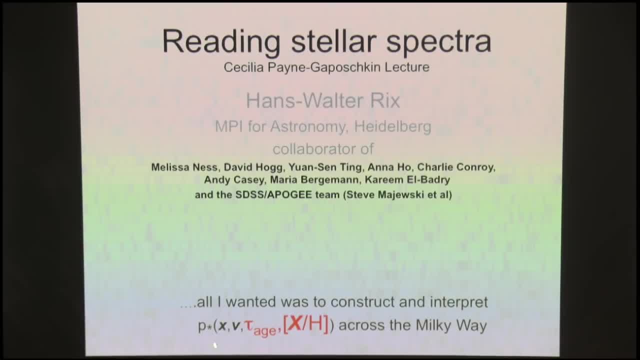 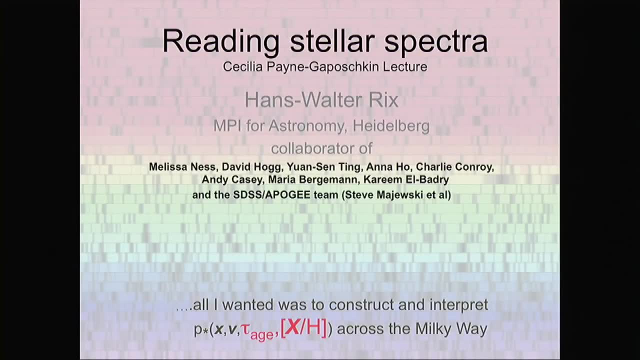 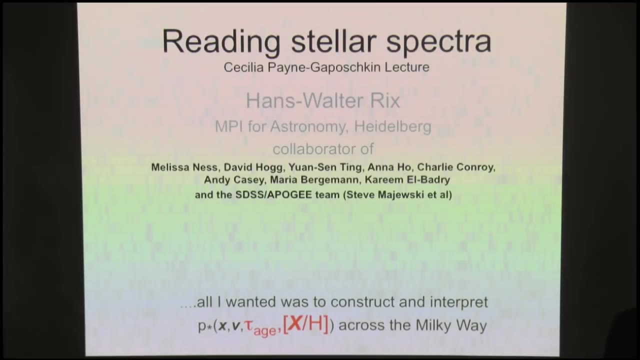 we realize. this is that actually to get to there, that distribution is really the position of velocity, and orbits are just an elegant way of encasing that. And then you need the element composition and their ages. Ages are, of course, a fundamentally important thing. because evolution means change with time. They're a fundamentally troubling thing because most stars are in hydrostatic equilibrium, which, by construction, means time doesn't show up explicitly. So just remember, you can't measure the age of a star if you don't have faith in stellar evolution. 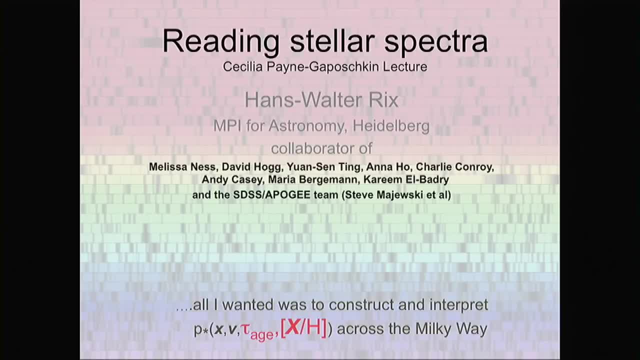 But let's presume you have faith in stellar evolution. Even then, it's very hard for many cases to actually measure ages. So and then I started making plots of such quantities, and every time something interesting came up, I talked to a certified spectroscopist. 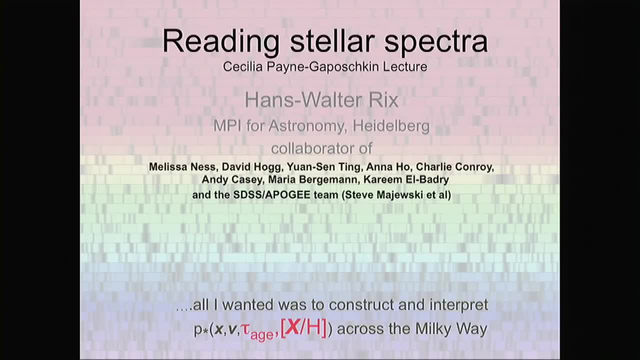 He said, yeah, but you can't quite believe that. So there was actually. you know, everything that was away from the unusual was tricky. I tried to combine data from different surveys. They were clearly inconsistent and there was very little information about ages. 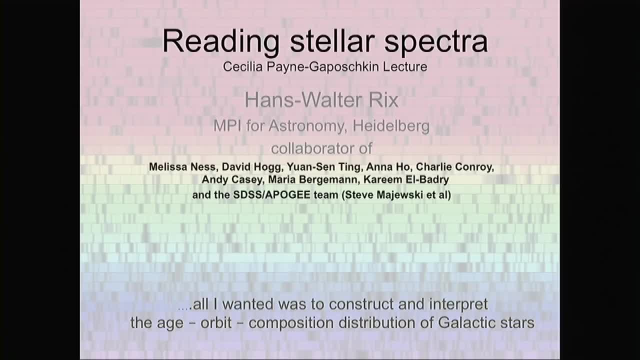 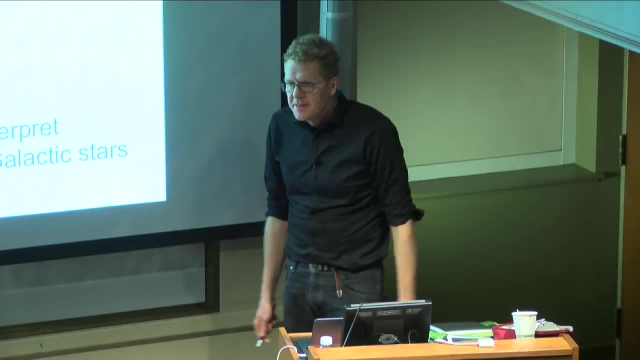 So that is where necessity, at least for a while, became frustration, And so what I want to tell you about is some of the things my collaborators and I have tried to do over the last years to overcome the practical difficulties. So we'll talk a lot about practical stuff. 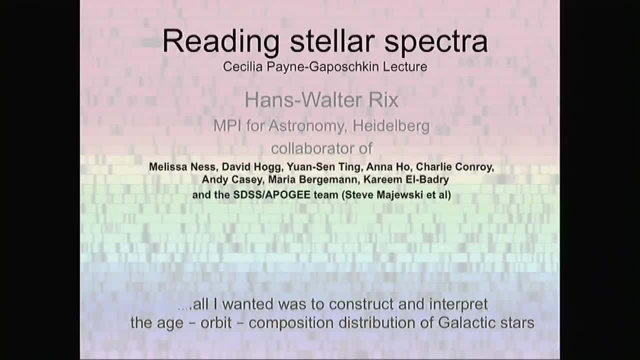 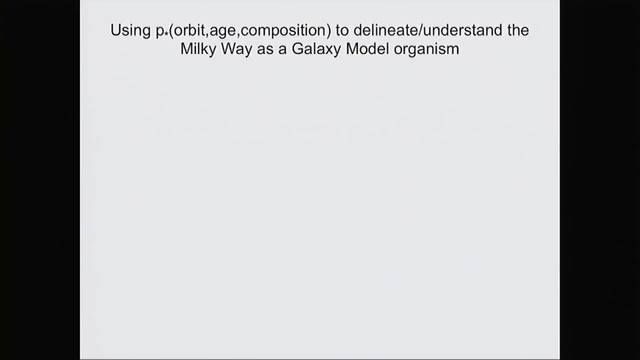 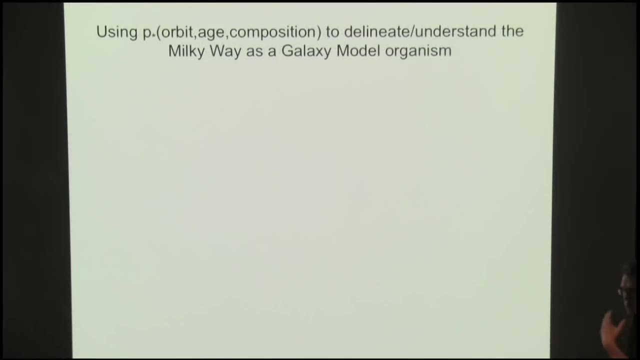 to work towards this. Before I do that, let me actually just give you a preview in my particular motivation. What if we had solved this problem? And what I will show you is because we have made progress in partially solving this problem. 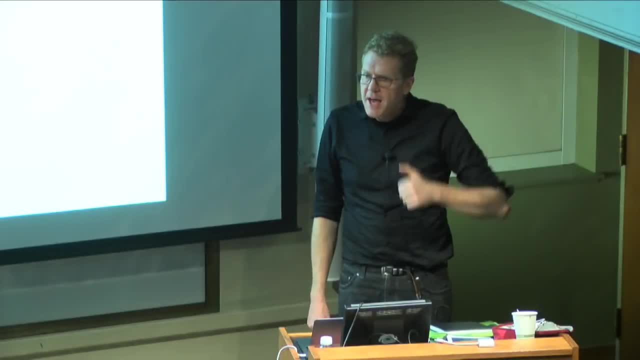 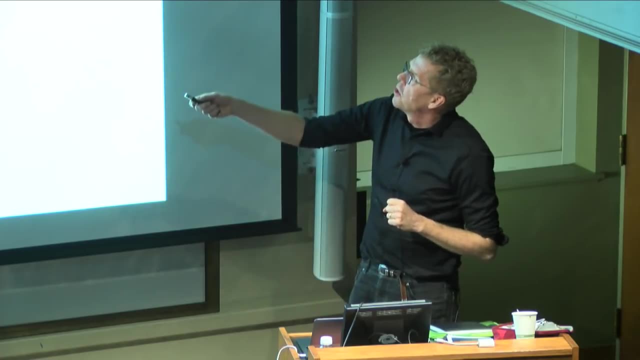 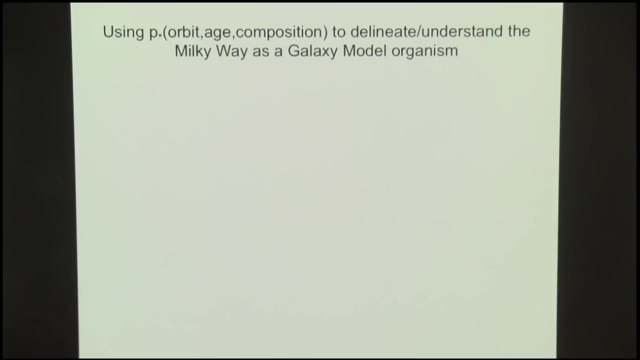 what if, across the entire galaxy, you had sensible estimates of stars, of the ages and at least some basic abundance numbers? So before the Gaia mission next April, I will only talk about positions in orbits. So that's one limitation. 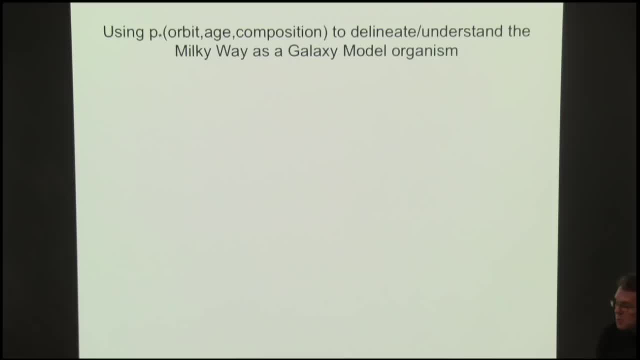 but let me just show you what one can do, and I will tell you where the ages come from in the course of this. So let's perhaps ask the most empirical question first. can we just map the productions of elements across the galaxy? 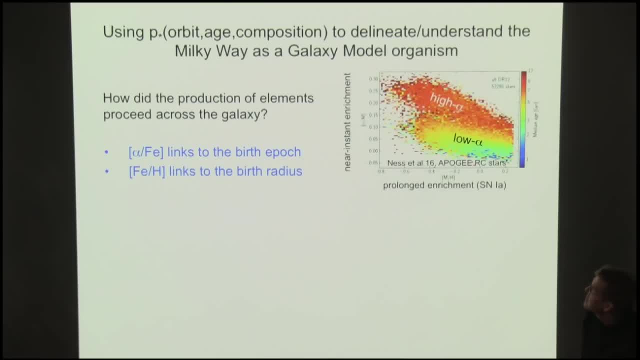 And one thing that the Apogee survey has allowed us is actually for red clump stars, whose 3D position we know across much of the galaxy, estimate their ages, and then you can do that kind of a classic plot: ask: how does the abundance of stars here? 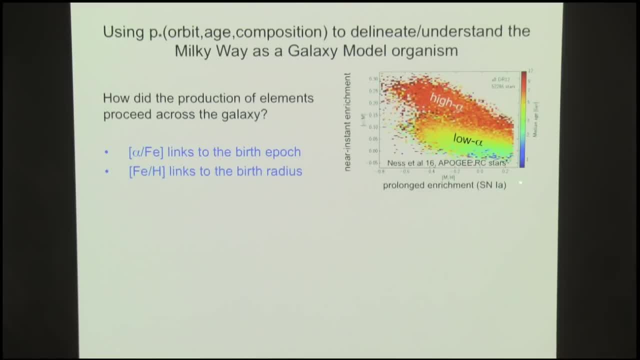 metallicity, essentially iron and alpha enhancement relate to age. So this is an axis of near-instant enrichment and this is of delayed enrichment, And so, at some level, what this plot shows in color-coded is age, if you measure. 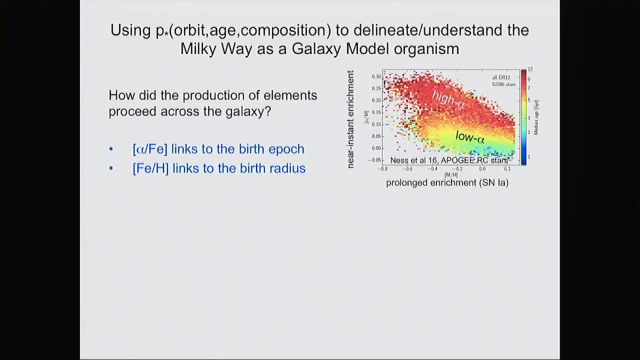 and that's a traditional thing to do. alpha enhancement, that is how much rapid enhancement has happened. that is a good way of estimating, meeting ballpark, the age of a star. All the very strongly alpha-enhanced stars are indeed old for the most part. 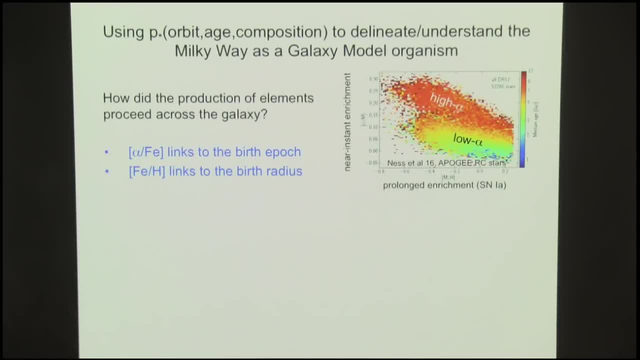 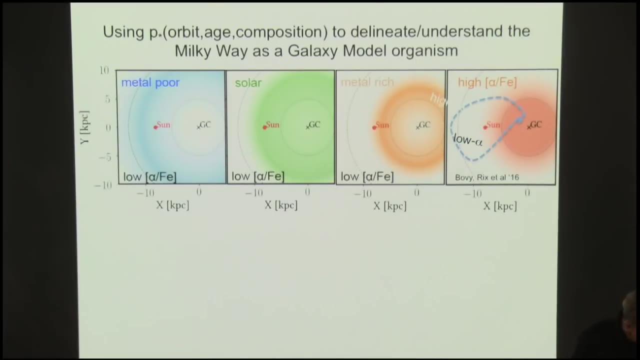 Metallicity is a funny, complicated story. for the bulk metallicity of the galactic disk And we'll mostly actually talk about the bulk of our Milky Way- At any metallicity you can find almost all ages, And this is. But actually metallicity has a very 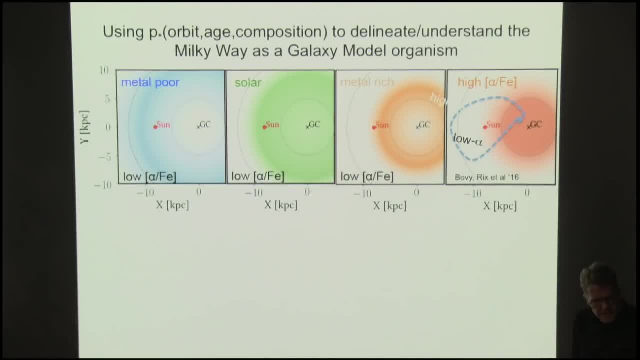 Interesting story there, And that is a plot that deserves slow walking through. Let us start here. What this shows is using information from the Apogee survey, And I've shown here what in this pseudo top-down view of the Milky Way. 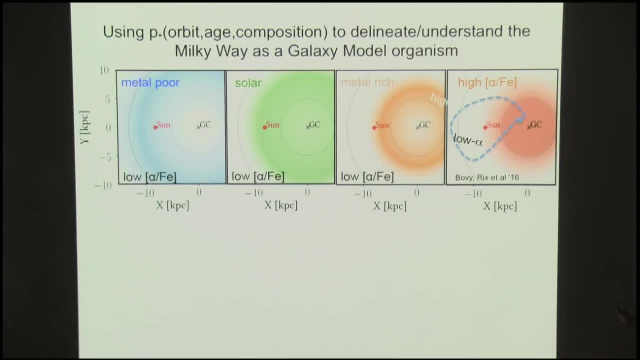 the actual survey volume is. You may not be impressed by this, but this dot alone would greatly exaggerate the volume that the Geneva-Copenhagen survey at some level- the state-of-the-art survey a good 10 years ago- constituted when it came to this. 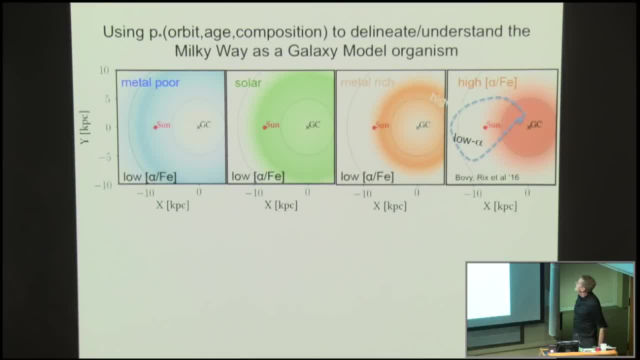 So if you make global maps and these just show the density of such stars from a model fit the first thing you see, the old alpha-enhanced stars actually are very centrally concentrated. We sit at the outer tail end And actually across the Milky Way. 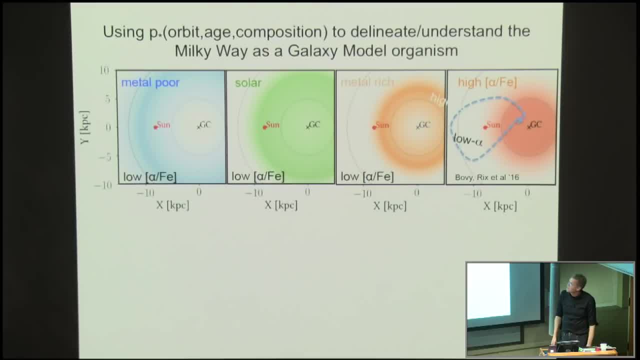 half of the stars, almost half of the stars, may be alpha-enhanced. So if I had asked you, you would look directly down on the Milky Way and only have eyes for high solar or sub-solar metallicity stars that are not alpha-enhanced. 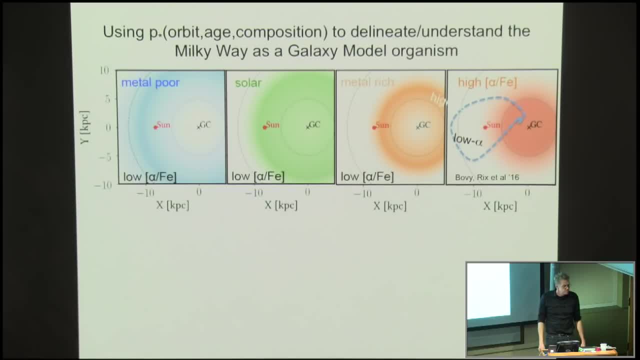 Turns out, the Milky Way looks like a bunch of donuts, That is, the middle-rich stars really live at a characteristic radius and their abundance tapers off. So there's an exponential rise and exponential fall-off. And if you take a look at the Milky Way, 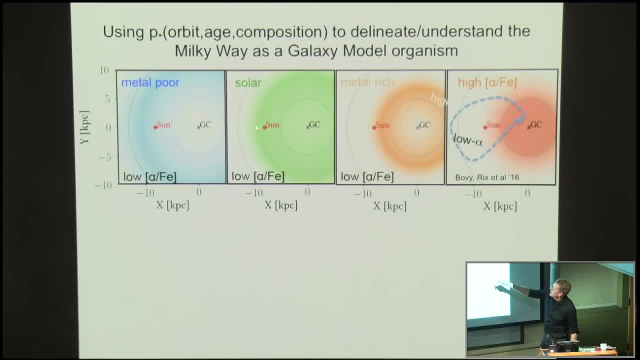 you'll see that the Milky Way is like lower metallicities: The same pattern holds, except shifted outward. So the way to think about this is apparently: imagine there is a special radius, a chemical equilibrium between enrichment and fresh gas inflow forms. 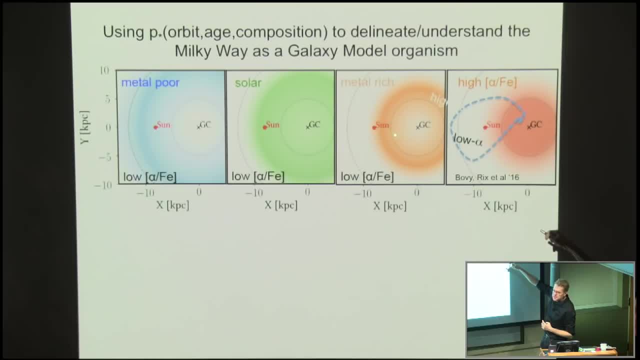 So stars of a given metallicity always form at the same radius And more metal-poor ones form further out. But then these stars are actually wide, So perhaps it is not quite rigorous. So you don't have strict mapping between. 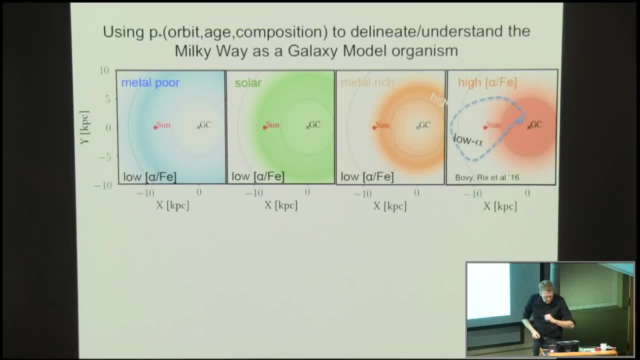 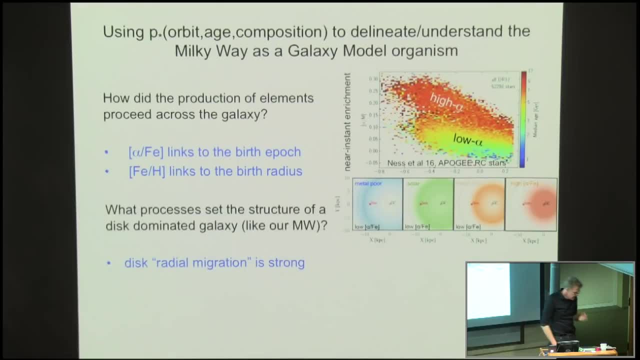 present-day radius and metallicity, But the text before said perhaps between birth radius and metallicity. So let me show you what that means, because that actually also shows you a new insight, or relatively recent insight, of what the Milky Way looks like. 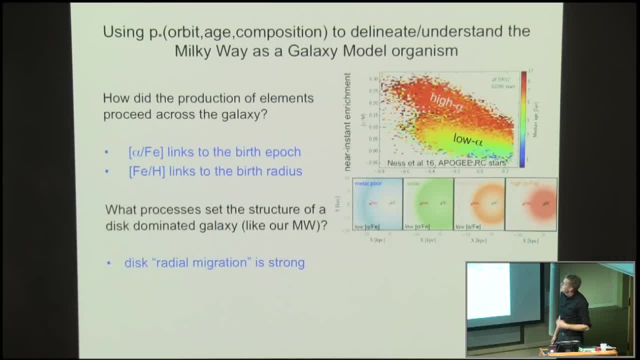 What matters in setting the structure of our disk. So it used to be that stars were born in circular orbits. Then molecular clouds came by and heated them that-a-way and that-a-way and they got on more eccentric orbits. But in some sense, 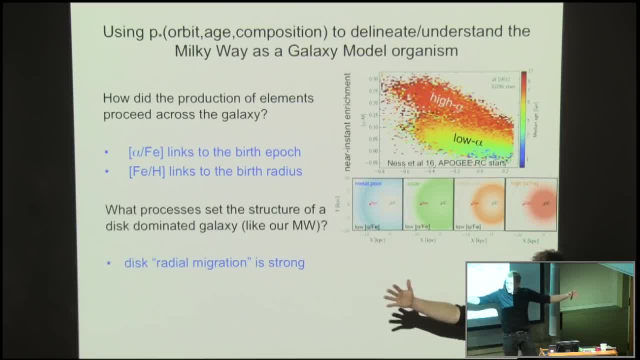 there was no obvious mechanism that would make them drift by large amounts in radius. So James Spinn and Jerry Selwood pointed out about a good 10 years ago that stars, stars, surf on spiral arm patterns- a process called radial migration- and they may change their radii. 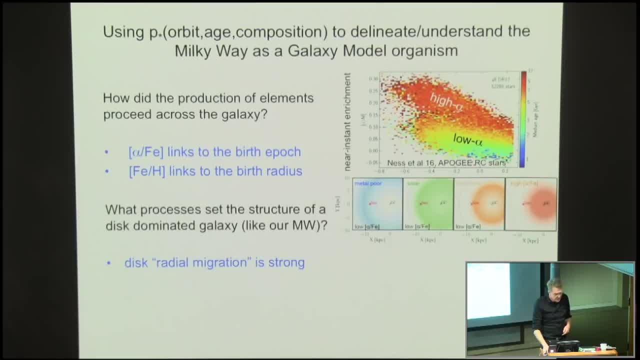 by a long shot without actually becoming eccentric, And now we can actually see whether this is only a minor perturbation or something. If you sort these stars, take all the young ones, and if you take even the younger ones, you get a beautiful relation. 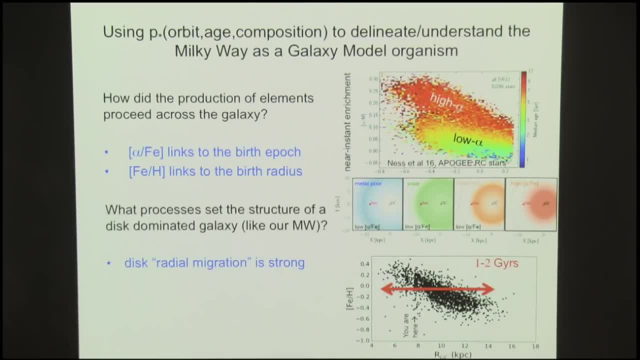 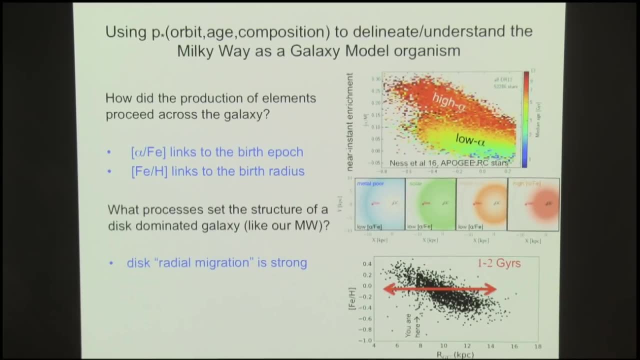 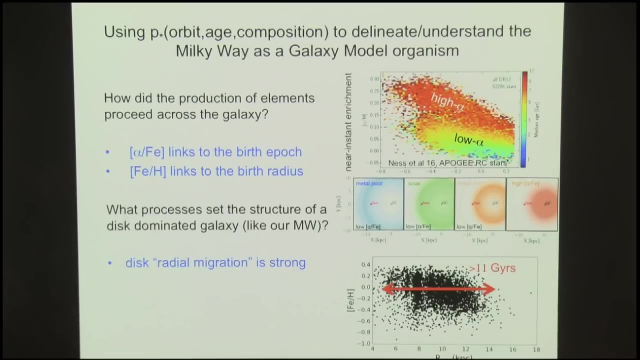 between metallicity and radius, But you don't actually get a. you know they can't change their metallicity, but let's presume they radially migrate. If you look at the old stars, it's well known there is no relation between radius. 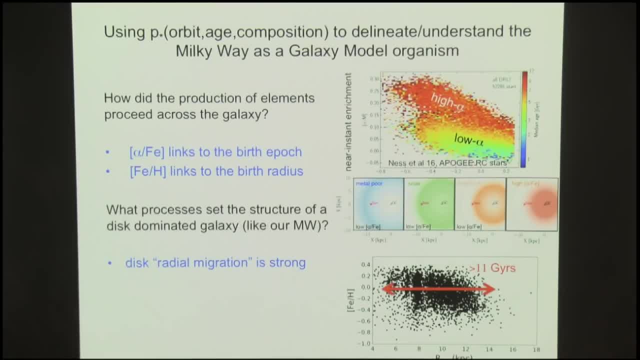 and between metallicity, age and radius. So you can actually model this process and find that these data tell you that stars have drifted over their lifetime, typically in the Milky Way, by about a half-mass radius of the Milky Way itself. 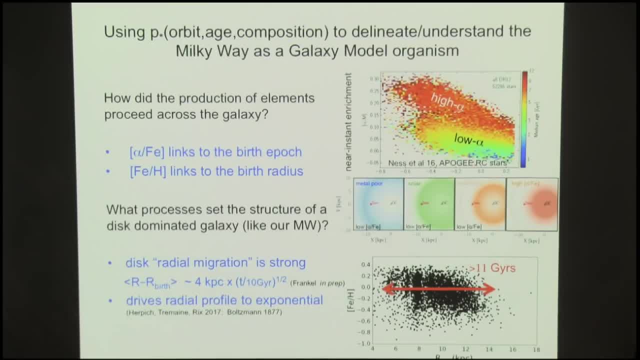 And one of the things that's interesting is if you ask what is the limit of maximally scrambling angular momentum, It is an exponential distribution which we thought we had figured out recently, but you know, other people of course have done before. 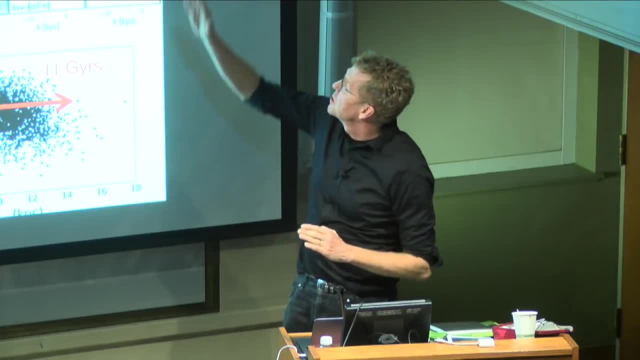 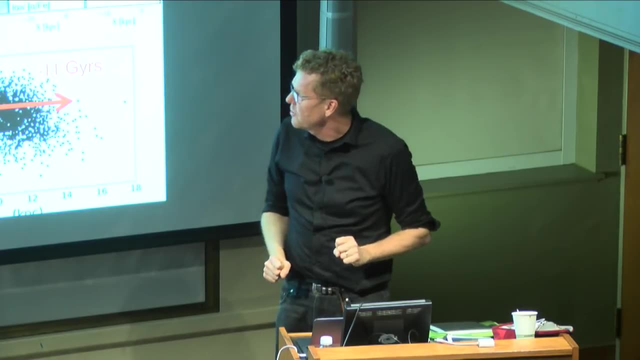 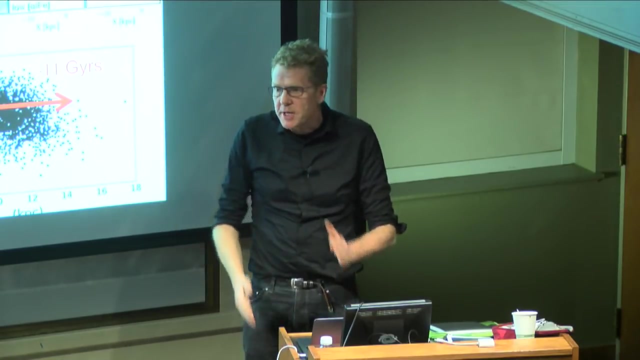 So if that's you know, this story would say there was an early phase of alpha-inanite stars, rapid star formation. as the Milky Way settled down in star formation you really had chemical equilibrium at each radius stars of a given metallicity. 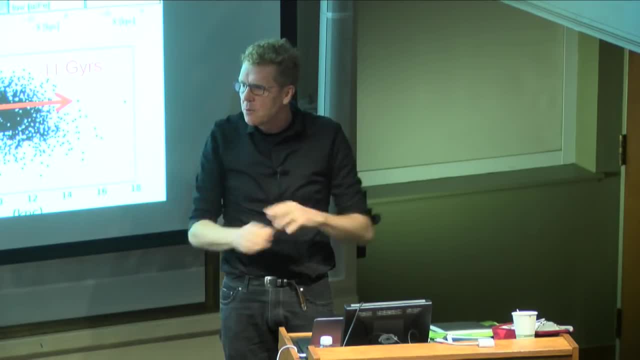 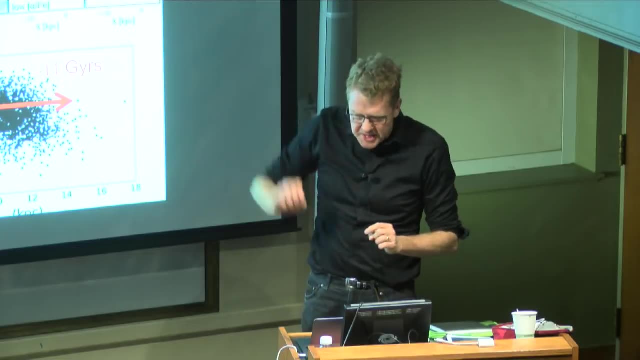 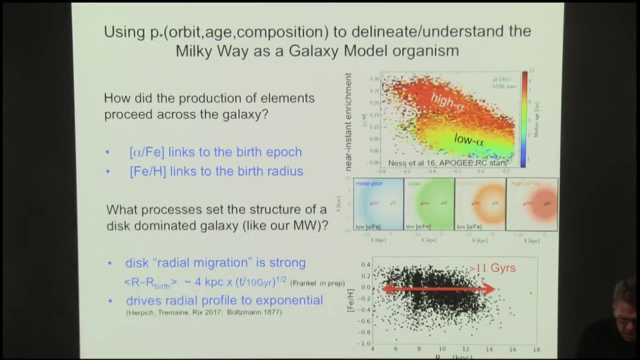 were formed at a given radius and then drifted away, which smooths everything out towards an exponential. So that is. you know, this is a sketch of what you can do if you have this distribution all across. So part of what 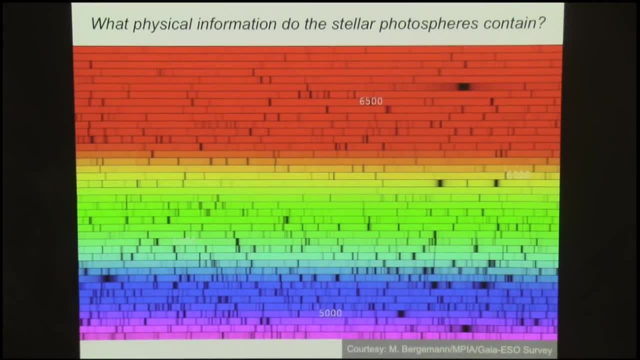 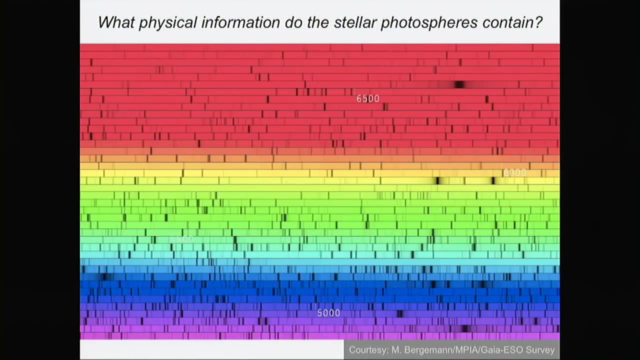 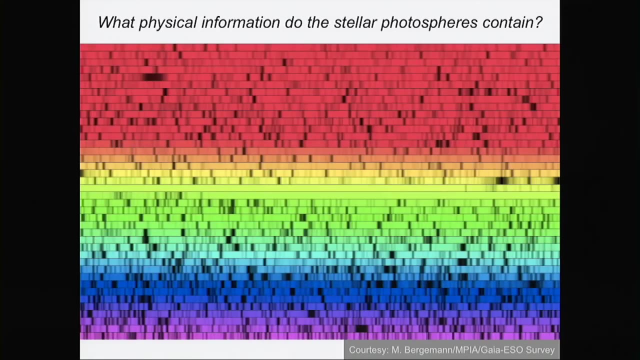 I will tell you now is where those ages come from. but that brings me towards really the core of my lecture, namely: you know, what can you read of those spectra? I've given you my personal take. I would like to just get out. 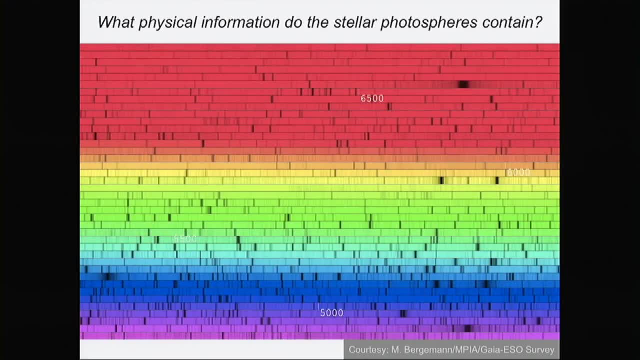 a couple of numbers which I can then use for galaxy evolution, but let me just remind you that obviously it's an interesting astrophysical project in itself explaining that, and there are also immensely good diagnostics of the stars themselves. 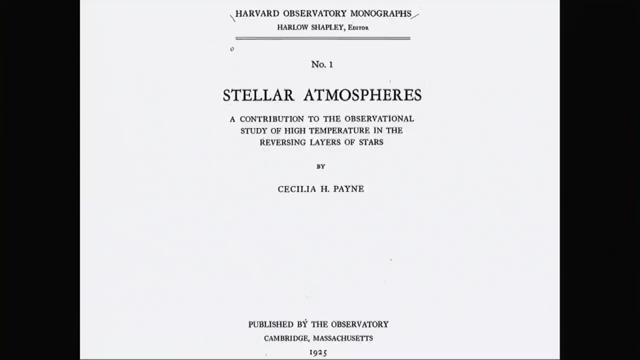 Right, And it is this field that was launched now, I guess 90 years ago, with Cecilia Payne-Kabashkins, or, I guess at the time, Cecilia Payne's work And what I now want to do. 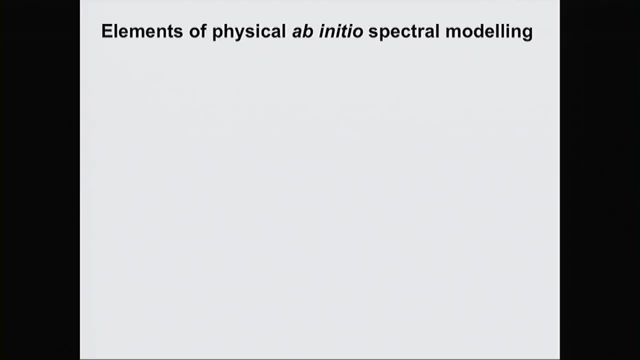 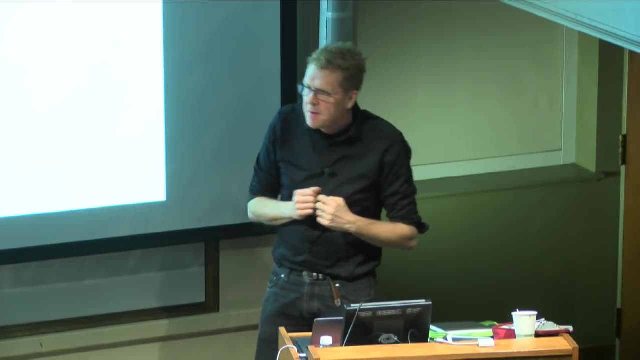 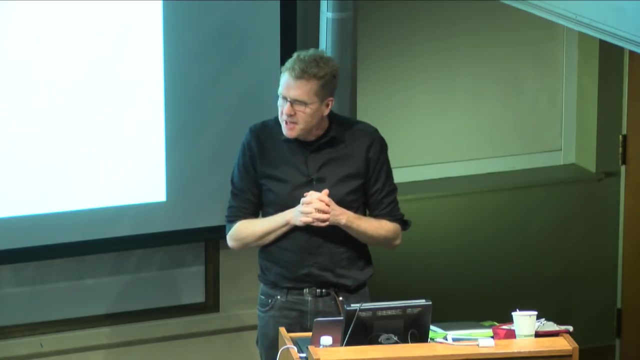 is give you a brief summary. I will spend relatively little time talking about physical models of spectra, but I will show you their beauty and their bane, because that is actually an amazing accomplishment. but data have gotten so ahead that actually the models aren't good enough. 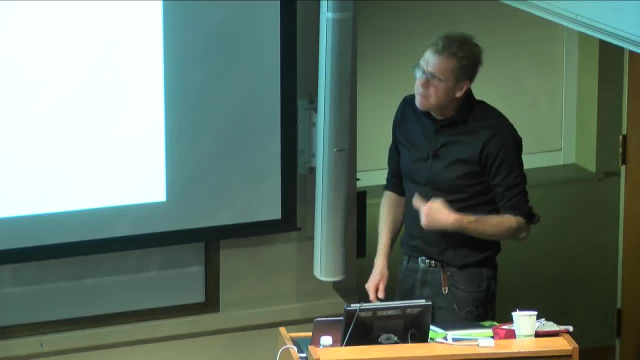 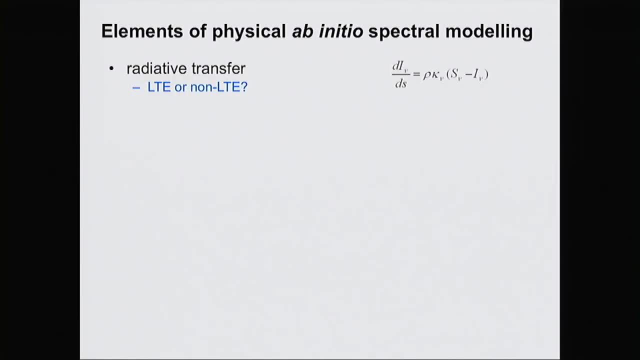 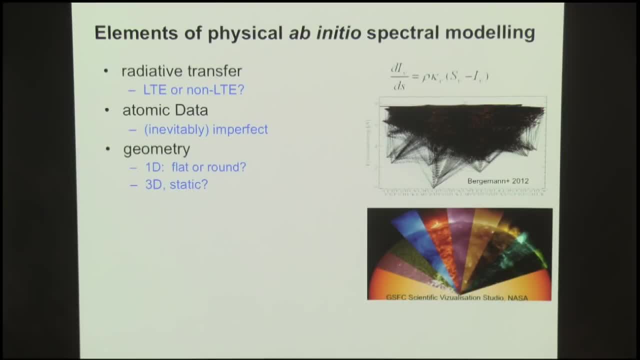 And you have to make a choice of geometry, 1D or 3D, even among 1D, flat or round, static, and of course, you know, at some level stars don't satisfy any of those assumptions exactly. And then the procedure is after you. 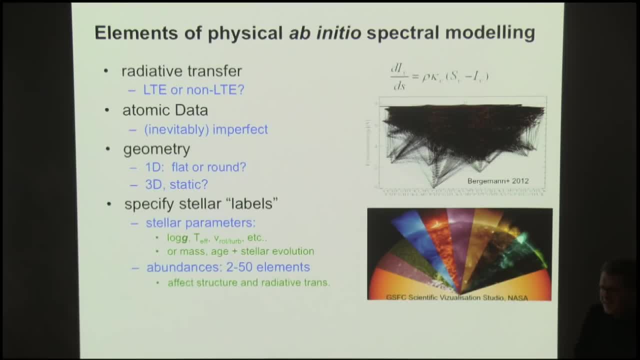 make these choices- and, of course, Bob Cruz has been leading this story. for is you specify your model by a set of parameters, right? Either you take log gt effective, or you take the mass age and cell evolution, and then you have to specify all the abundances. After you've done that, you 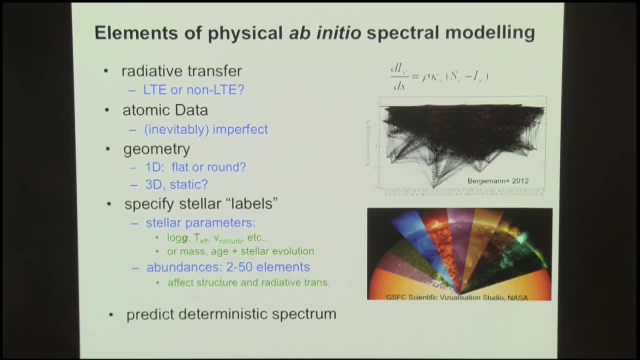 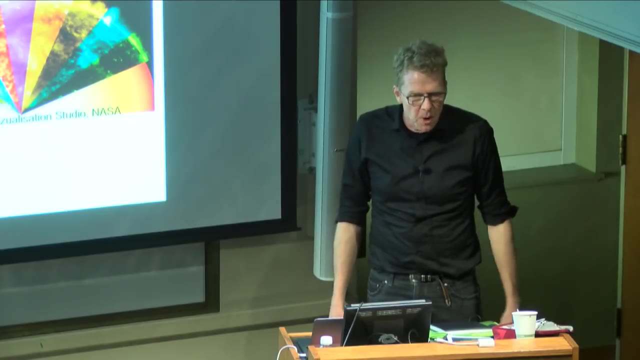 can predict a almost deterministic spectrum, and that, I should say, is actually a beautiful thing about stars and stellar spectra. For most stars, most types, once you specify those numbers, even nature should give you a deterministic spectrum at better than a 1%, if not at a level. Remember. 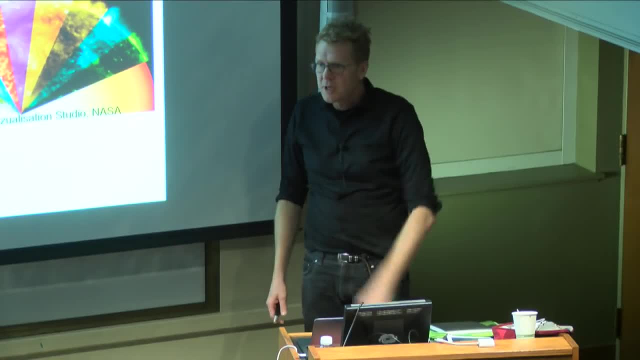 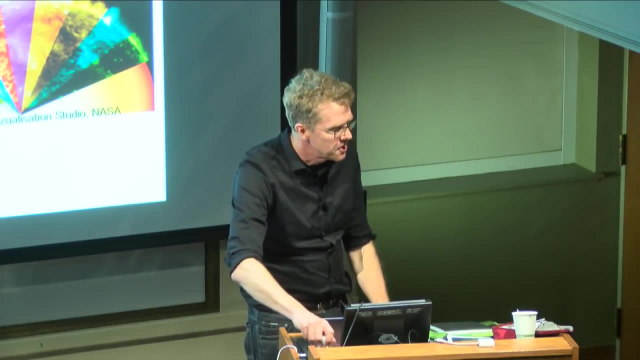 in Galaxy. if you predict the number of stars and stellar spectra, you can predict the number of galaxies. If you're predicting galaxy formation, there's no point in trying to predict the particular geometry of one galaxy, because the Gaussian initial conditions still percolate through. 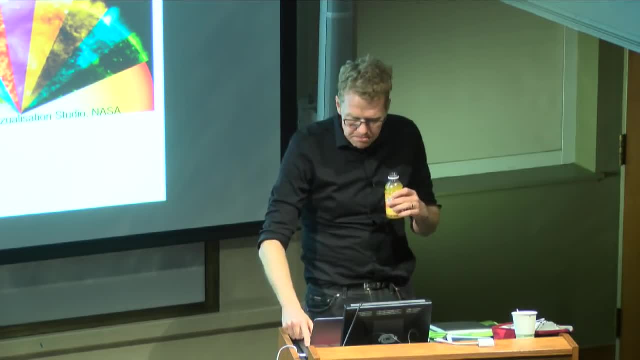 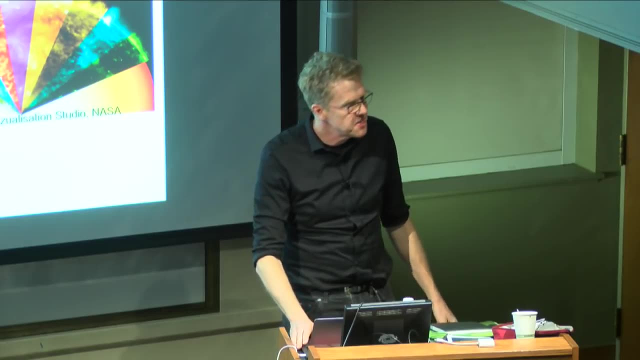 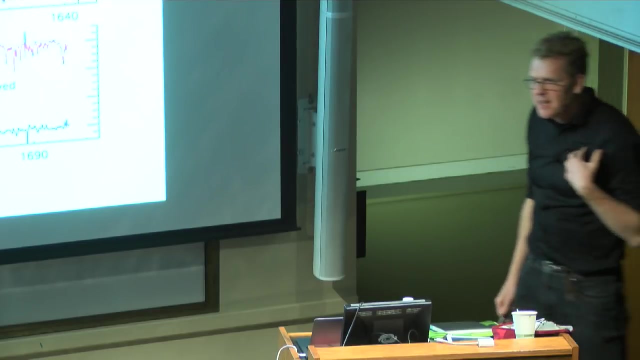 right. So galaxies have a lot more weather than stars, And then you fit the spectrum and learn right. That is the basic procedure intended, And why did I call this the beauty and the bane? And so this is the tricky part. 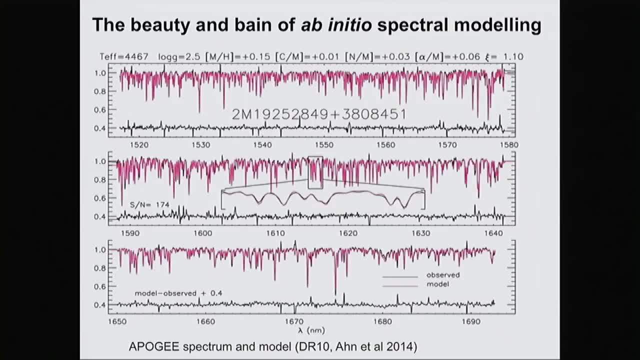 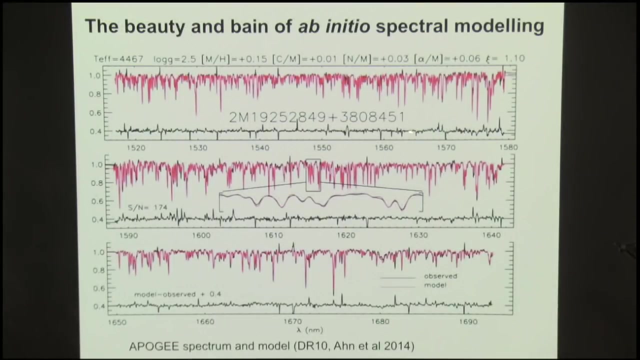 This is because these models are an immense intellectual accomplishment, but still they actually the data are so good that the shortcomings of these models hurt. So here's, just from the Apogee A, a comparison of a DR10 model. and you see, you know it works here, but these 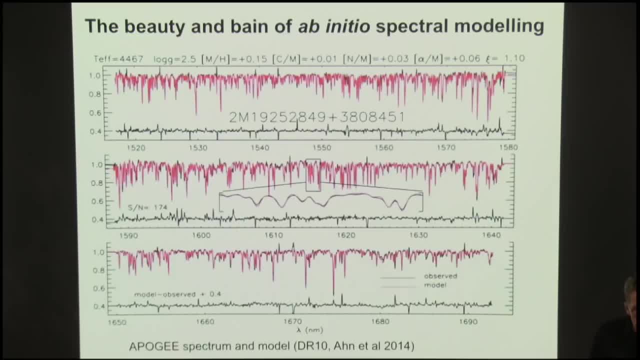 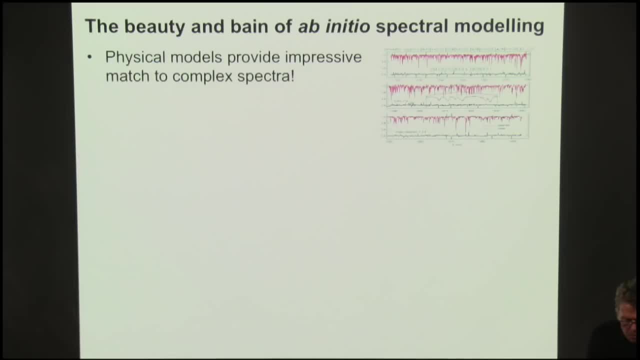 are the deviations, and just in many places, you know, some lines don't fit and they differ by a lot more than the noise, And so this is why one is in this dual situation, that there are significant systematic mismatches that can reflect, in different regimes, any of the previous model. 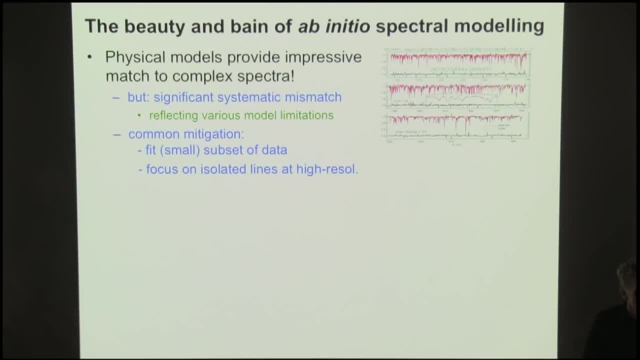 limitations- atomic data perhaps foremost, but also radiative transfer and the approximation of staticness, et cetera, And if you then just blindly fit it, you get answers, but that do not make physical sense in many cases, And so there is a remedy and is focused on the 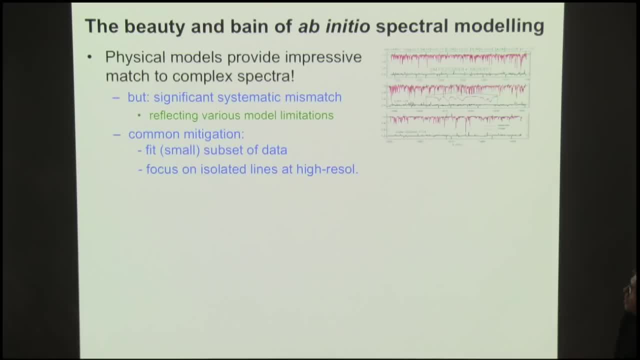 subset of data where the models doesn't have shortcoming And, in particular, often it is best and easiest if you focus on isolated, straightforward lines for diagnosis, right? But let me just show you, I have anonymized. this is for survey spectrum. 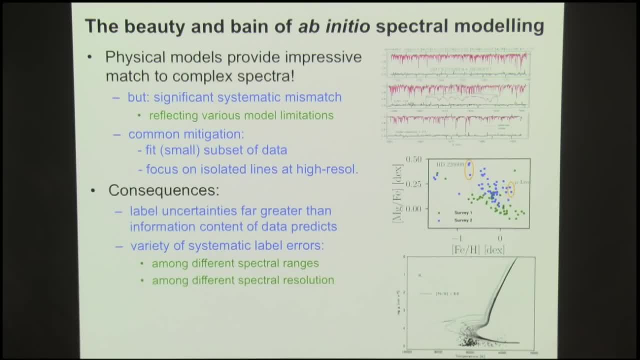 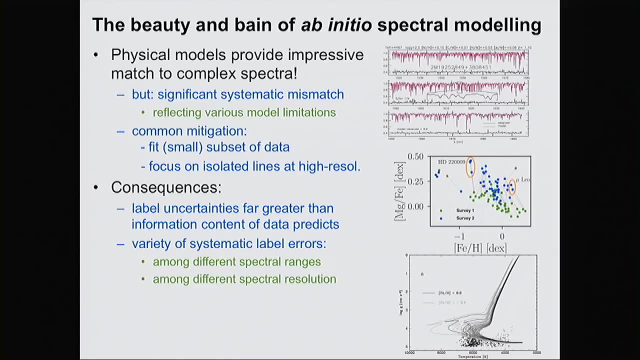 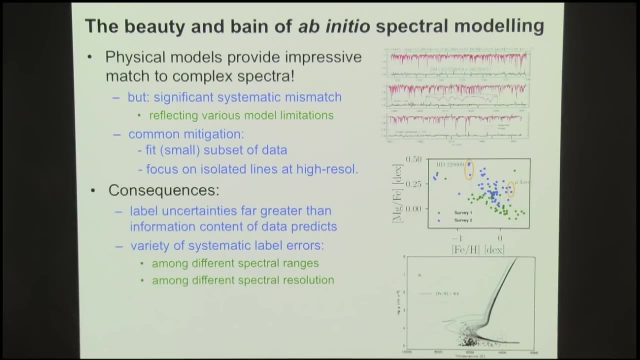 So you have different groups looking at the same stars with different codes- I think by all accounts state-of-the-art- and get differences in the magnesium abundance that are very significant. Or, of course, that procedure gives you no guarantee that the log-GET effect, if you get out, actually allows for a hydrostatic equilibrium solution. 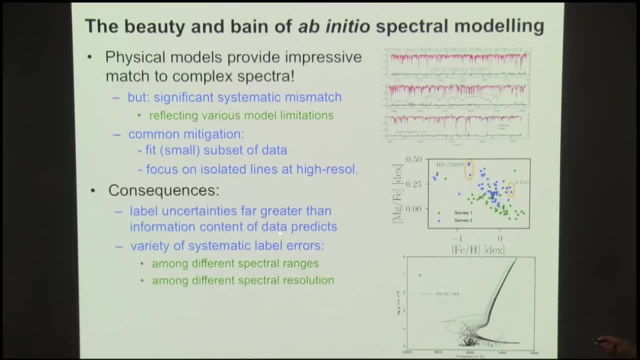 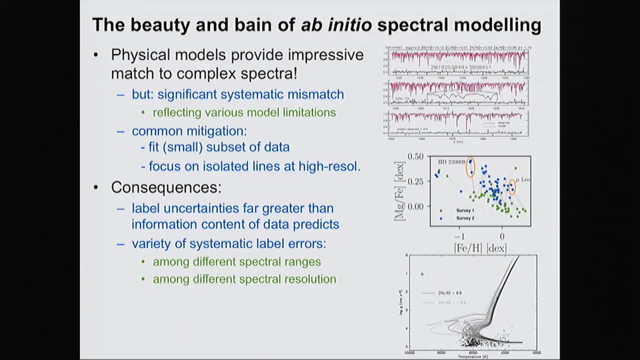 of the star itself, Right, And so you can fit small subsets and get the right answer. That requires enormous amount of signal-to-noise And it's very hard to get things consistent among different spectral ranges and different spectral resolution, Because, after all, the effective temperature of a star is not a function of the wavelength at which you look at it or the resolution. 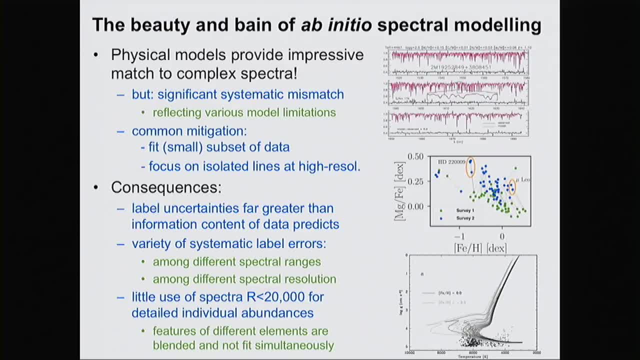 So, and as a corollary, this has meant that if you want to get detail abundances to look at the information of the elements, there has been little use of low-resolution to do this, And the reason is also because they're all spectral features, at least in cool stars, are highly blended. 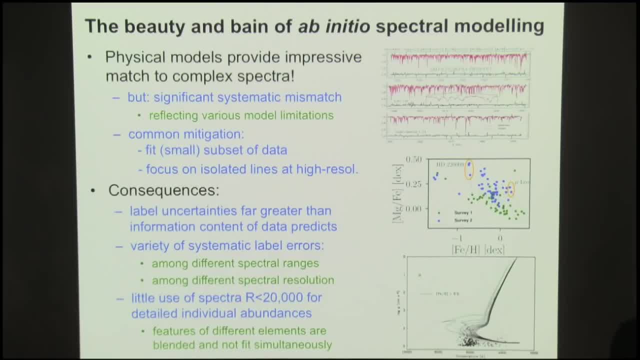 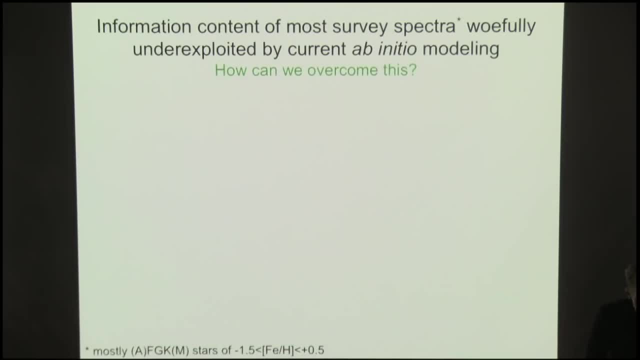 so it's very tricky, if you don't fit them all at once, to do it right. So, despite despite all the model progress, the data have gotten ahead faster, And so this leaves us in the problematic state that, indeed, for this survey spectra of 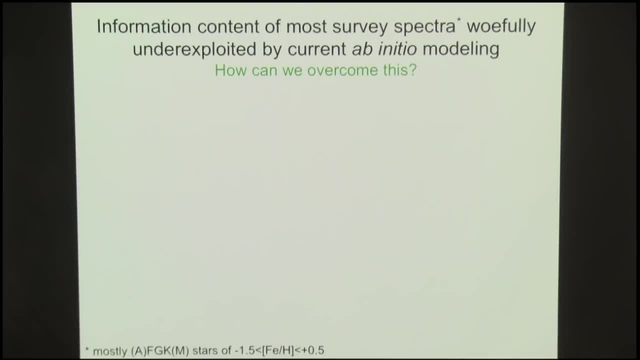 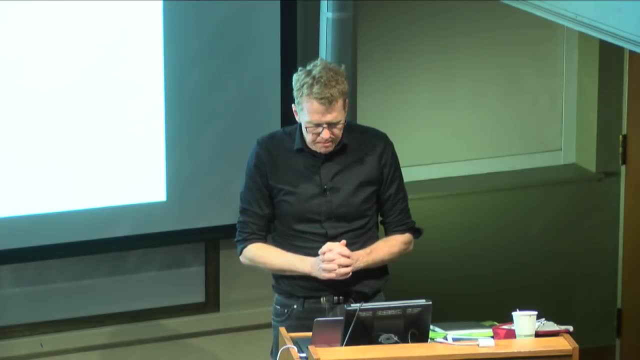 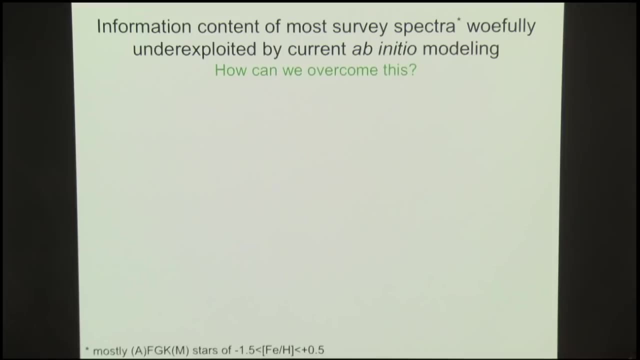 average stars. the information content is actually very much underexploited and there are many systematic issues. So this is at that point there was a few years ago. we started asking that you know it's hard enough to actually get ab initio models right for a few stars and 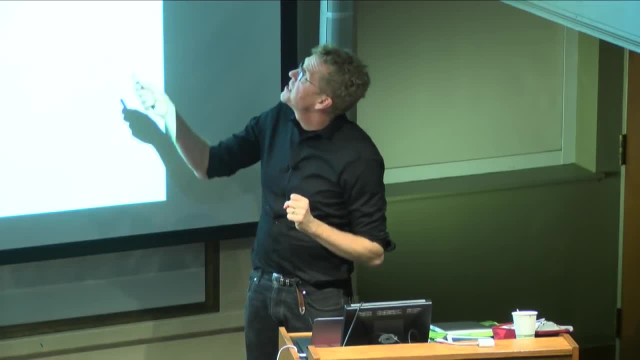 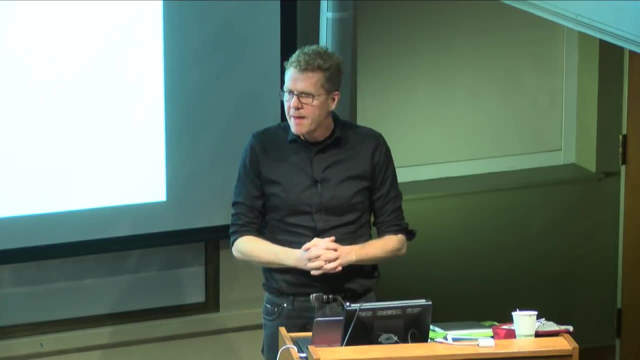 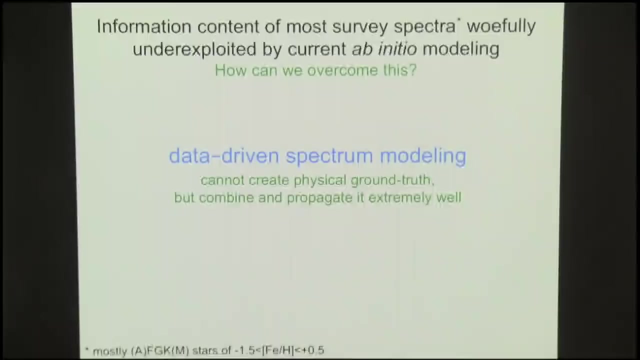 you get it right in certain regimes. it is a tough thing to ask to get them right for millions of stars. What can we do to go from spectral analysis craftsmanship to simple mass production? There are two things that I will tell you about. The one is a different way of looking at things, namely data-driven spectral modeling and 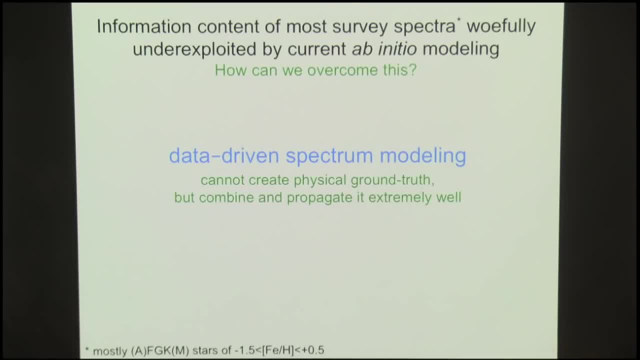 the important disclaimer and benefit is data-driven spectra cannot create physical ground truth, but they're enormously good, as I'll show you, to combine pieces of information to create, to propagate the ground truth to vast samples. I'll tell you more what I mean by this. 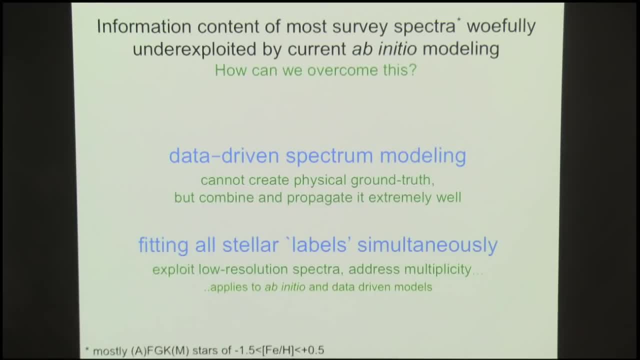 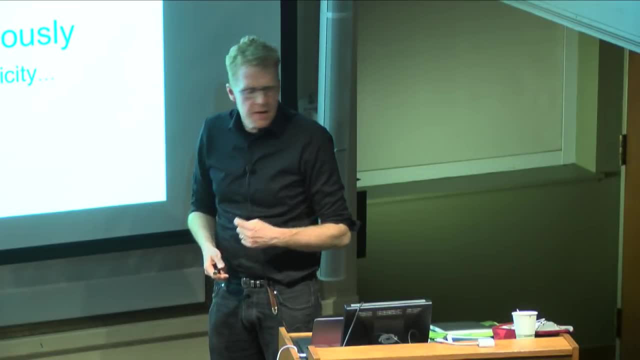 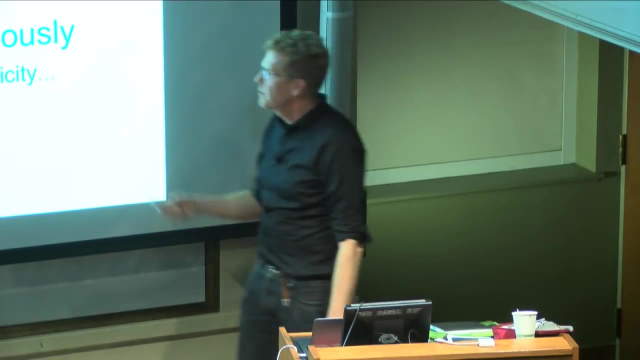 The other part is: imagine you really could fit 20 abundances in all the stellar parameters all at once. then the blending of features would not hurt you. that allows low resolution spectra. and once you can fit 20 parameters, you can fit any unresolved spectral doublet, triplet etc. also at the same time and actually dig in a lot deeper. 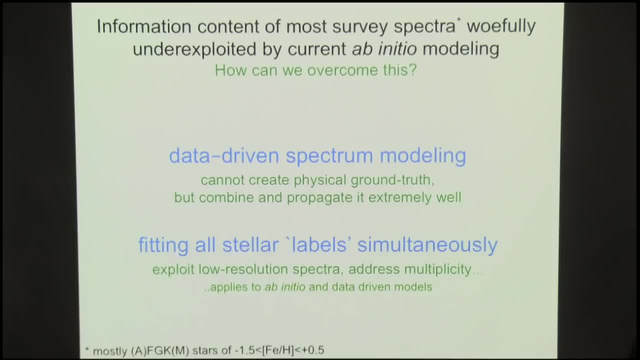 That second part applies both to ab initio models and data-driven ones. So what I will now do with some applications. I will show you, foremost, how pleasingly well this has panned out. I will also tell you about this and along the way, I will show you. 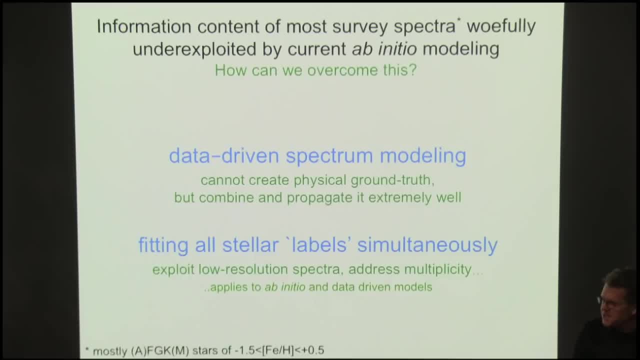 some of the applications At some level. that is perhaps a bit technical, but I think it matters because we have all these millions of spectra that we know there's interesting, fascinating information in it. I've shown you the age part, but I could give you. 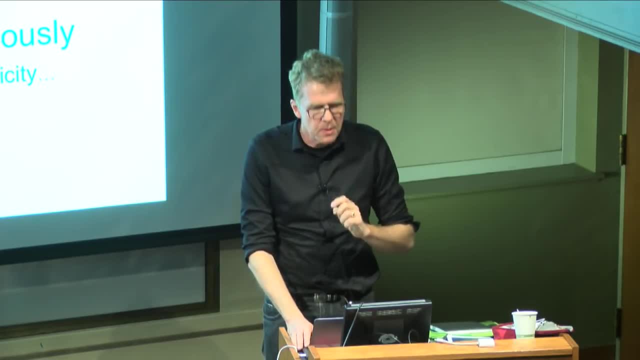 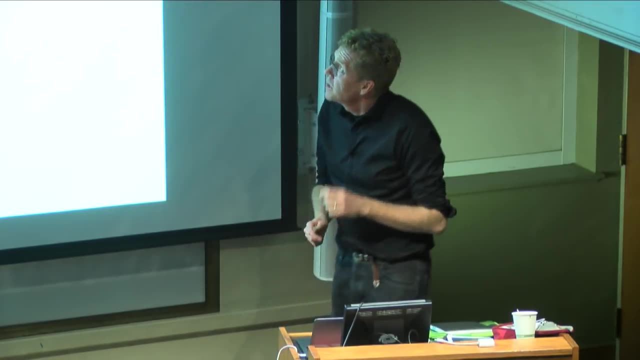 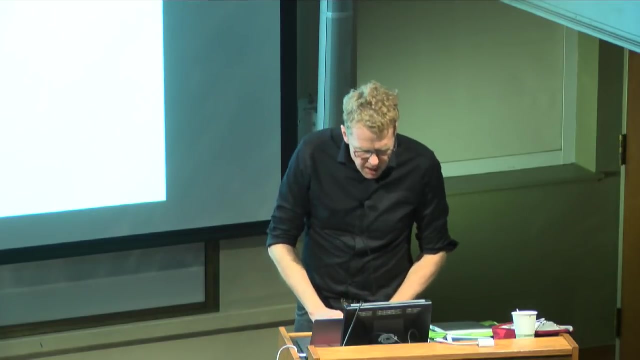 you know, about abundances, about physical parameters, about binaries with compact companions. There are many other stories, but it's good to get all the information out of this. So now this approach, which my collaborators dubbed after another former colleague of yours and 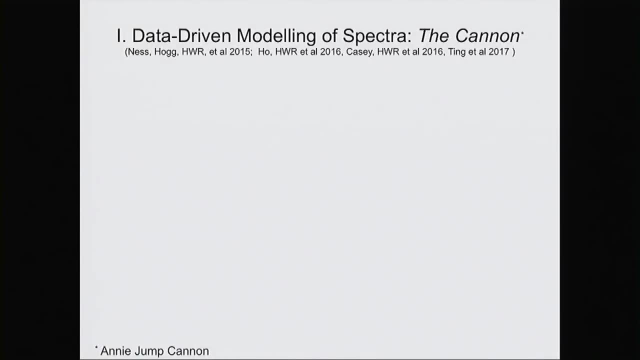 he called himself Andy Andy Jump Cannon, And my friend David Hogg insists that indeed, Andy Jump Cannon was doing data-driven spectral modeling, while Cecilia Pinkovashkin was doing physical spectral modeling. You can talk afterwards how correct that brief assistant is. 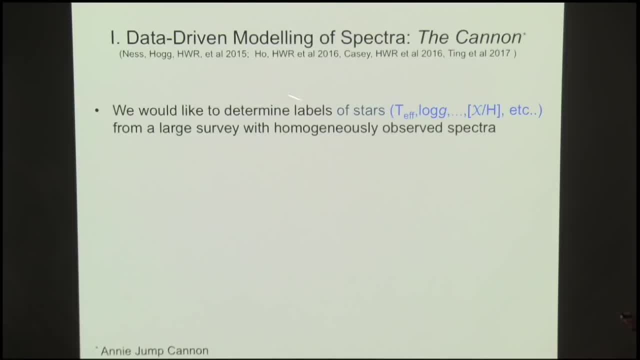 So the task is: we'd like to determine what we call labels, so the stellar parameters in the abundances for spectra, from a very large survey, And it turns out that very simple assumptions help us forward: First of all, stars that have identical stellar parameters. 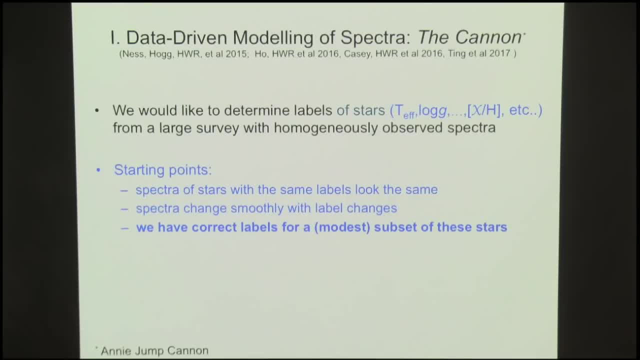 and identical abundances have identical spectra. The second one is: you move any one of these parameters. every pixel in the spectrum will move differentially or smoothly. So that's- And let's presume, for good reasons. we have ground truth for a very small subset of those stars. 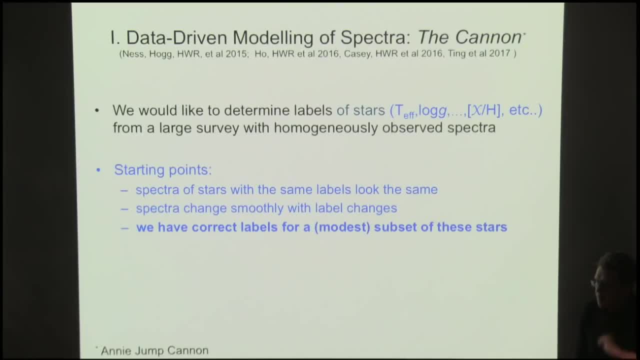 Because we happen to have very high-resolution spectra where we can analyze things, because we have astro-seismic information, any of these things. And now the question is: how can we use that information to get it right for the entire sample? And I'll get back to this point. 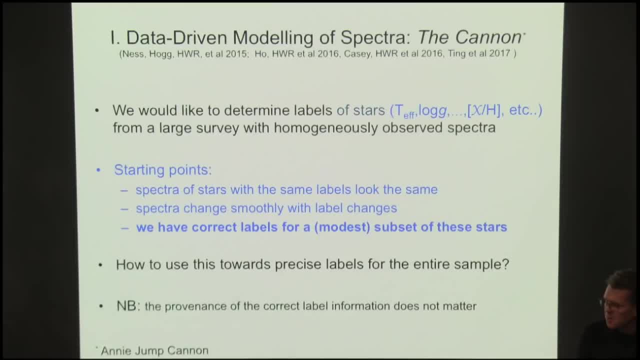 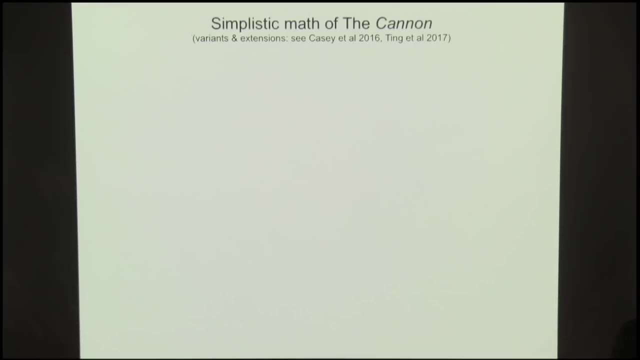 whether other physical models or something else told me, the answer doesn't matter. That is, we have a small subset of spectra where we know what the right answer is in terms of this, And then it is a very simple matter to proceed. Let me just walk you through this. 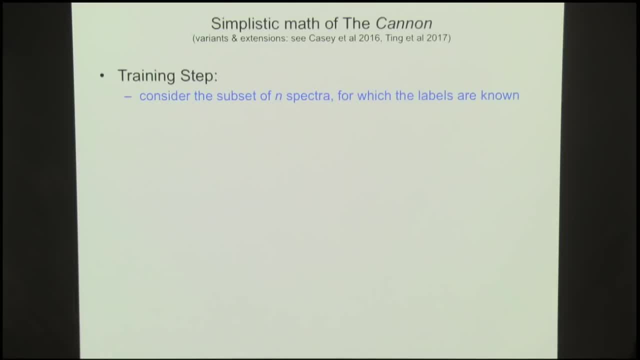 So we take this small subset of spectra where we know the answer, or we accept that we have ground truth. Let's say, at each pixel the normalized flux is some function of these labels I've shown you here, just to keep it simple. 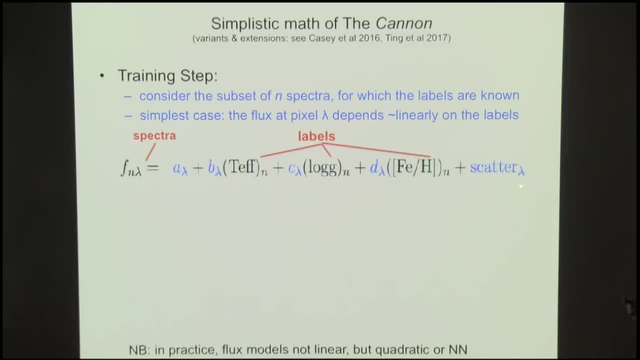 linear. in practice, you can generalize this. So then, if you have, say, 50 stars at each pixel, you solve for these coefficients in the equation. very straightforward thing to do, And what you've done is now: you've created a model that can predict that flux. 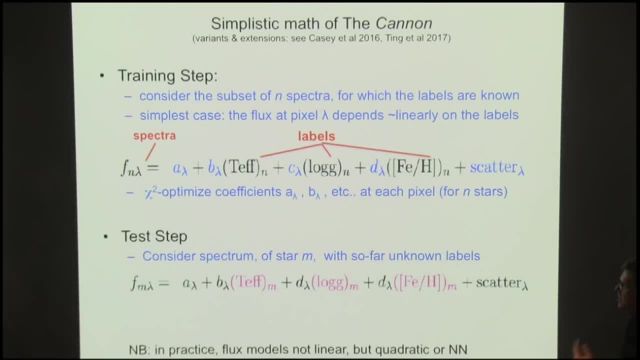 You find those coefficients and then you go to a star where you also have a spectrum with the same setup, but you don't know what the labels are. But hello, you've solved most of the work, namely, those coefficients are still the same. 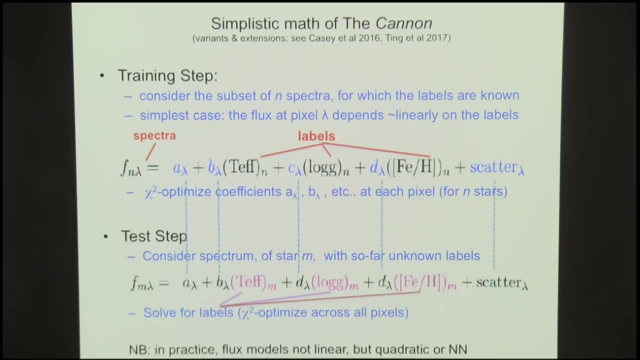 and all you have to do is solve for those coefficients and then you have analyzed this spectrum And think of it. an even more primitive version is: if you have a thousand examples of spectra where you know the answer, you pick a new spectrum, say: 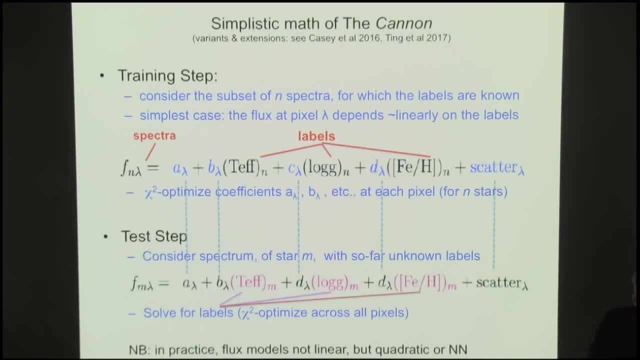 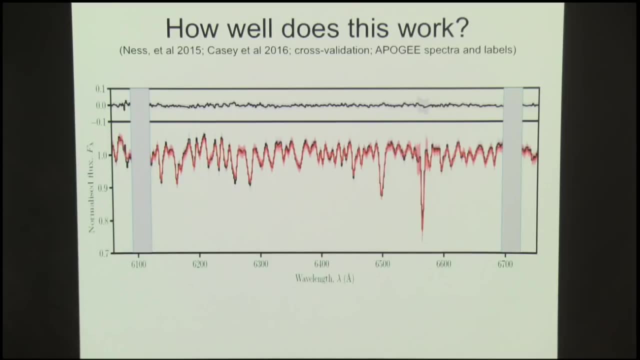 to which of these does it most look similar? and that's about right. But you can generalize this. and let's now see how well this works. Here is a model. again. It works basically beautifully. I have fig-leafed those two parts for later use. 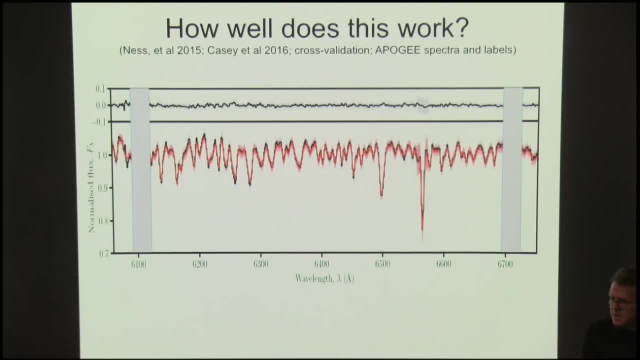 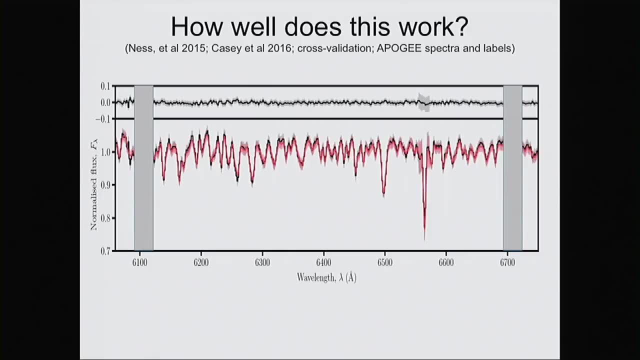 So in spectral space you get a perfect batch. But how well do you actually do in recovering from the new spectra the numbers you care about And that we can check very easily? It's called cross-validation because you actually have held back. 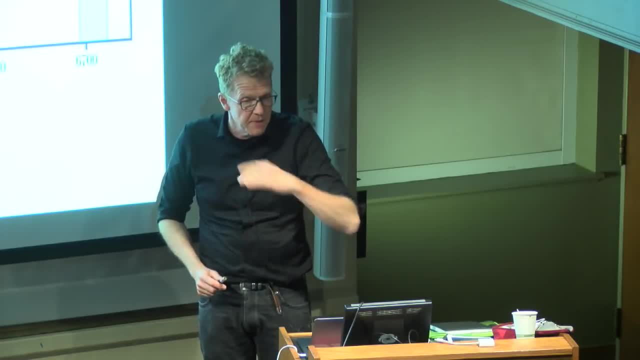 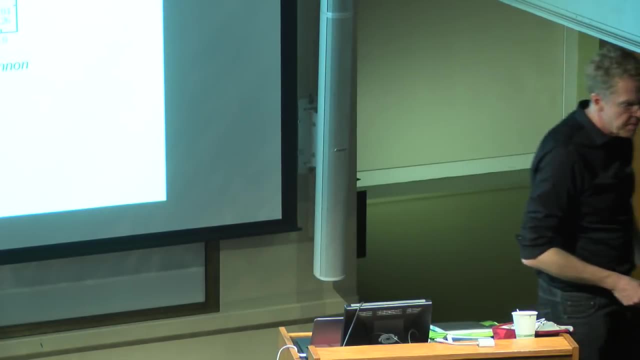 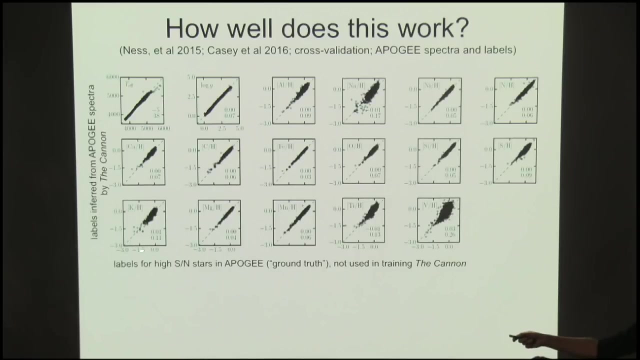 a whole bunch of spectra where you think you also know the answer, say from high-resolution spectroscopy, and you try it out, And the more boring this plot looks the better, Because really here you've taken new stars, you have solved that second equation. 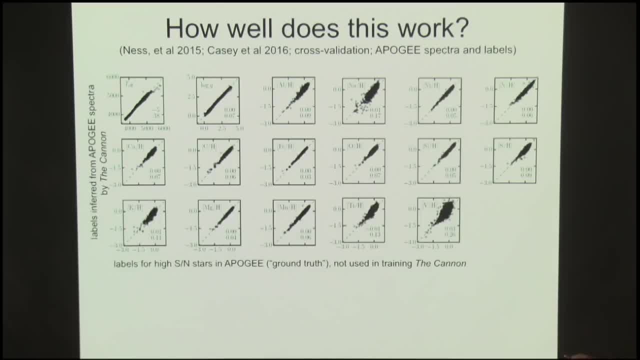 to get a label whether it's effective temperature, aluminum, manganese, and here you have. you looked up the answer which we have gotten elsewhere. That looks good, and you get temperatures: 38 for those, You get iron to 3% precise. 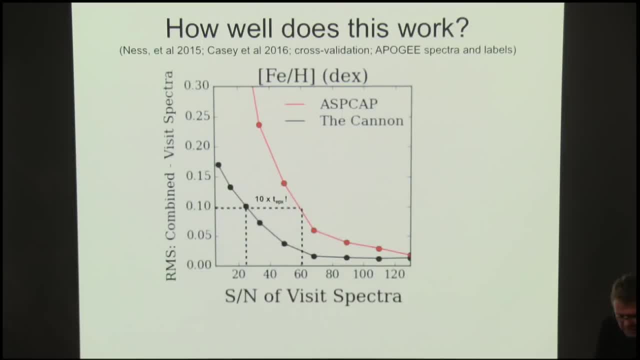 You just reproduce it before, right, You get precision. Let me now walk you through a couple of the practical advantages in successively more interesting. The first one is you now actually use the entire information in the spectrum. So for a given information, 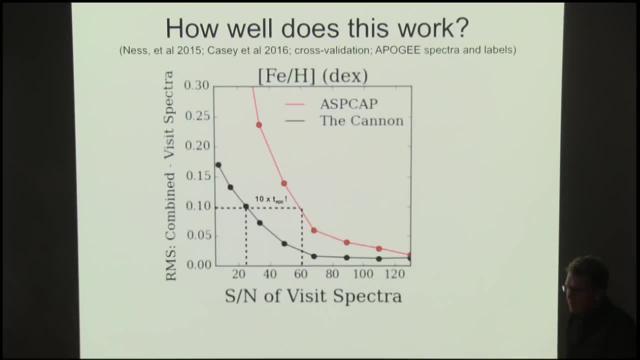 because the lines you don't understand about iron still have information about the iron abundances in them. you just can't model them ab initio. So you get the same precision at a third of the signal's noise, which is a tenth of the exposure time. 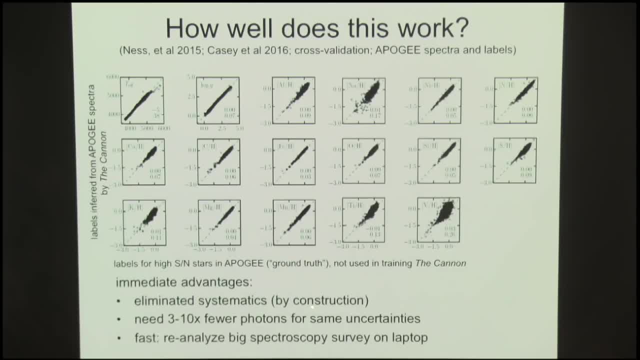 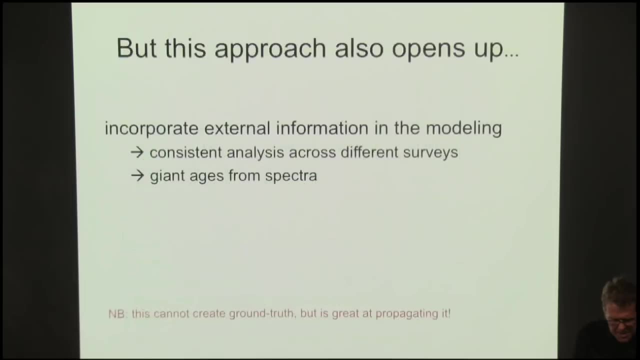 So perhaps at first here a banal thing: by construction you have least eliminated systematics. You can do it fewer. and the other thing is any problem that you've reduced to linear algebra goes fast. You know, that's perhaps undramatic changes. 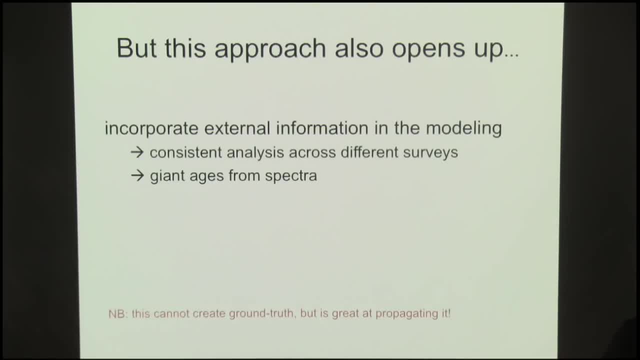 except if you realize how much money has been spent on collecting photons. So let me actually- I'm sorry, let me- walk you through things that, from my perspective, get increasingly more interesting. Namely, you can actually achieve consistency across different surveys. 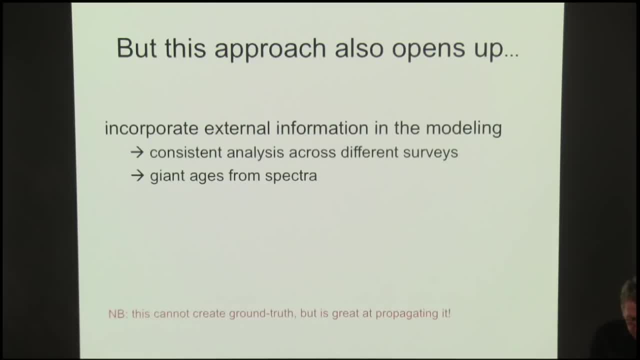 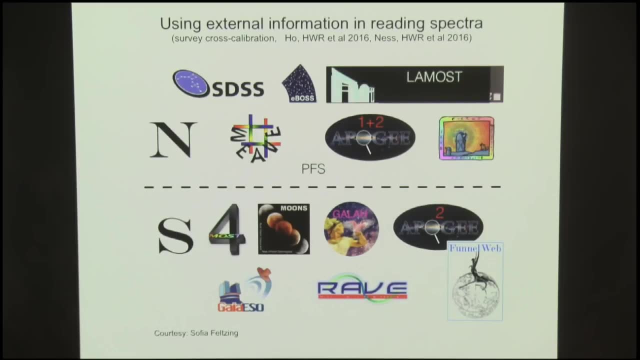 and you get ages, which were central to my initial argument. Why does it matter to get consistency across different surveys? This is the bewildering landscape of northern and southern hemisphere. spectroscopic surveys: Infrared- high resolution. optical high resolution- medium resolution. 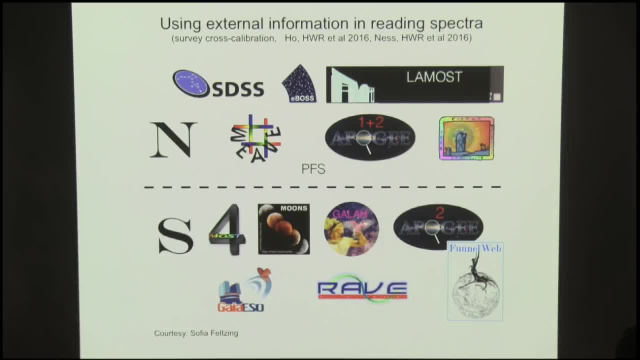 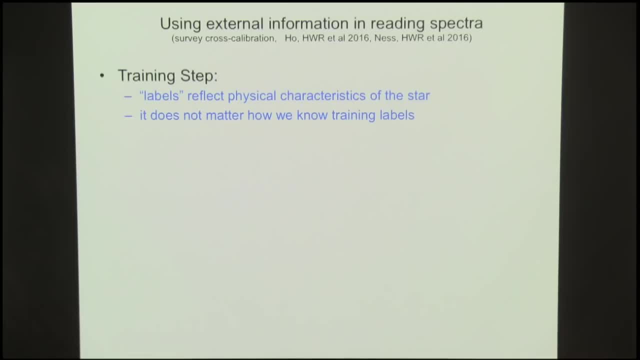 low resolution, different wavelengths. But the good news is, the labels reflect physical characteristics, not actually any property of the spectrum. So let's go to the last one. LAMAS survey, Lousy resolution: 1800 spectra in the optical. 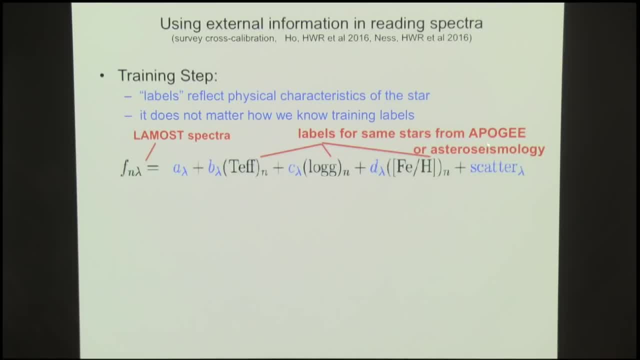 We have a LAMAS star where, from the resolution, 22,000 apogee spectra. we think we have good estimates of the numbers, But then again, where that information came from, where we solve for these coefficients using a few hundred examples. 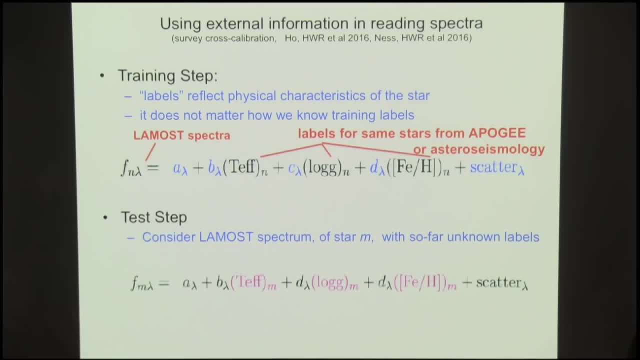 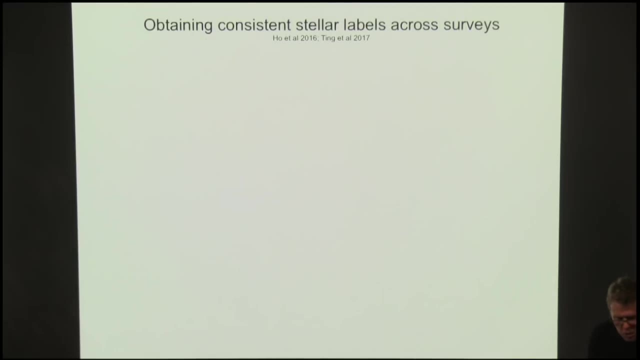 And then you go to a new LAMAS spectrum. you know those, you solve for those and boom by construction you actually have LAMAS spectra on the apogee scale. Let me just show you how well this works. 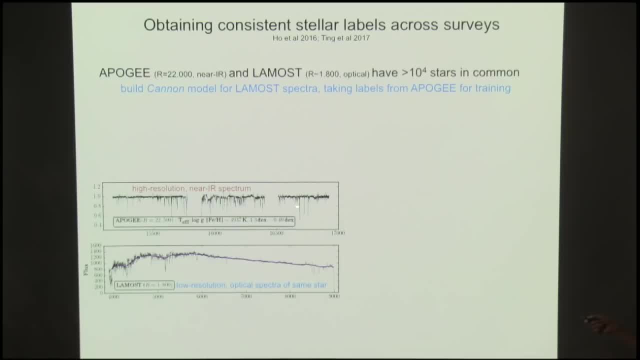 So you have a high resolution in the infrared spectrum where you derive your numbers. then you have, for the same object, a low resolution LAMAS spectrum, but you basically have a few thousand examples of low resolution spectra where you know, for whatever reason, 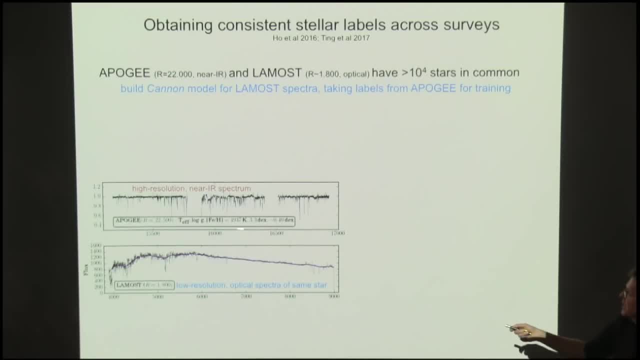 this is what a LAMAS spectrum looks like. if these are the numbers, And the plot looks pleasingly boring because you can then for new objects out of the LAMAS spectra. temperatures to 50 Kelvin, log g to 0.1,. 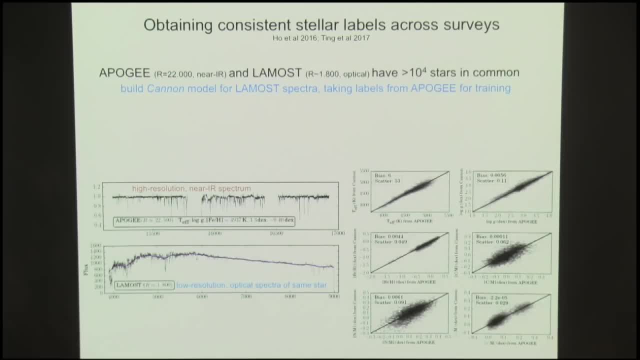 and you know, and alpha enhancement with a scatter of only 3%. So this is just the precision with which you can tie the two surveys together. Okay, This is actually. it is remarkable to what length sometimes different surveys go not to observe the same objects. 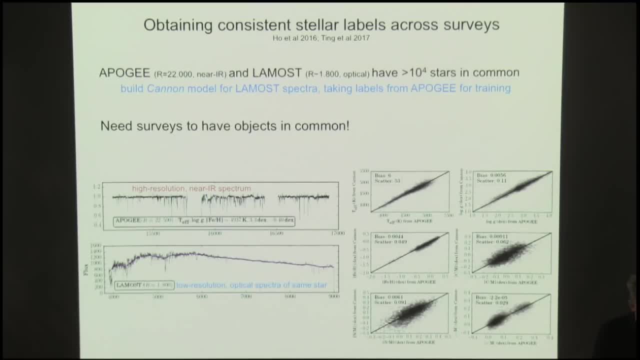 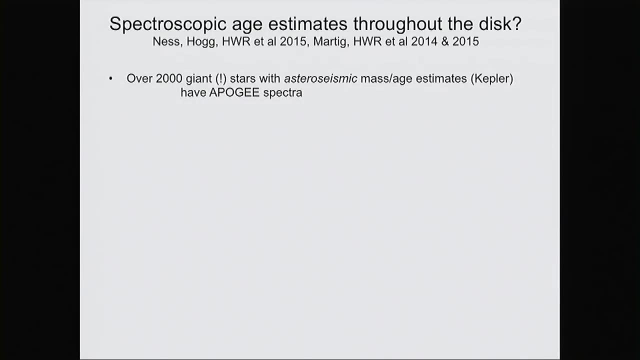 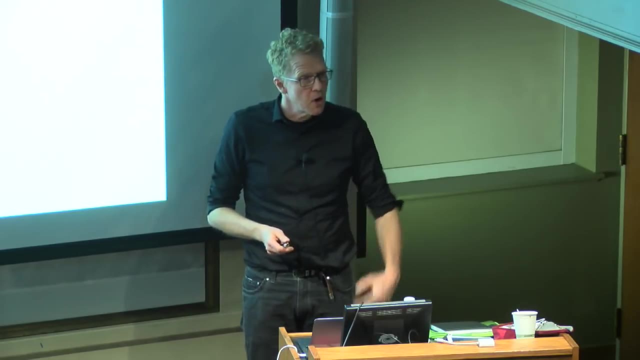 which is a no. no it's. I know it's funny, but it's actually not funny if you have to deal with it. So now let me get to the spectroscopic ages, So the best place to determine the age of a star. 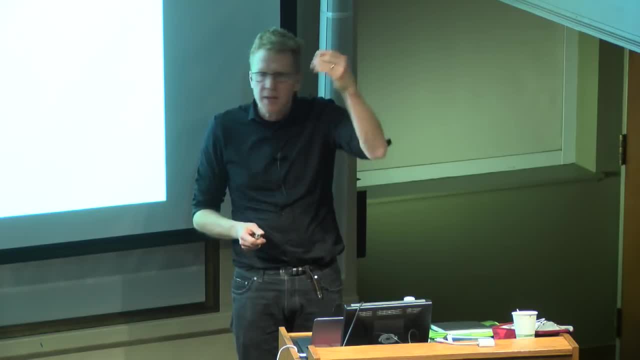 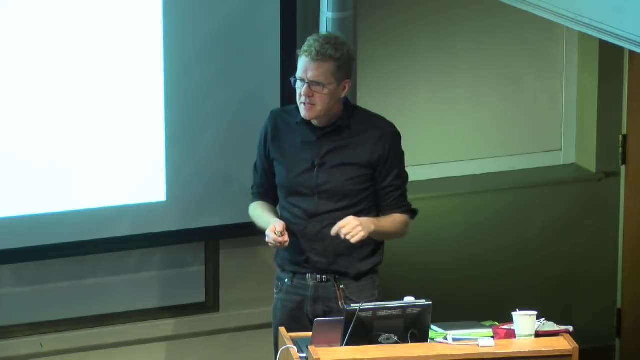 is on the subgiant branch. When you turn off, you just place it on an isochrone and then you know its age. The problem there is that, of course, a 10 times older star on the subgiant branch. 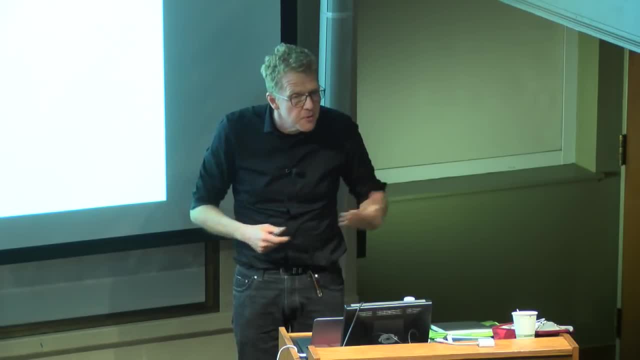 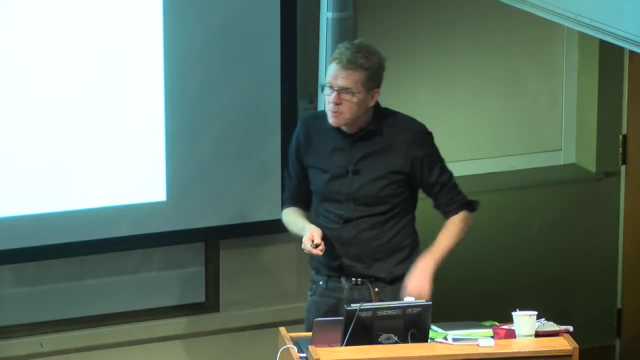 is 10 times fainter, So in a flux-limited survey you only have one thousandth of the survey volume. Giants are great because they're equally bright irrespective of their age. So would it be great to get ages for giants. 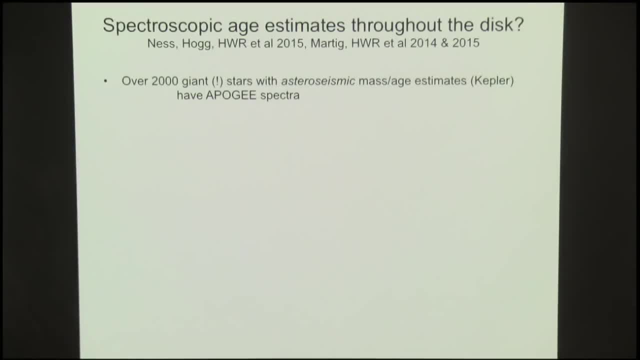 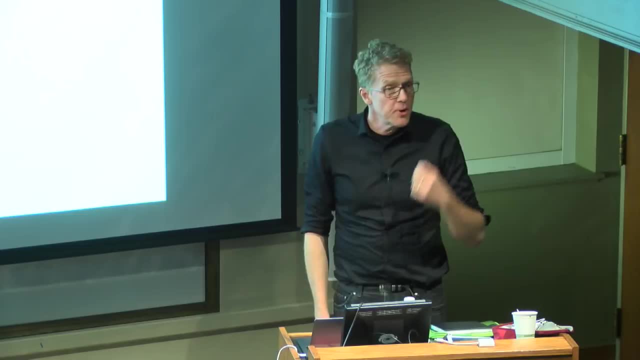 Now the Apogee survey looked at 2,000 giants with astroseismic data from Kepler. Now, just to remind you, for a giant star, measuring its mass is approximately measuring its age. If you know, a giant has two solar masses. 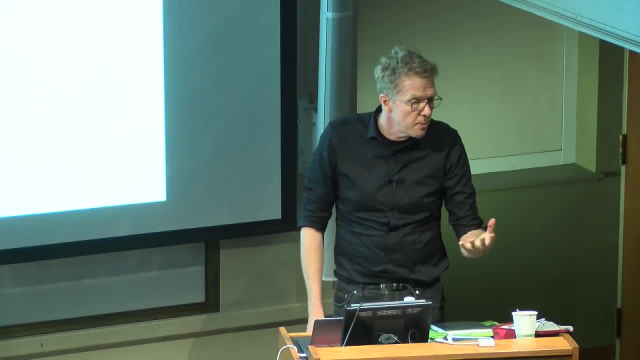 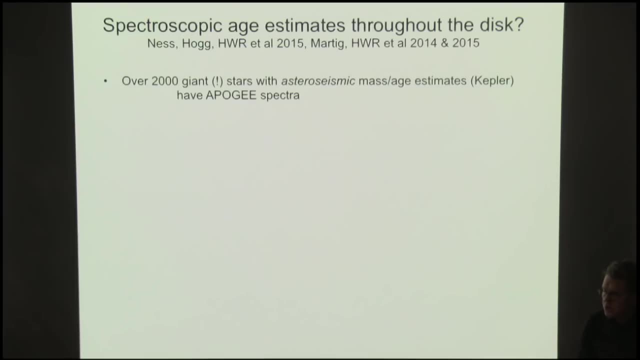 you know it's a little bit older than the main sequence lifetime of a two-solar mass star. So you get astroseismic masses with which some faith in stellar evolution turn into an age, And so then you make that a training label. 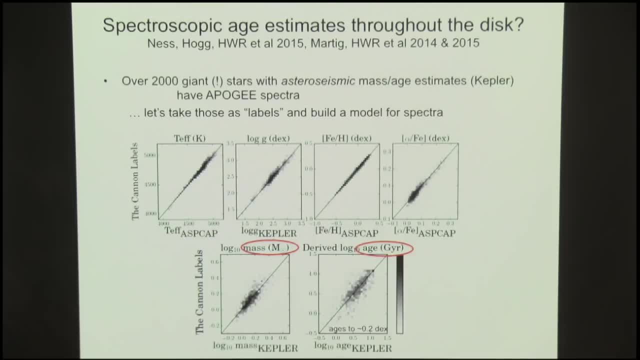 And you just add a term of age and you apply this to Apogee spectra. Then you go to new Apogee spectra. it said: estimate the age for me. You look up its astroseismic age and it works pretty well to 0.2 dex. 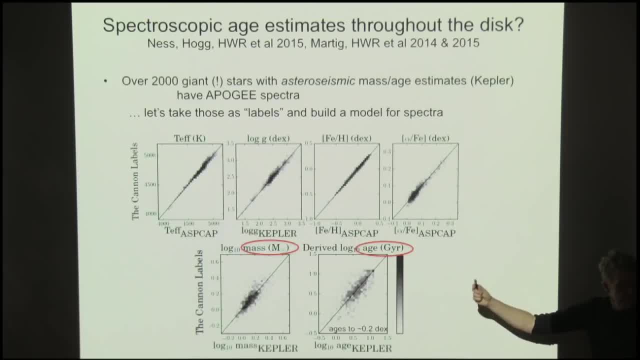 I think, to compare it to the total range between the dynamical time and age of the universe is 2 dex, so actually 0.2 dex is good. This is where your discomfort level that now we have finally reached the stage where data-driven models are just all this voodoo. 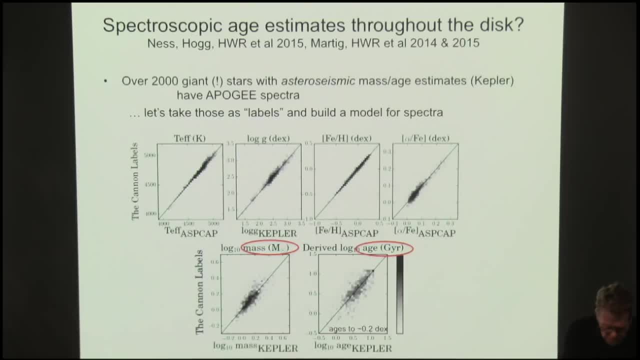 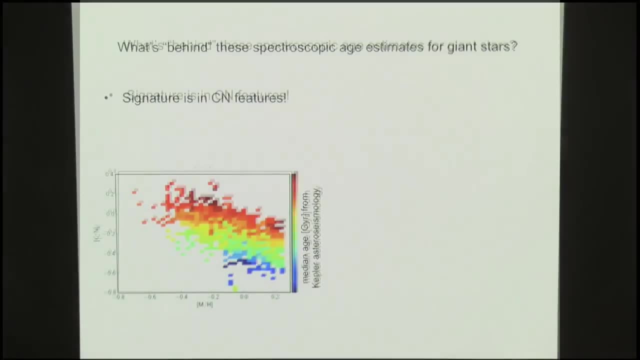 that works, but nobody knows why, And there should be at least two points when this happens. Now, the good news is, you can actually figure out why this works and how it works, and you can show it. So the first thing to say is: 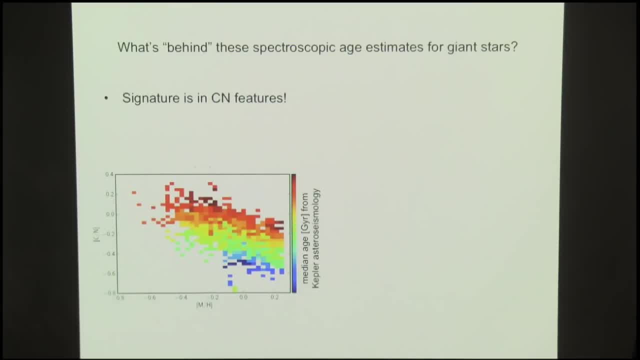 that the signature of age in a giant is in carbon and nitrogen. So one way of looking at this is you plot metallicity in carbon over nitrogen for all the giants where you have astroseismic masses And you see, or astroseismic ages. 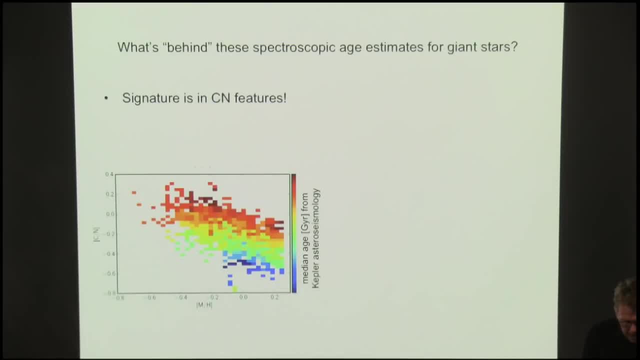 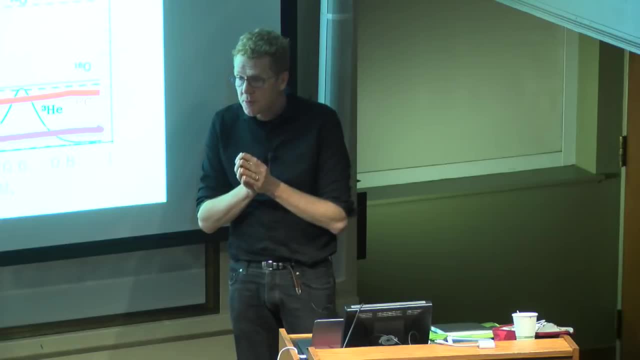 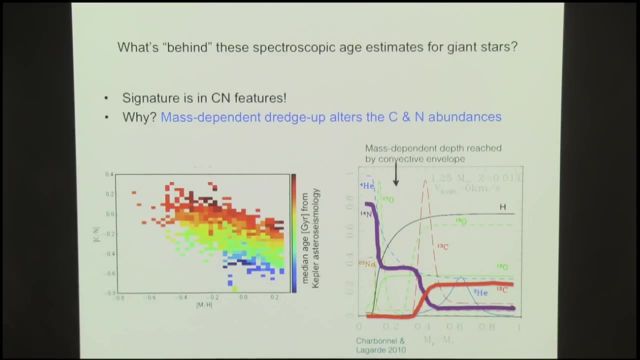 that beautifully correlates And there's a relatively straightforward explanation, at least qualitative explanation that would be hard to make quantitative- Namely, the carbon and nitrogen photospheric abundances in giants are altered by convection. If this is radius of the star, its composition. once a convective envelope gets down deep enough to dredge up material altered by nuclear fusion at the center, the surface abundances get altered And the depth of this convection of course depends on the mass of the star. 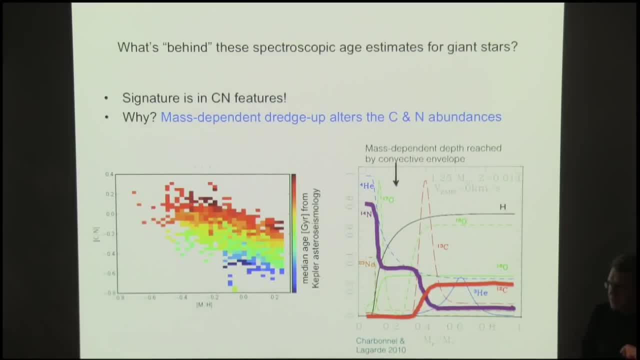 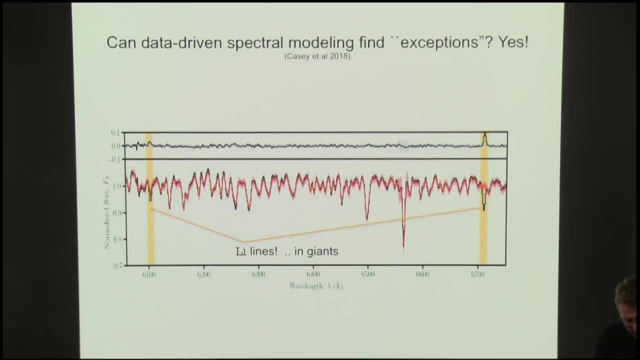 Now, I wouldn't dare, and it's my understanding. it's hard to predict this ab initio, but you have a qualitative explanation and you get to calibrate it against the astroseismic mass. Okay, now let me come to a second part. 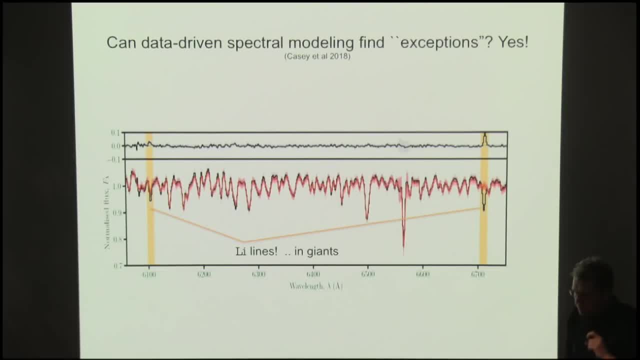 of data-driven stuff. You can only find what you trained it on. That is another common thing to be said. Let me just give you a little blurb here from a paper by Andy Casey. It's about to come out. So you built a model. 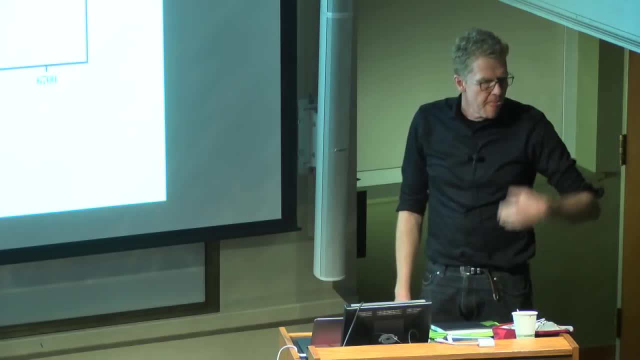 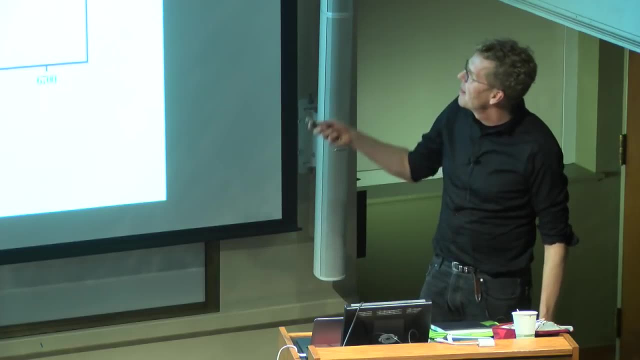 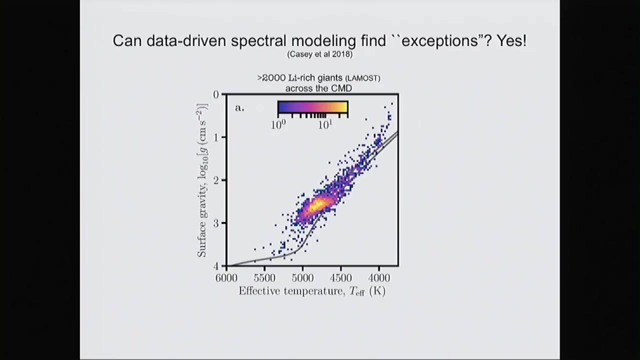 in this case on LaMosse spectra, that is supposed to fit anywhere except for the lithium lines. And then you find objects that have excess lithium And in the LaMosse survey, in one fell swoop Andy found over 2,000 lithium cancer giants. 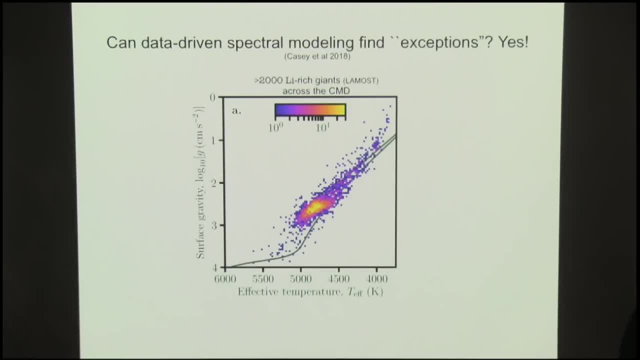 Now, lithium does not live long in the photosphere of a giant star, And one of the interesting things that there could be is that lithium is a giant star. One of the interesting things there could be is if, indeed, a star had swallowed a Jupiter while expanding. 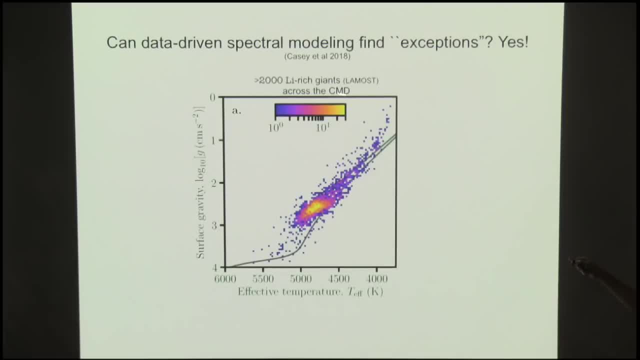 But there are other explanations. What's interesting is here: now you can see, actually you know how fast up and down things go, and you see where the lithium-enriched stars live, So you can kind of actually know during which phase it must happen. 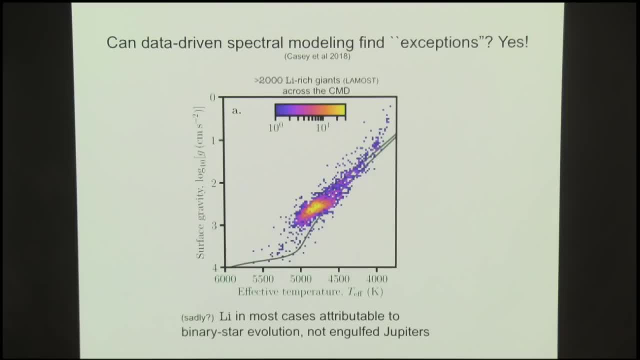 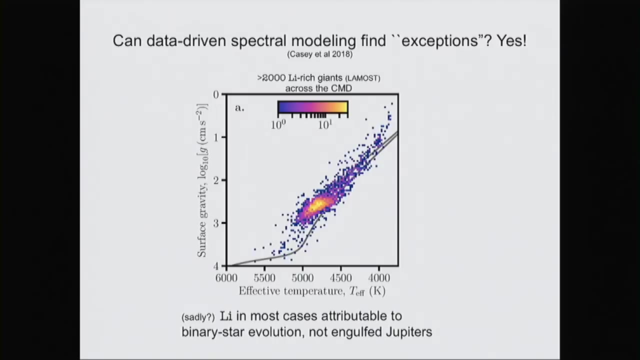 And the perhaps sad answer is that at least models were. the lithium abundance is a consequence of binary star evolution, It tells me. it seemed to work better than perhaps the more sexy explanation, But I think I'm just showing you that if you have these large samples, 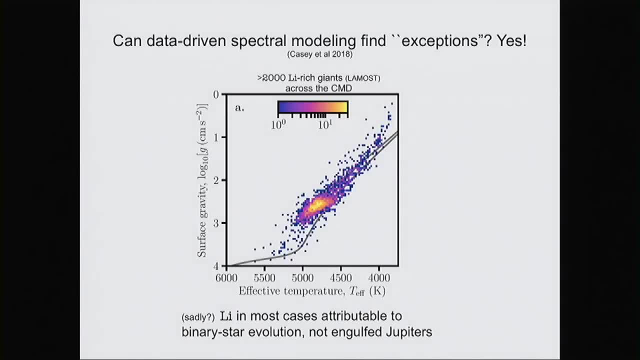 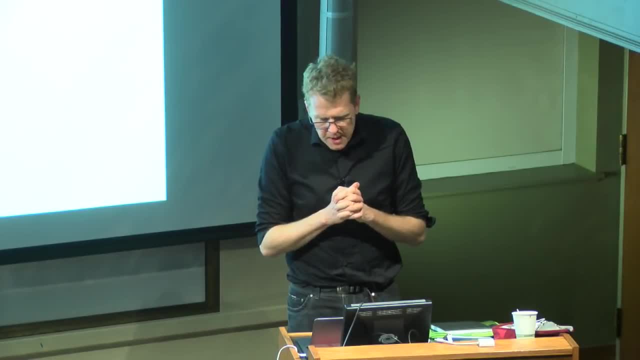 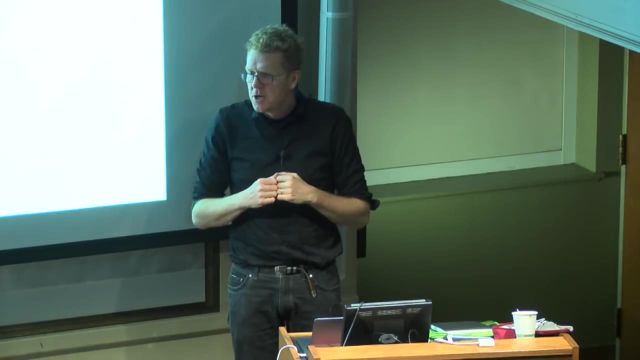 you can do different types of reasonings about this than you could in any one case. Okay, so this was the data-driven part. What it's done for us is you can get all these large samples tied to the scales, where, either from astroseismology, 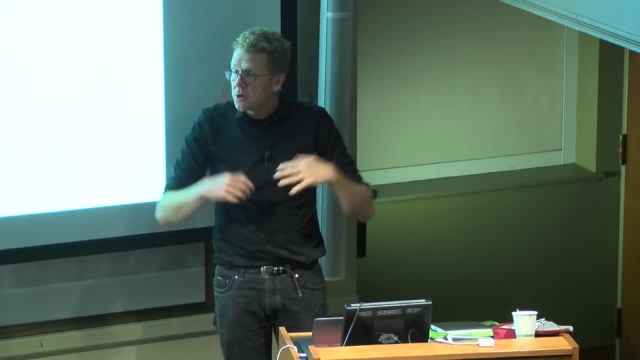 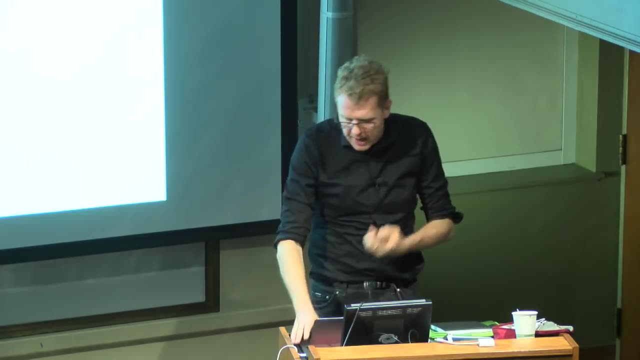 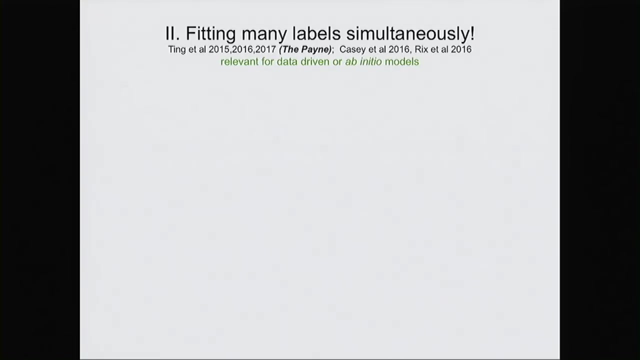 from clusters, from Gaia, gold standard stars. you know the truth. You can bring all of this in and you get these very large samples which you can use for stellar astrophysics or for galactic evolution. Let me bring up the other point. 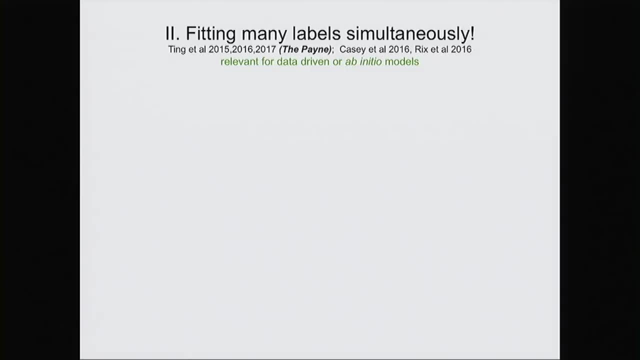 that Janssen has worked on. He may have talked about it. Why is one afraid of fitting everything in a star at once? Imagine you wanted to fit stellar parameters and 20 abundances all at once. Well, how large a grid of stars. 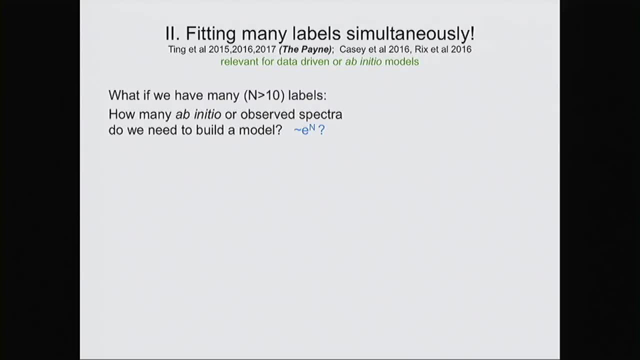 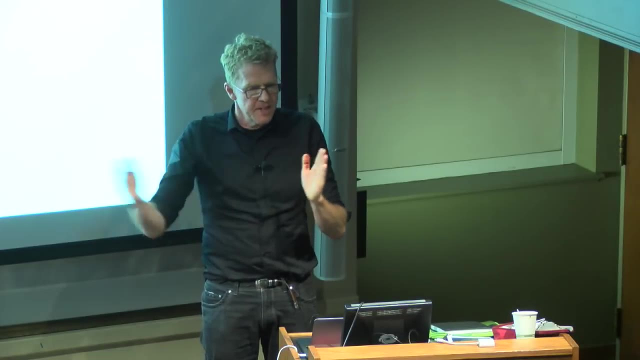 would you have to calculate if you want to have initial models, Or how many training stars would you need if you wanted to have a data-driven model, And in general the answer would be that grows exponentially. Five models in T-effective, five in log-g. 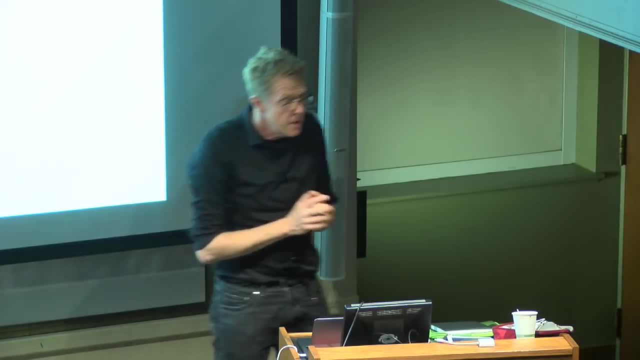 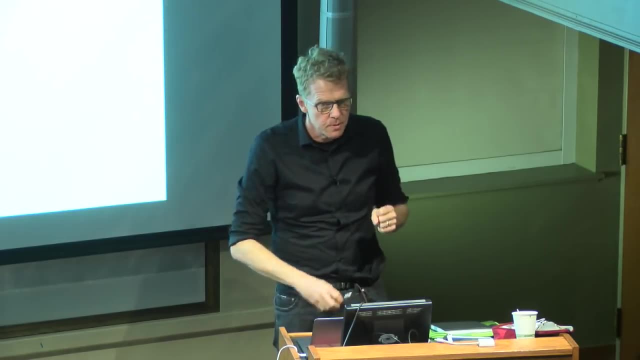 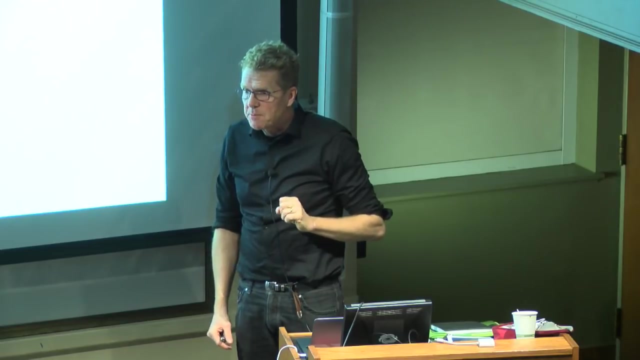 five in metallicity, five in carbon, etc. It just runs away. And if you know nothing else about how spectra change with the labels, that's what you would have to do. But if they vary smoothly, let's imagine each flux varies only like a quadratic polynomial. 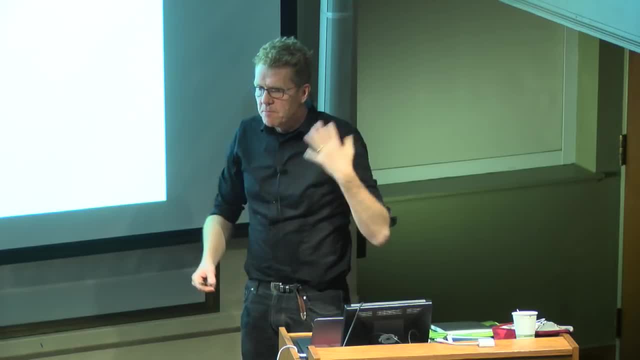 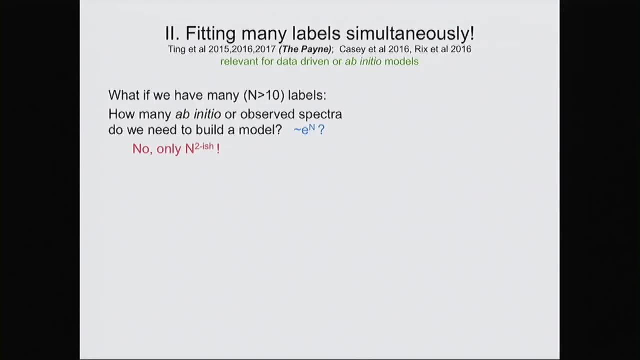 then you need only as many models as you need to pin down the coefficients of a quadratic polynomial, and that's only n-squarish And that actually means with modest number of model calculations you can fit all of these things at once. 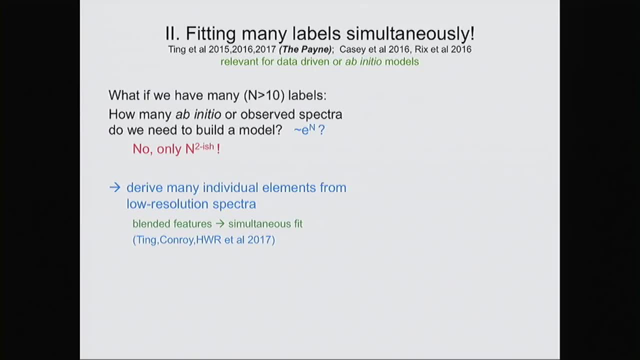 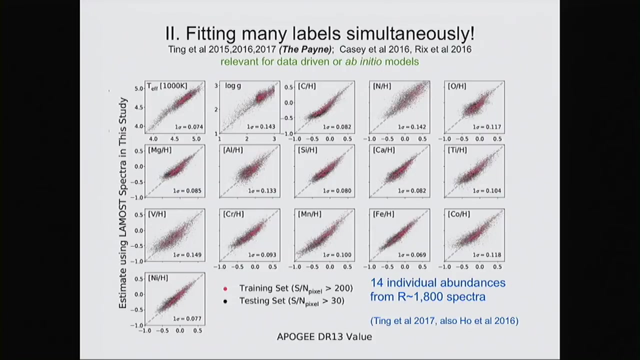 And I will now show you two examples. The first thing that it opens up, in my view, is getting many individual element abundances from plain low-resolution spectra with all the horribly blended features, And the second thing is unraveling multiple stellar systems. So this is yet another. 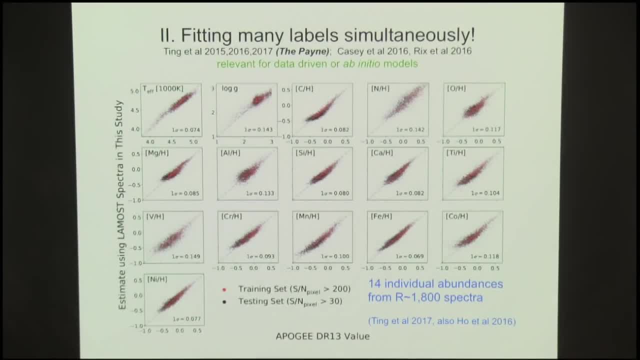 abundances from high resolution versus by building a model from the most low-resolution spectra, fitting everything at once, 14 individual abundances, and it seems to work beautifully well. This is now where, the second time or the third time, you should say: oh, that data-driven voodoo. 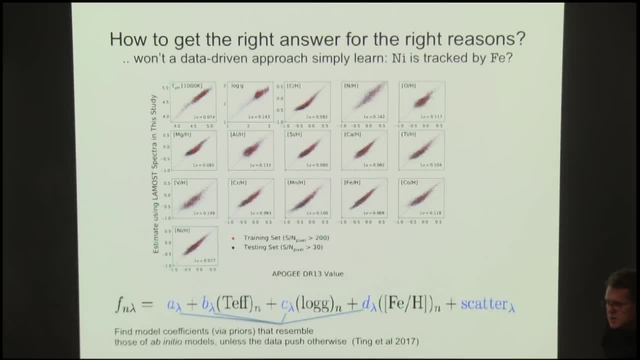 worries me, Because what should worry you is: perhaps nickel just gets tracked by iron. That's astrophysically right. The yields are such that those two things are coupled. Perhaps a data-driven model. all it learns is: hey, let me look up the iron lines. 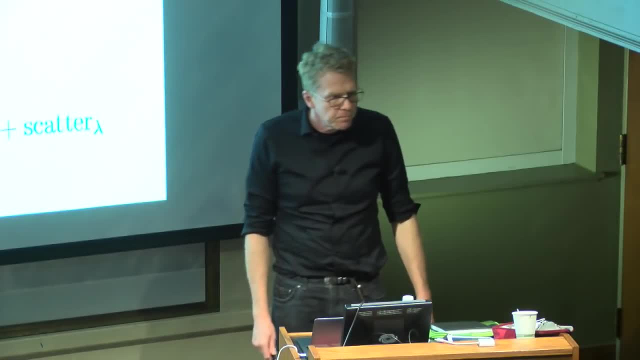 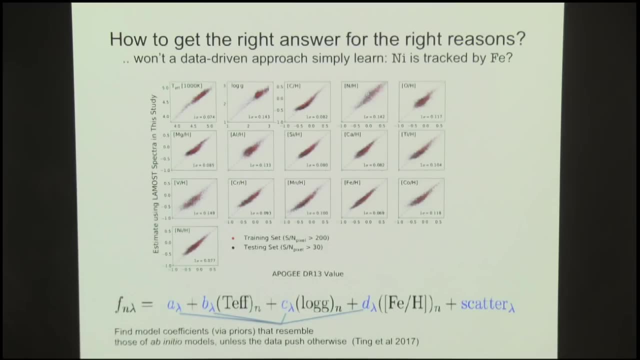 and then, on that basis, predict nickel, and you have learned nothing, And that is of course a worry. But you can actually make a slight modification of this approach. Solve this say: I would like to build a model whose coefficients look like the physical ab initio models. 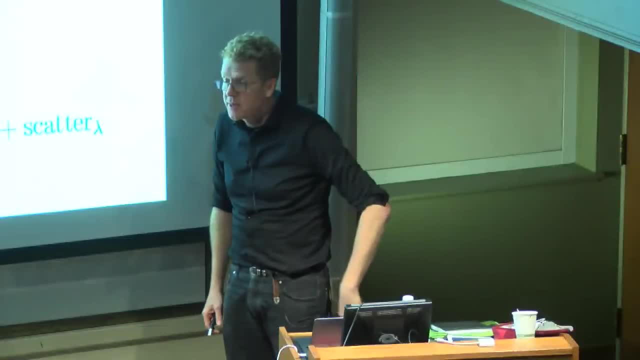 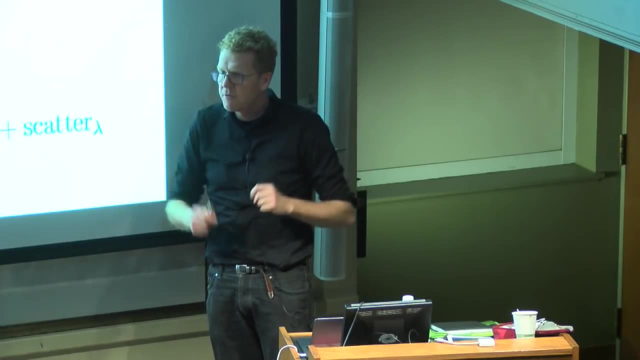 because we actually have some faith in them, say everywhere within 20%, except where the data tell us they can all be true. So there is not a true dichotomy between data-driven and physical models, And then you can actually show that manganese abundances. 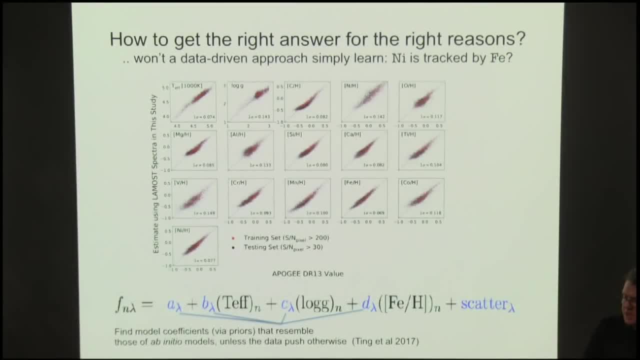 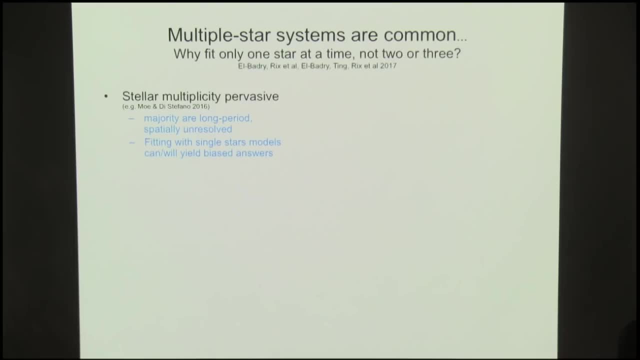 come from the places in the spectrum where theory tells you even that manganese sensitivity should come from. And the last part, the very last thing about what, if you could fit everything at once, is stellar multiplicity. So once you are no longer afraid of fitting 20 or 30 parameters, 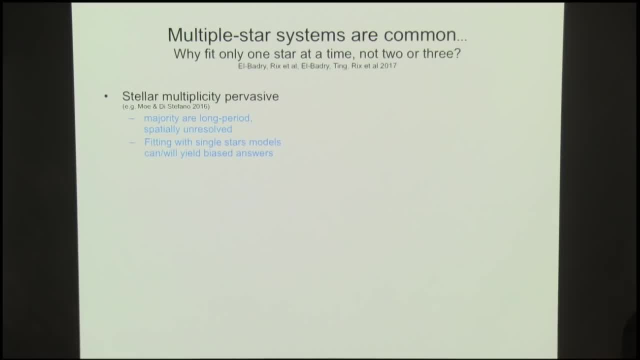 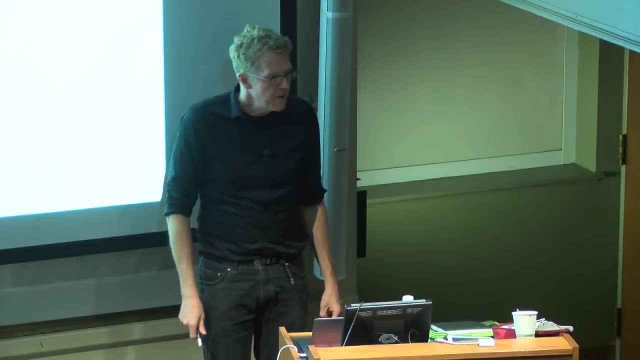 why not go to a spectrum and ask: are you actually an unresolved doublet or triplet? For the spectrum surveys that is very important because the majority, many stars are multiples and in those surveys they are far enough away, they are not spatially resolved and they are long period binaries. 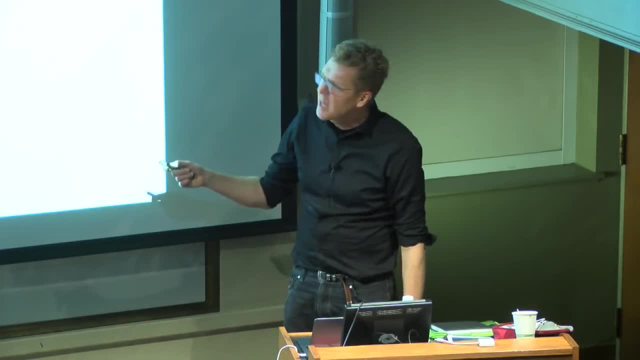 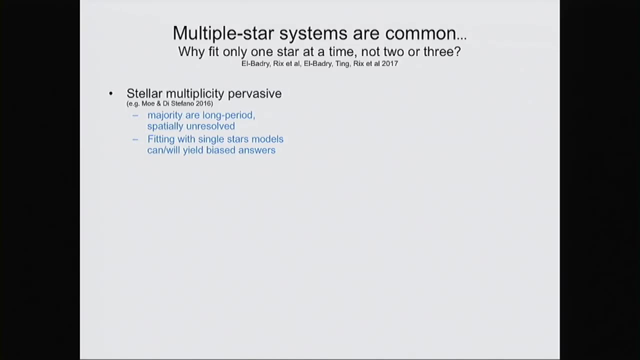 so you don't get a very obvious signal. If you then fit the superposition of two stars with a single stellar model, you get the answer for some hypothetical star in between that represents nothing And that actually, if you care about detailed abundances. so just to show this, 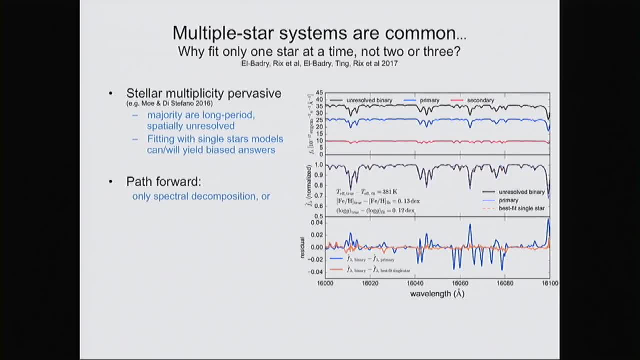 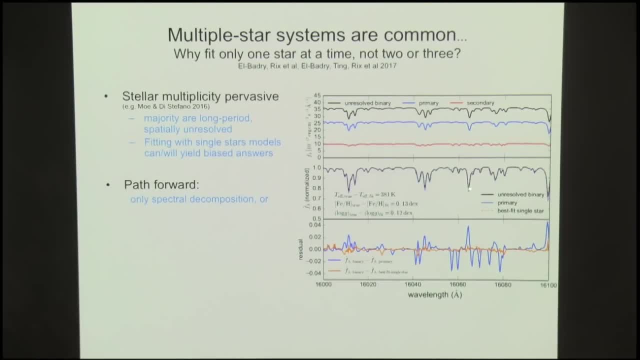 that's the spectrum you have underneath our primary and secondary. you can actually fit it pretty well with a single star that's 380 Kelvin cooler than the primary etc. and some hypothetical object And you have deviations at the percent level. so it's not. it's not like a white dwarf. 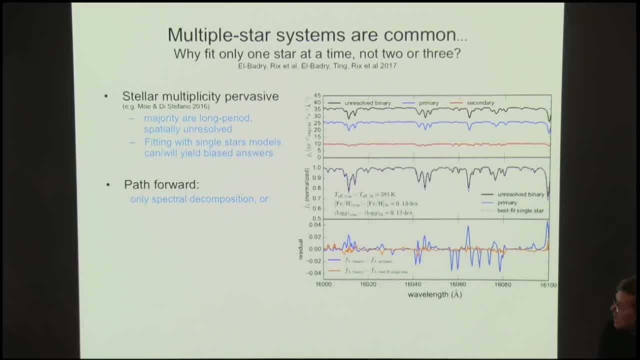 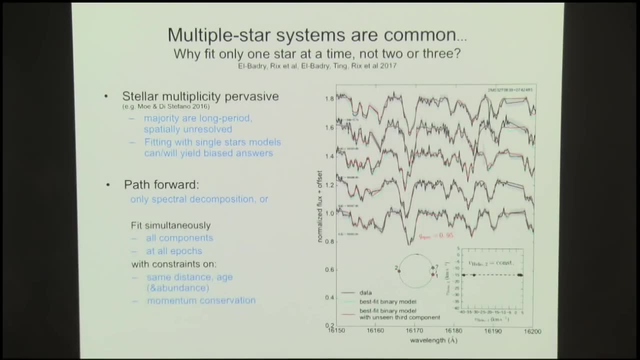 and an M dwarf where it jumps out, So that you can actually do and it works quite effectively and it's actually not that many more answers. But if indeed you have multi-epochs spectra, why not fit all components at all epochs, with constraints that they have to be? 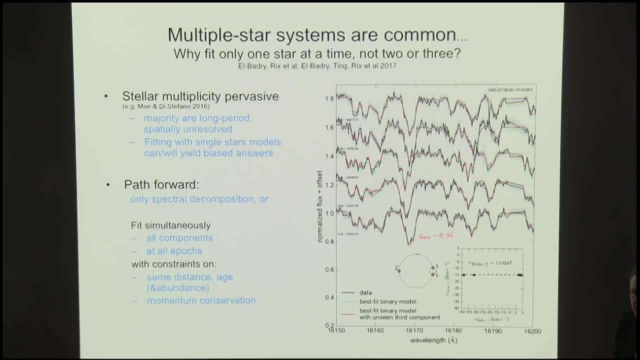 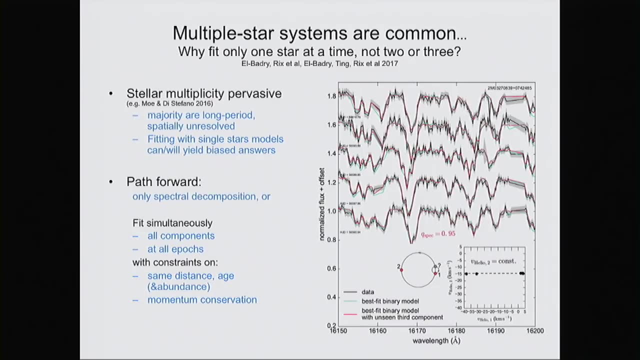 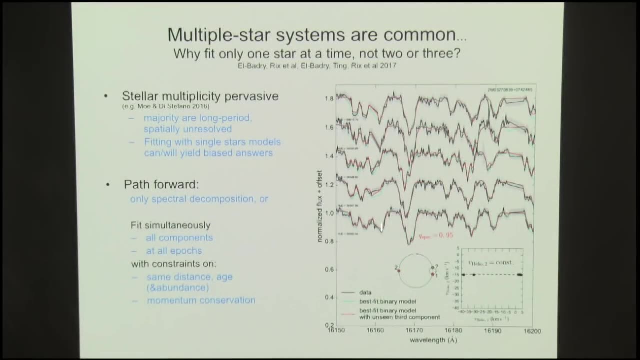 the same distance they have to come from, the same isochrome and also momentum conservation, And that too, that's shown here. that's work that Karim Elbadri did with me last summer and Janssen. shown here is an apogee spectrum. you try a binary. 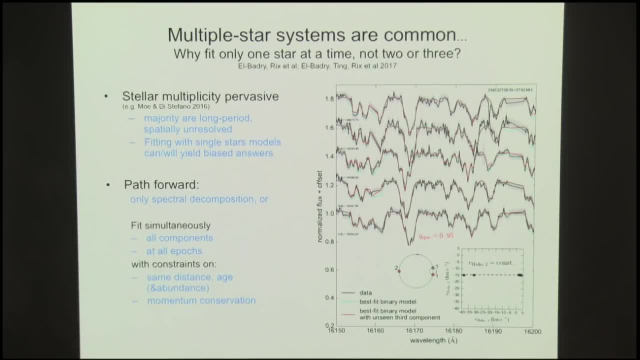 and it doesn't fit. but an unseen third component in a hierarchical binary works well, and on top of it you can actually show that this must be some form of compact object, because given its mass we look very hard. if it was a main sequence star, we would see. 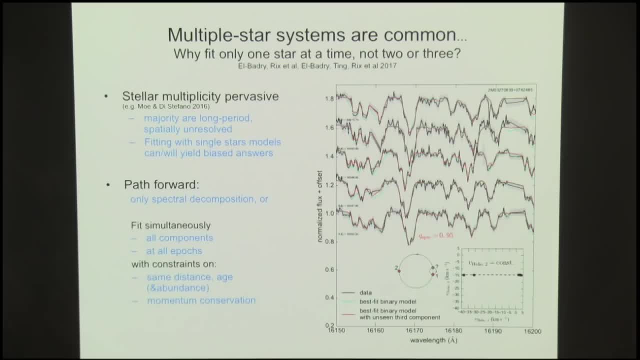 the spectral signature in it. So this is, of course, you know, just a much more subtle version of a double line spectroscopic binary, but you can actually dig in very, very deep, and since I often, you know, I have been accused of being a preacher for low resolution spectra, 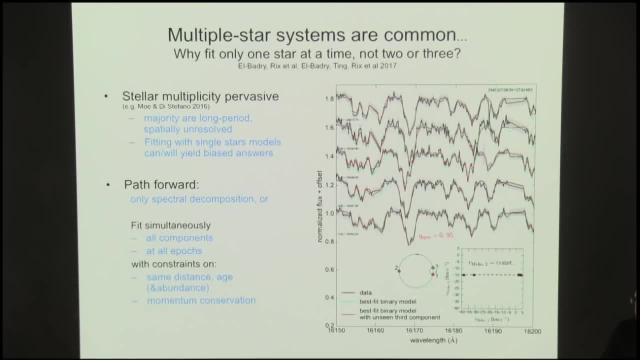 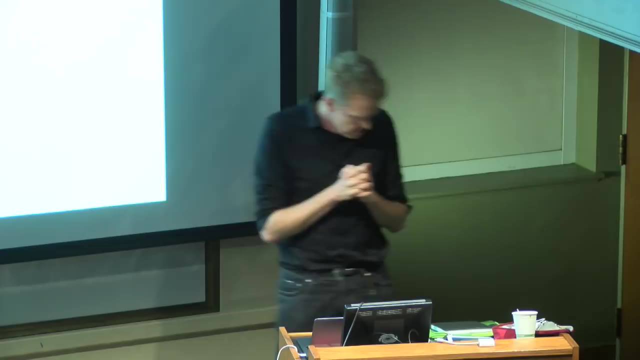 that type of stuff. as soon as the velocity differences are more than four or five kilometers a second, with resolution, 20,000 spectra, you can dig it up. So let me, before I become a used car salesman, give you, give you the, the upshot. I think. 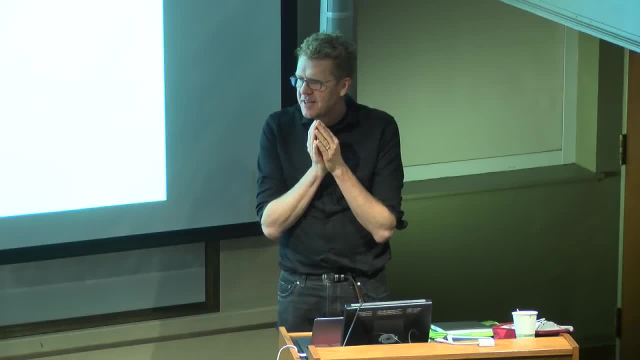 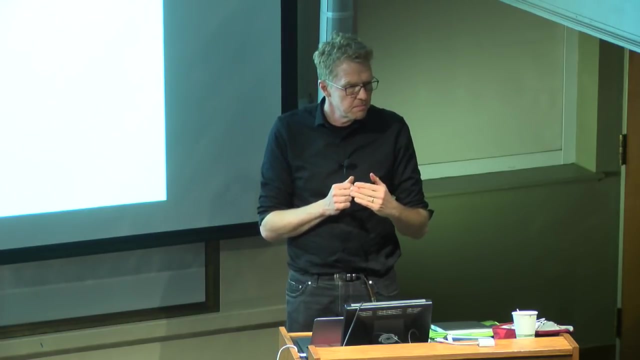 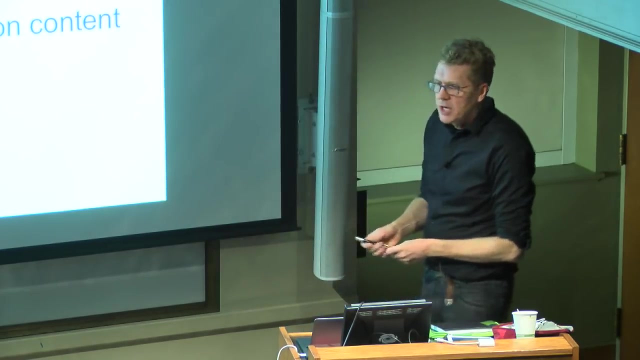 you know, we have been in this uncomfortable situation that, despite all the beautiful effort of physical models, whenever you applied them to this big survey spectra, out came either demonstrably suboptimal results because you had to just pick special lines or systematic issues. I think the combination 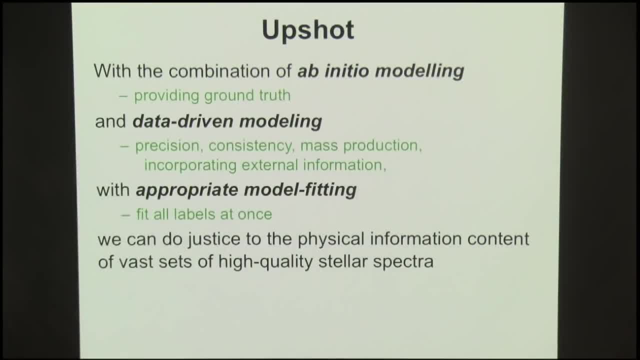 of doing the correct physical model under the circumstances works for just a few cases. high resolution: take clusters, take binaries, whatever circumstance works well, gives you the ground truth. the data driven modeling gives you precision, consistency across surveys, easy mass production and I have shown you with astro seismology. 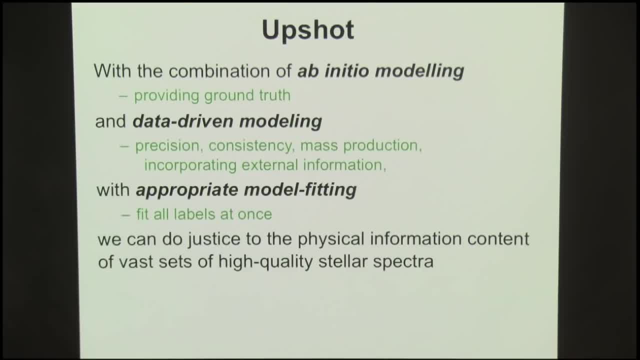 an easy way to incorporate external information and at the latest next April, when all of a sudden Gaia gives us luminosities, all the stars, because the question of how a Gaia parallax makes a spectroscopic analysis better is actually a non-trivial question. 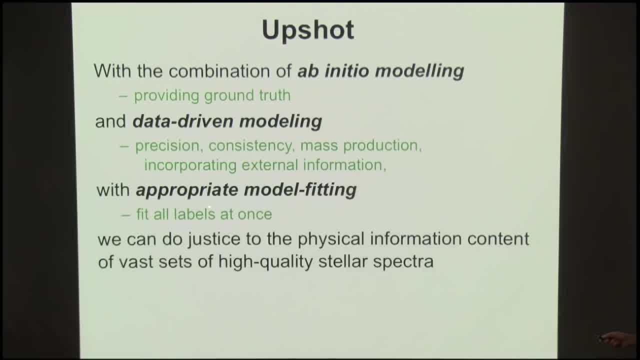 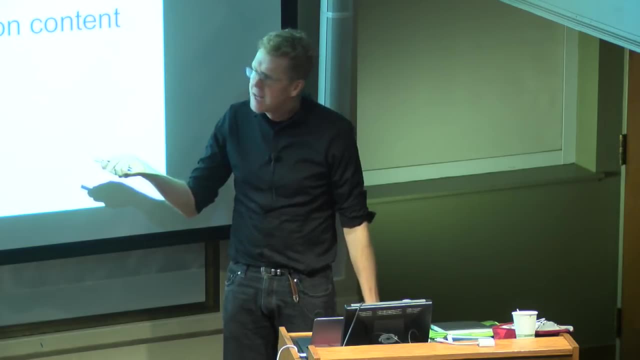 and if you do the appropriate fitting, then you can also deal with the covariances and you get unbiased answers. and so this combination to me, even in this world of spectroscopic surveys, now gets us a lot closer that we can do justice to the information content. 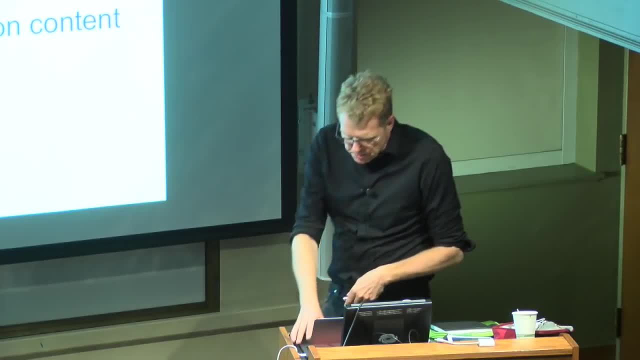 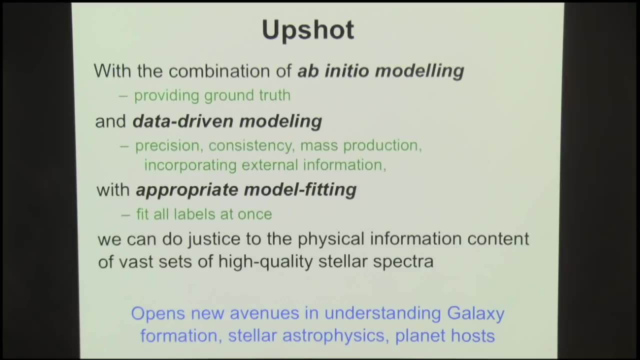 of those vast sets of high quality spectra. that opens up new avenues in understanding galaxy formation. I've shown you one example. initially, if you have ages throughout, you can kind of see the Milky Way build up metal. it's a production of different radii and drifting away. 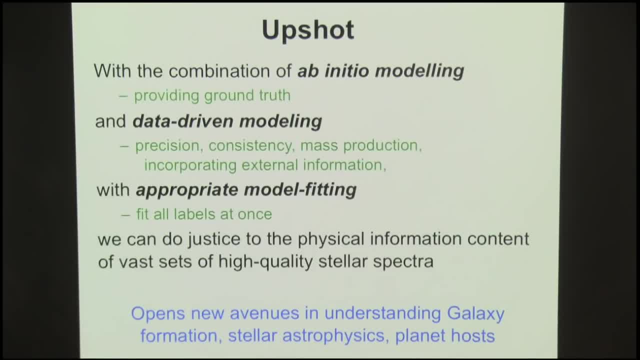 but of course this is a very sketchy picture. there's a lot more stuff to be sorted out. I think having just these constraints for for hundreds of thousands of stars will teach us enormously much about stellar astrophysics- things we don't know. so my, I think actually. my guess is still that Gaia will be remembered as much for improving stellar astrophysics than the knowledge of the Milky Way. of course. stars with planets- on all of these we can get a lot of precise stuff, and it'll teach us also about a census of multiplicity. 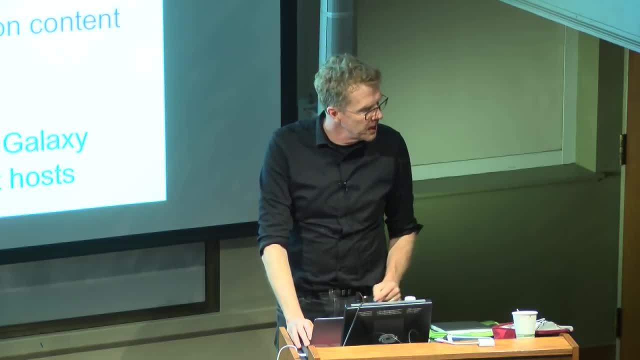 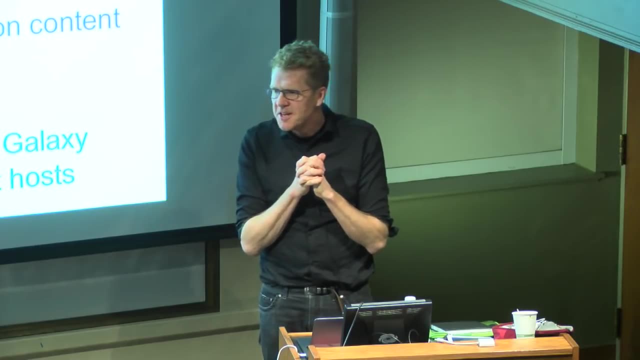 which, for example, the question of how many black holes there are in the Milky Way, I'll come to in just a second. so this is why I personally feel now in a position to look forward to the next surveys, because I feel strongly if you haven't demonstrated. 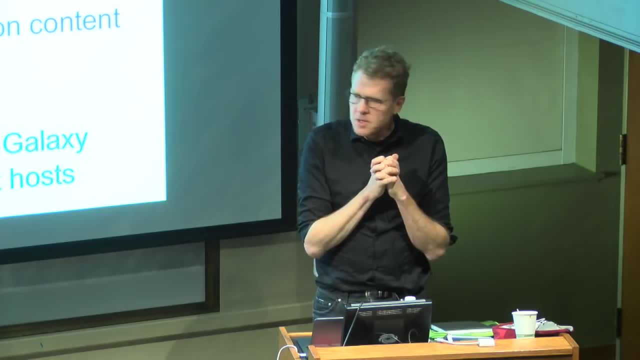 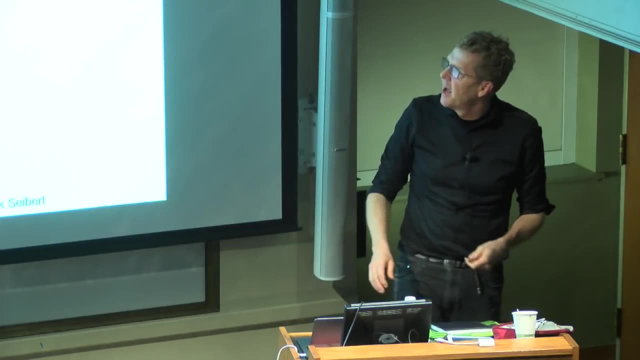 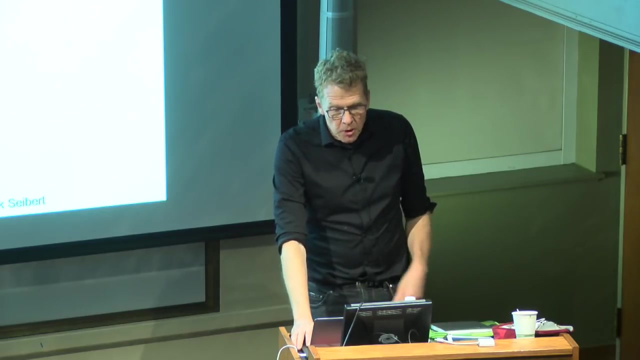 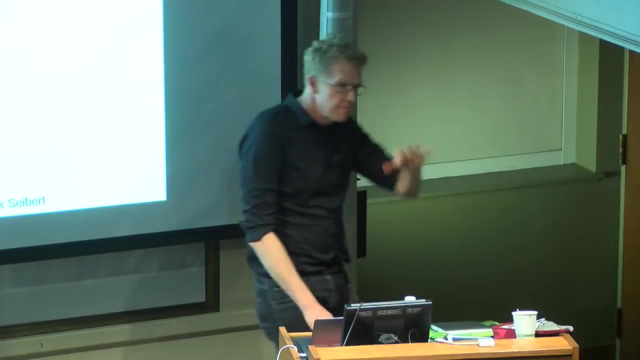 that you know what to do with the data at hand. you have no right to ask for more, and this is why I've actually am now spending a lot more, a lot of my time on Sloan 5, which is not your grandpa's Sloan survey, at best, I mean. 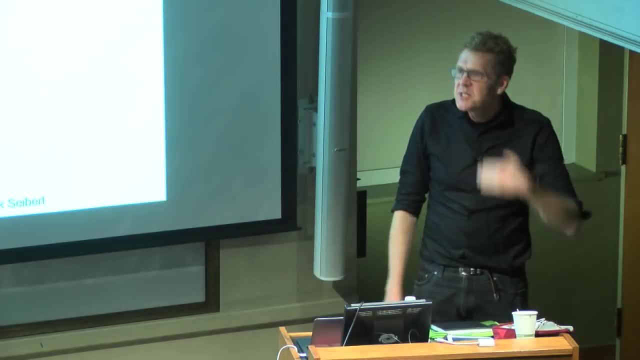 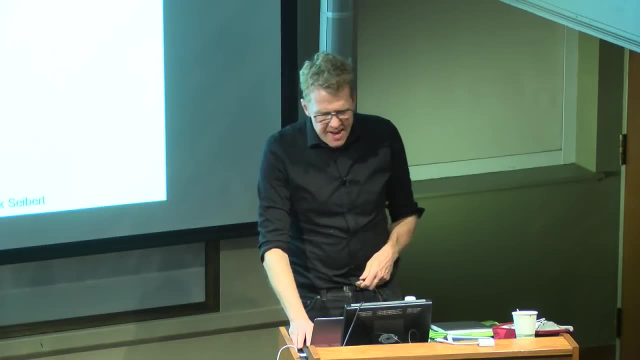 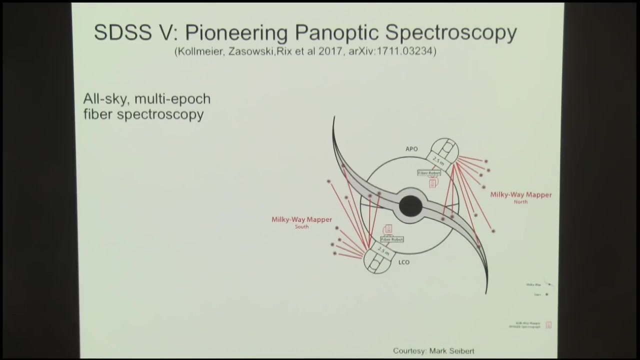 Jim Gannon, not Daniel Isaacson Stein. it is no, it will no longer be a galaxy survey. it'll actually be an all-sky, multi-epoch stellar survey which we like to illustrate in this kind of medieval looking view of the world, right with spectrographs. 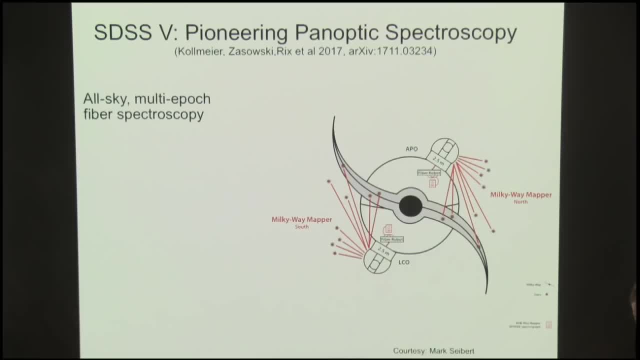 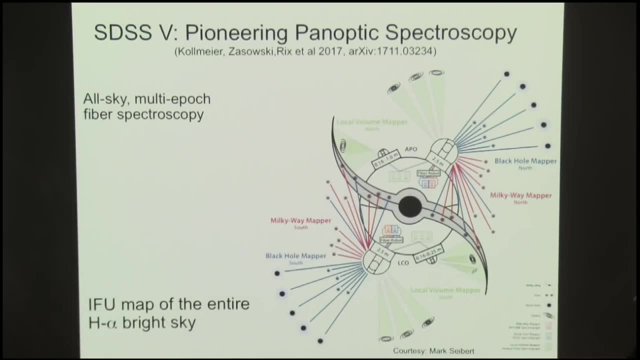 in both hemispheres, that you can look anywhere on the sky that you know we will also make an IFU map of the entire H-alpha bright sky and you know we will look at six million objects, mostly giants by number, to map the Milky Way. I'll show you. 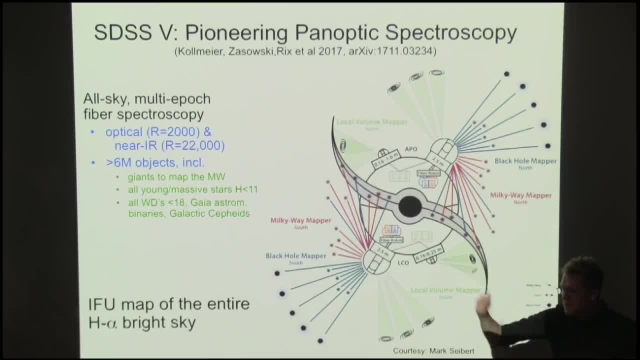 some of that. but also, while you are, we will be going across the sky repeatedly, so if you're coming by each part of the sky repeatedly, you might as well think about what is multi-object, multi-epoch spectroscopy, multi-epoch spectroscopy that I can do. 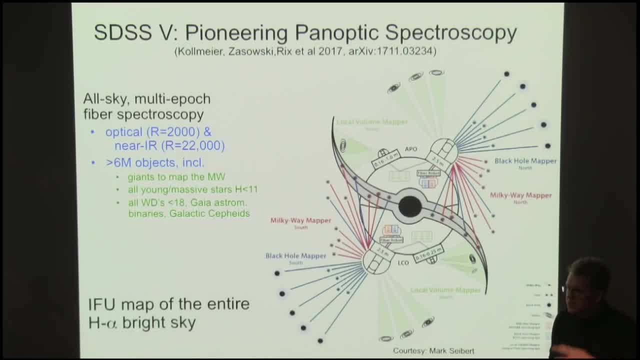 especially if the number- ah, let's just do 10,000 more of these- is not scary. so we will look at all young and massive stars, repeatedly brighter than 11th magnitude. we can look at all. Gaia identified white dwarfs to sort out the origin. 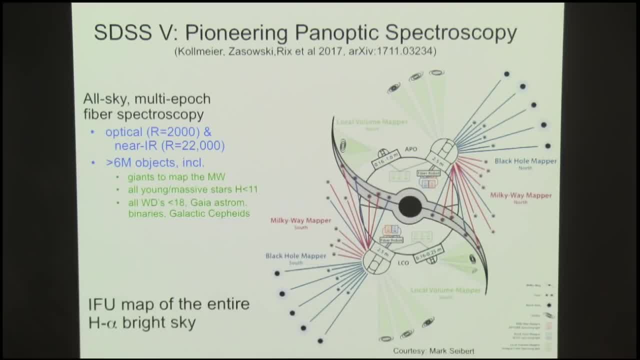 of type 1a's, um, all the Gaia astrometric binaries. actually, if you have one good spectrum to solve for the visible companion, you have solved the system for me. so one spectrum will do it, and galactic cepheids, which, to my mind, 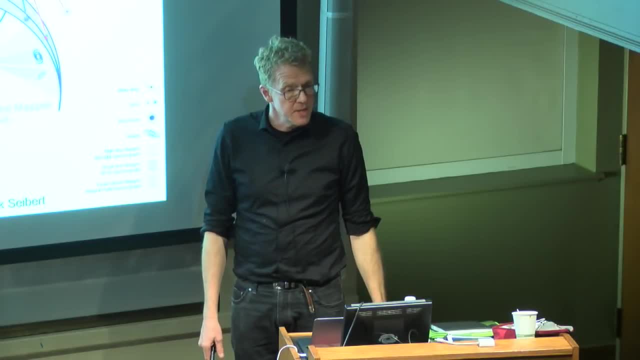 are only the stars that have encased the interstellar medium, placed in a 5000 degree photosphere, so that I finally actually get to look at all 20 abundances that the interstellar medium had, rather than being confined to oxygen and nitrogen, if you wanted to see. 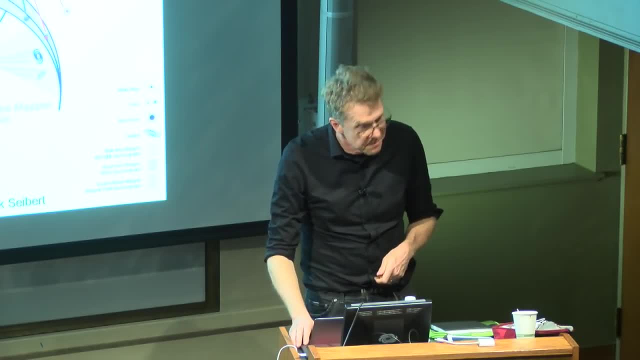 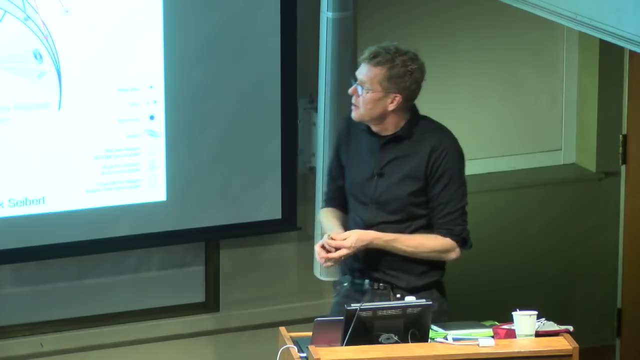 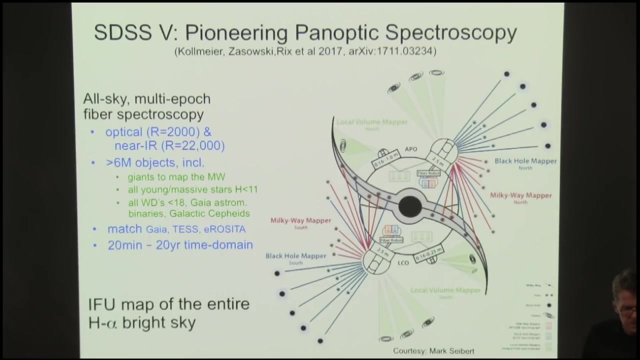 on what time scales the interstellar medium needs to be stirred or is being stirred. and the other thing is this survey goes bright and across the skies, entire sky, and that's actually very much in vogue with a lot of the space missions that are going on. 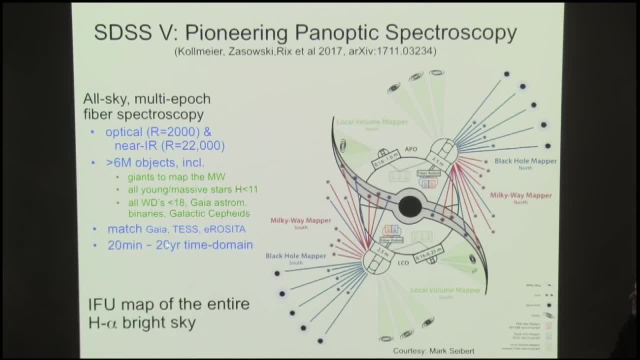 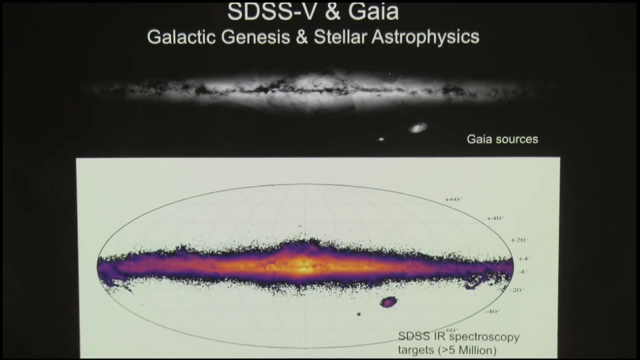 coming up and, given um Sloan's legacy and the survey structure, you can actually get time information on these time scales. so the philosophy is: stay bright and survey fast. now you might ask: why do you know? so this is what I mean. why is this survey matched to Gaia? 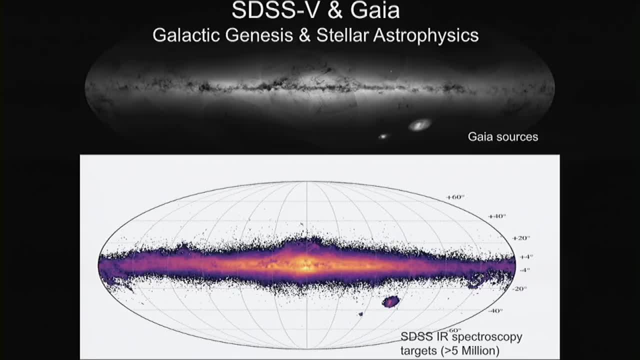 this is the Gaia source list, not an image. this is the Sloan 5 Apogee source list, not an image. now there has been this funny thing, since so many stellar surveys have been piggybacked off galaxy surveys. you know the, the one percent. 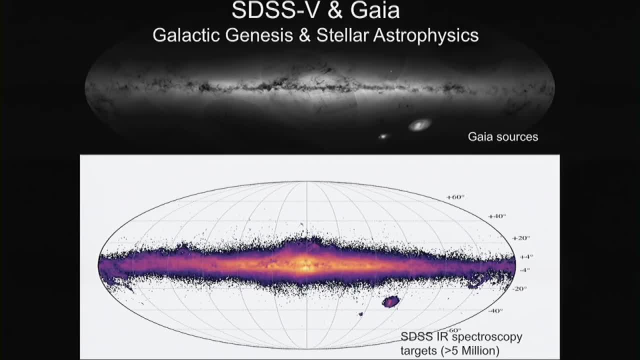 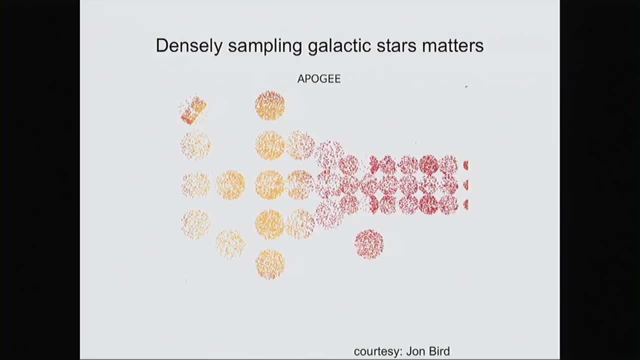 of stars in the halo has been studied so much more than the rest of the Mercury, and so, um, I want to close with showing you why densely sampling the galactic stars may matter. this works well for a good, over educated audience, like I can expect here. so this is 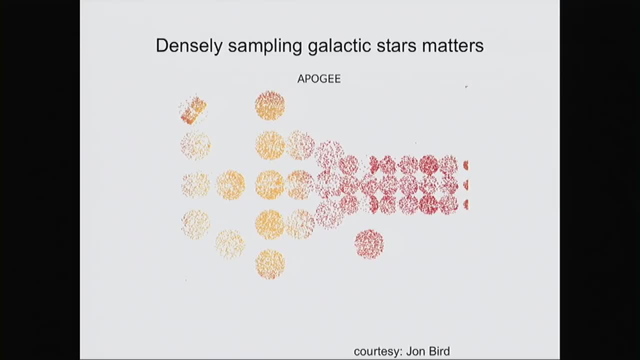 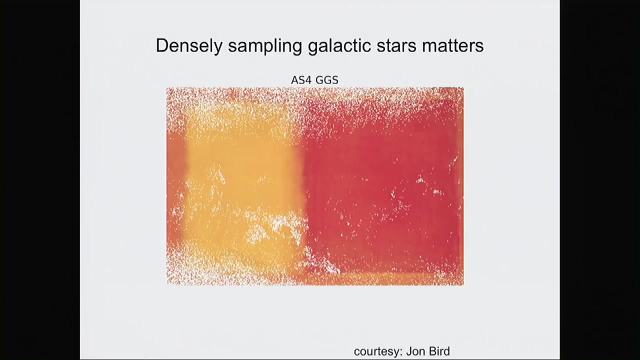 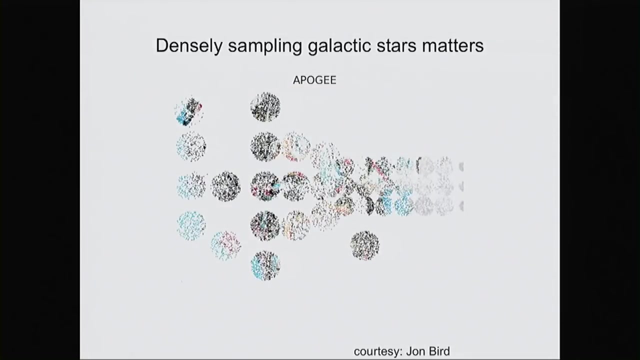 an art history quiz. I have sampled a painting by an American painter the way that Apogee currently samples it. what's the painter? Rothko? and you will say: oh, why did you spend so much time sampling it? I have sampled the Apogee style a painting. 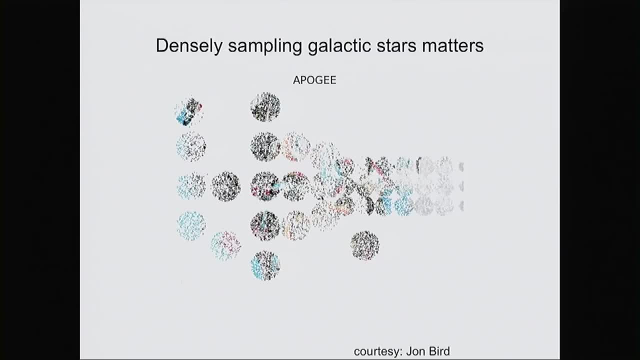 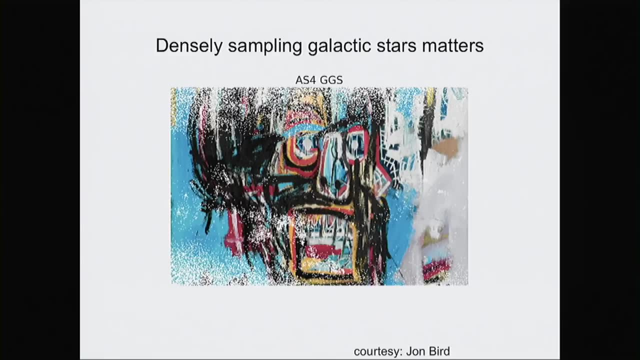 by another famous American painter. I gave this talk in Strasbourg three weeks ago. somebody guessed it, somebody said it: Basquiat, that's true. so the point I'm trying to make is we don't know how much small scale structure the Milky Way has. there's reason. 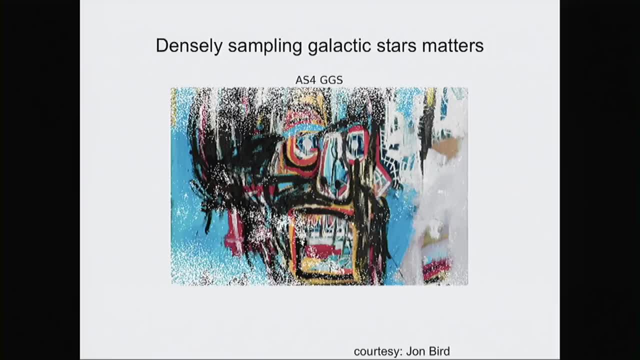 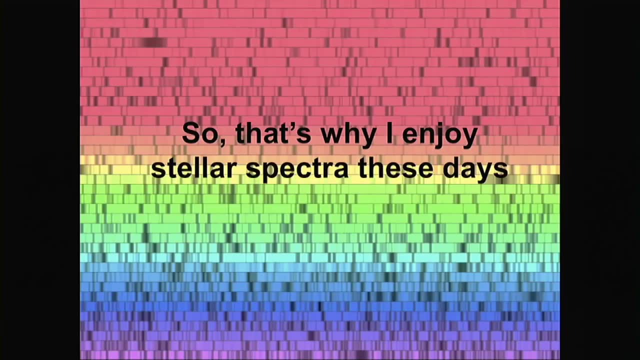 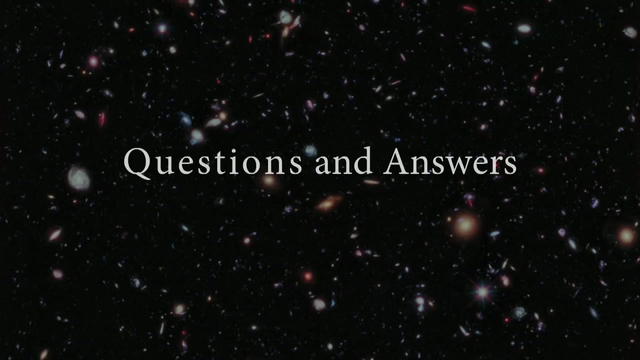 to believe. it has a lot of small scale structure, and so the best way to find out is by looking at the information content in Joy's spectra, because I feel we can do justice to the information content a lot better than we did in the past. thank you, 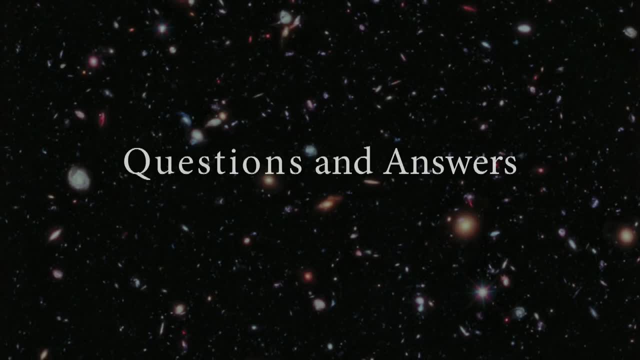 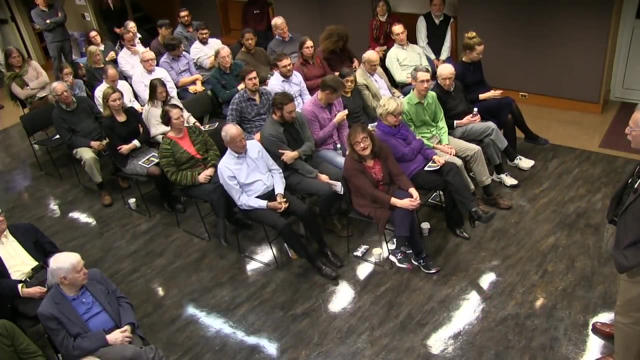 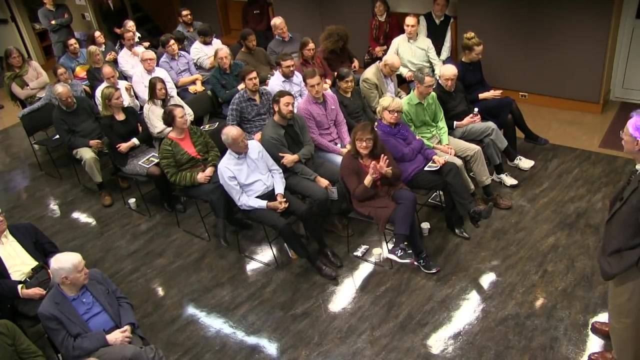 thank you very much, and the talk is now open for questions or that. well, you've given us a lot to think about and I think, looking at your method, as I was able to understand it from here, it seemed to me that there might be a possibility, even though 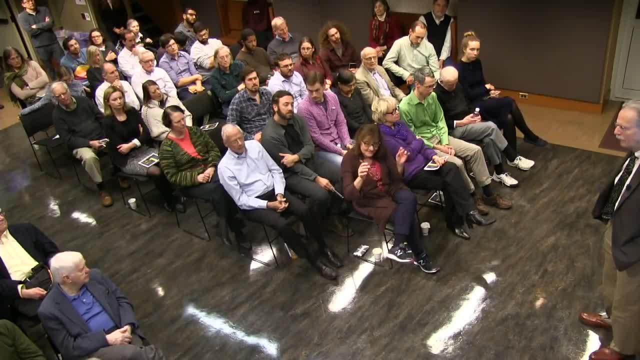 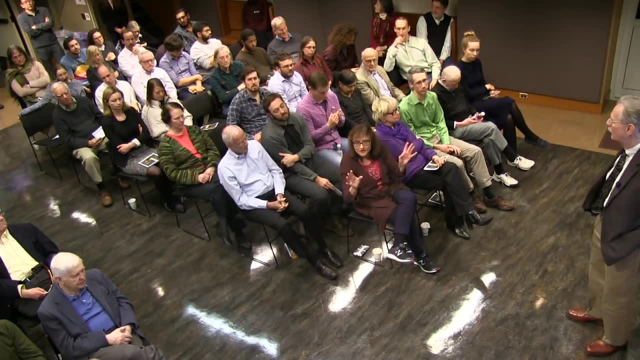 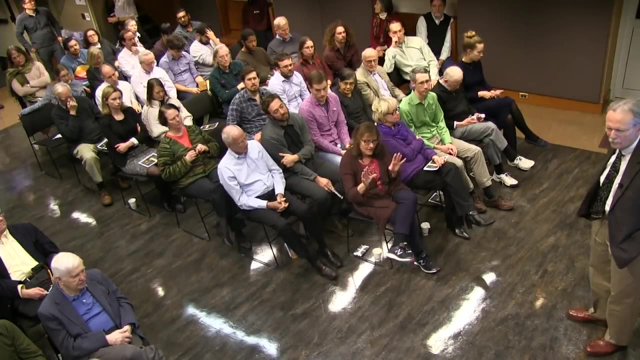 the focus that you have is on these very detailed spectra, that it might be possible to actually decrease the number of variables that you're observing and, in fact, as you know, as we look at the sky, we have many more. that take this in a somewhat different direction. 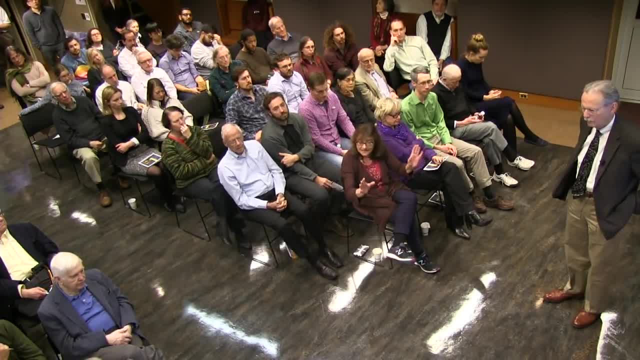 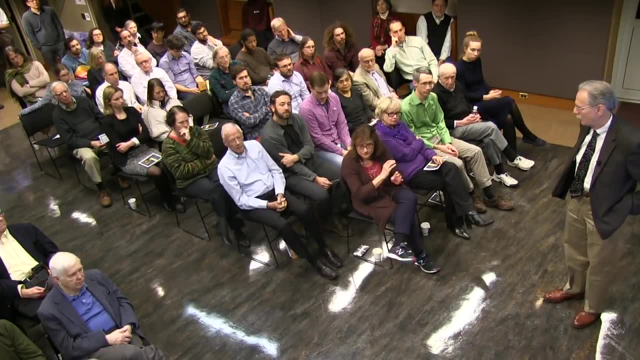 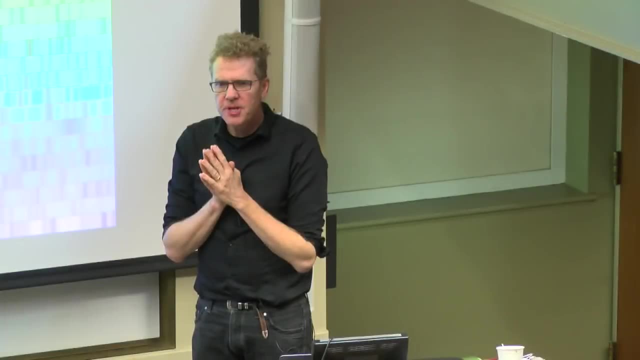 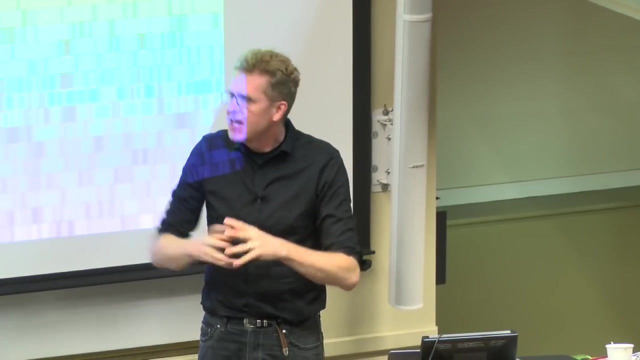 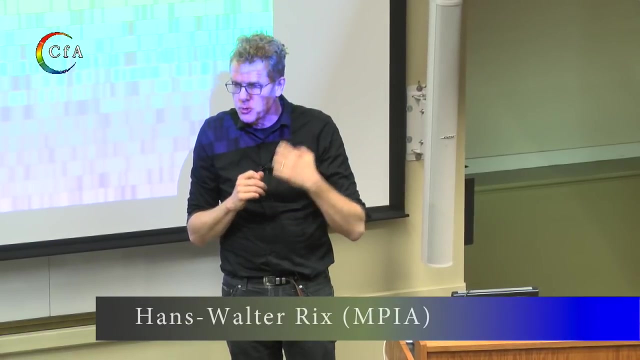 use the same kind of data driven method, perhaps not get the same detailed results, nevertheless potentially important results by looking at a smaller number of observed variables, whether they're broadband filters, position on the sky or in the sky, and so we have a very interesting question about how much. 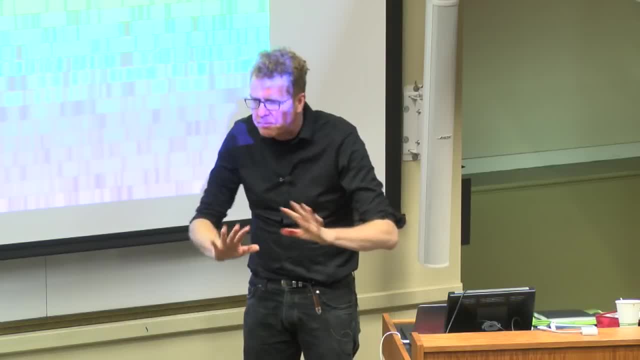 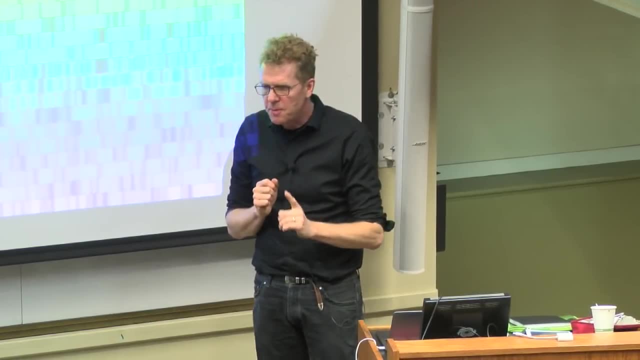 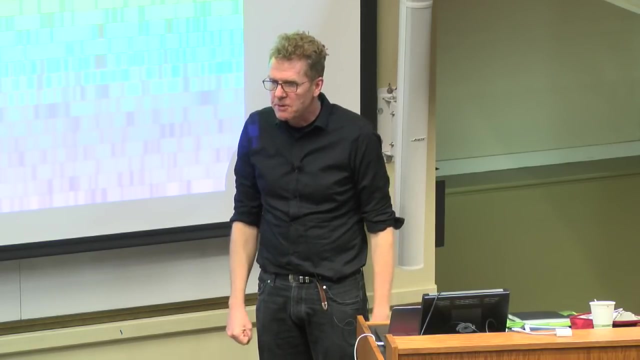 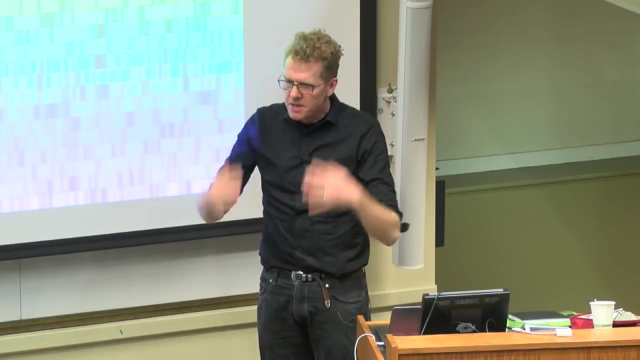 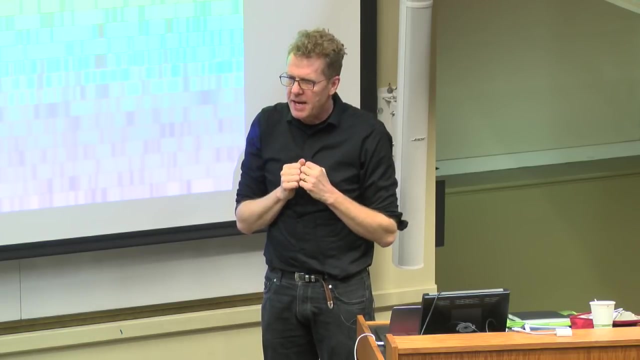 information is in those, and so the fact that for 100,000 of those we have beautiful high resolution spectra that tell us that right, there's a very interesting question. so I think the general principle: these properties are not a a function of the observational setup. so let's. 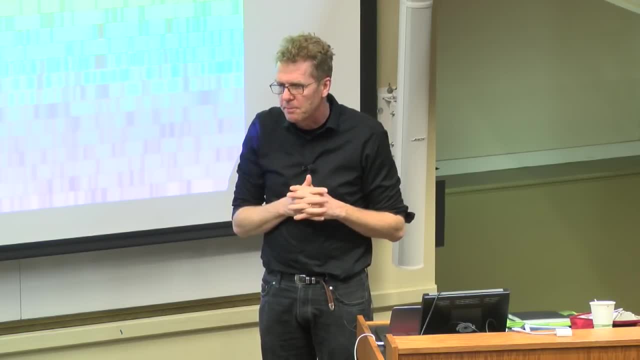 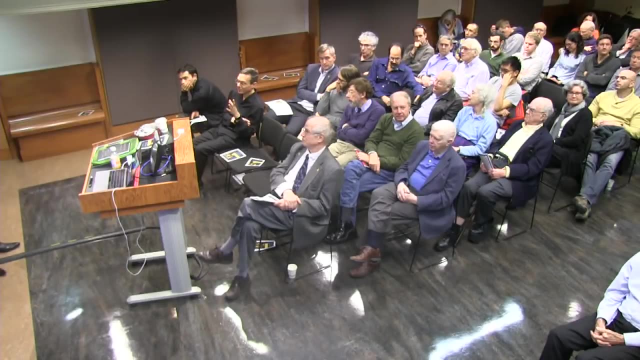 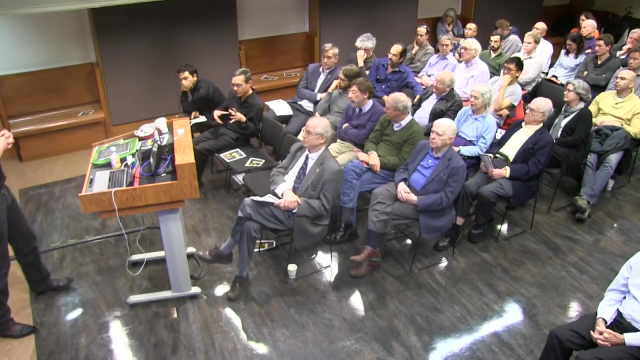 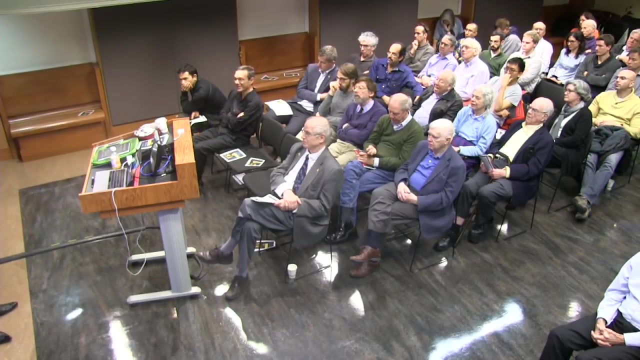 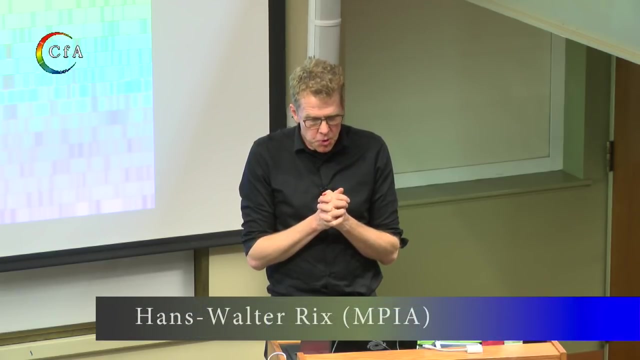 get a number of examples where we know the answer. and this is the funny looking data set. I think that is the the only reason why not try to fudge the theoretical modeling such that it fits the data and we make the best out of it, and the 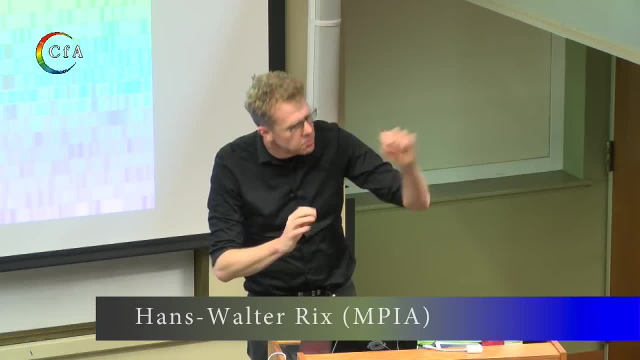 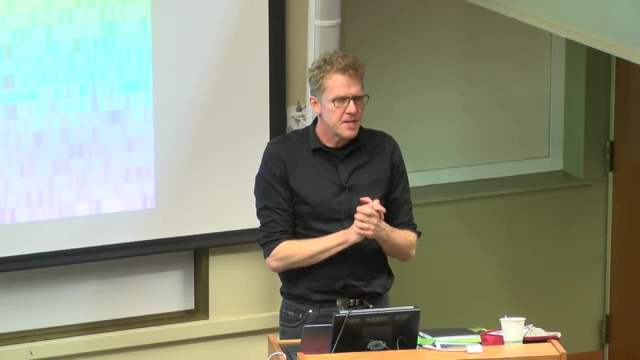 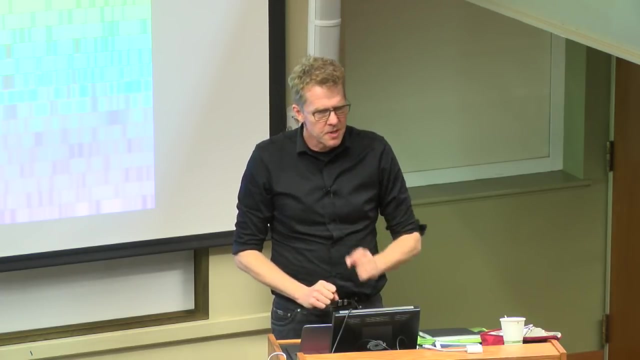 second is to look for anomalies and try to learn something new that we- I would argue that the problem that I want to solve is the evolution of the Milky Way. I want to get the ages and, if I know how to transfer the physically motivated mass age estimates from astro-seismology. 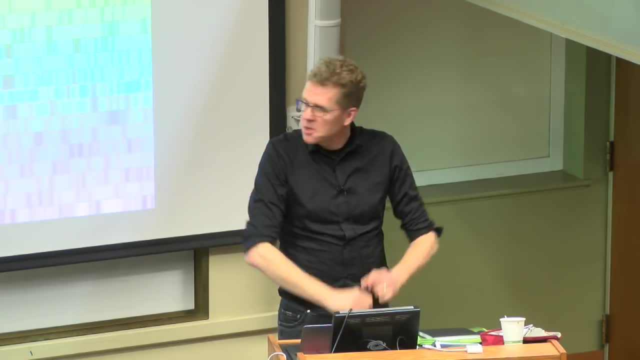 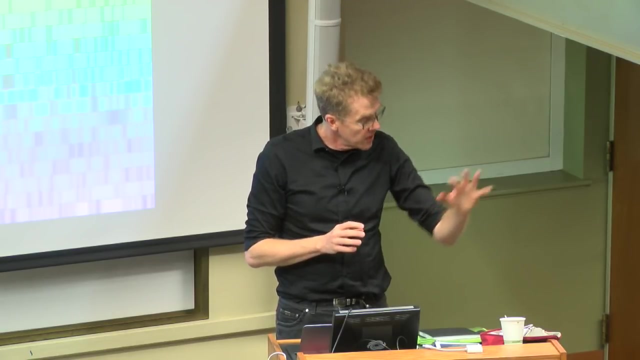 to their spectroscopic signatures. there's nothing fudgy about it. On the other hand, I would say I think I would just like to relieve the community that builds ab initio physical models from the pressure to deliver mass production, because actually then they can focus on getting exactly those physical issues right. 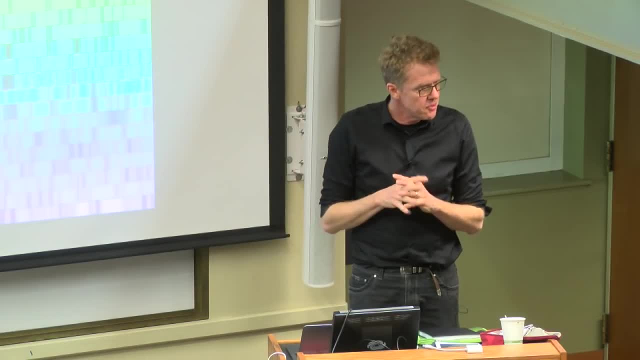 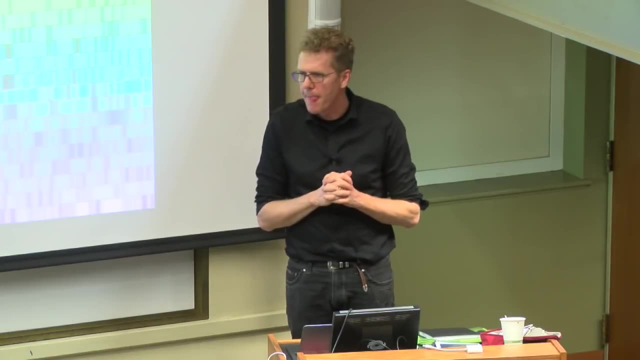 And the question of how some of the stuff learned from data-driven modeling could actually feed back onto the physical models is an interesting one to discuss. What a relationship. It's a great question actually. I was wondering if the field is actually in a kind of intellectual balance. 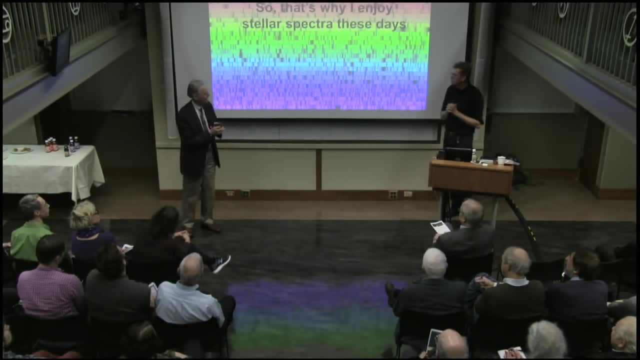 between modeling and data-gathering interpretation, because very large groups of people appear to be working on these various surveys. I think there are relatively much smaller groups of people doing ab initio models. Is the field in balance in that regard, or should there be more effort in the modeling and less on the spectroscopy? 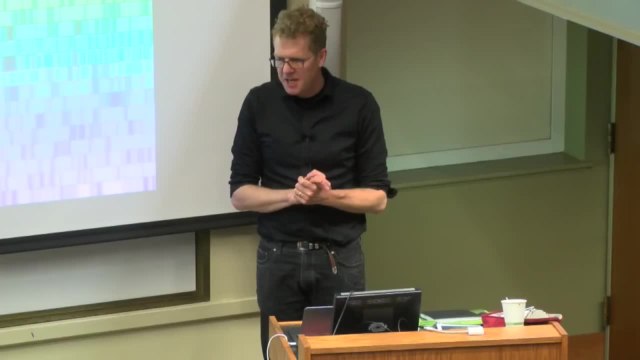 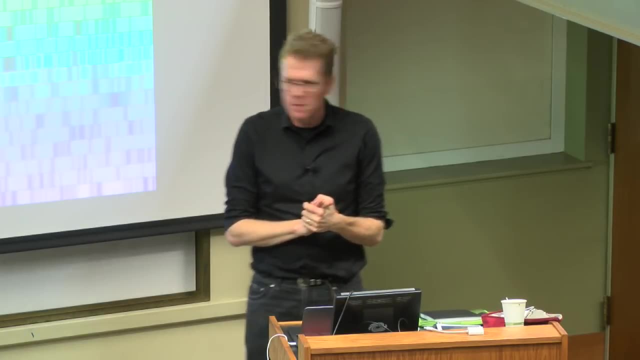 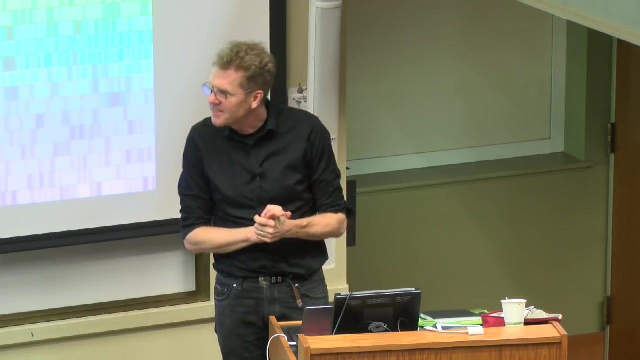 Where So? so Well, the and my personal answer, as I told you, is: the last two staff hires were two research groups in building real. you know this is the 3D non-LTE hardcore crowd. So this is my- not with my feet, but my wallet. 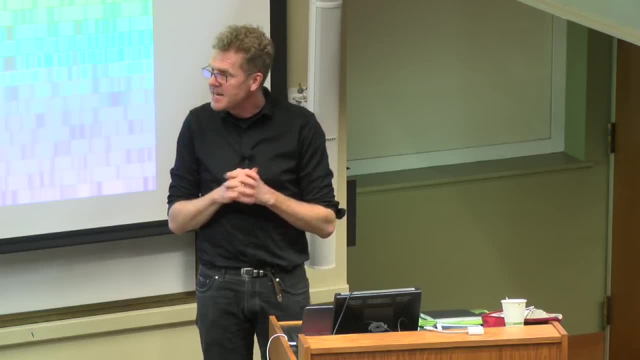 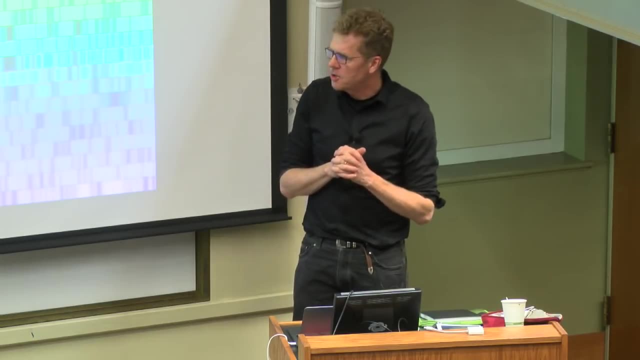 So this is. I think that is an important thing to do, and the question is how I can make this a gratifying and promising career prospect. Um, I do. I think that in the- I mean, it is actually, I found it in new surveys. 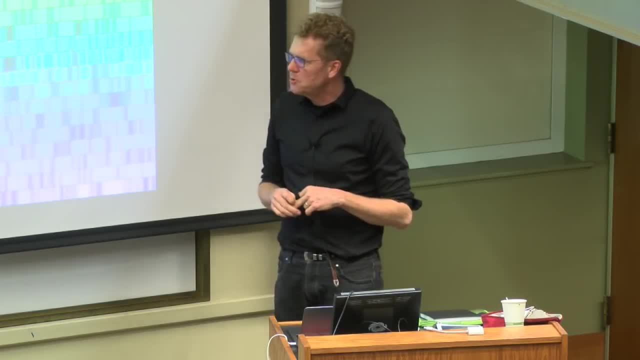 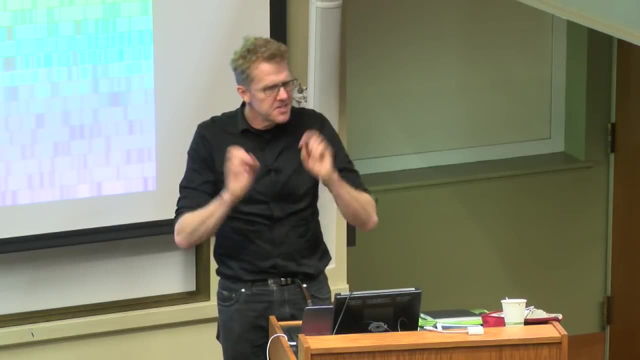 if I say: you know, I think we can actually re-reduce the entire survey on a desktop that actually has threatened a certain subset. It's sociologically an interesting thing to look at, but again, actually I should go back to re-reducing. 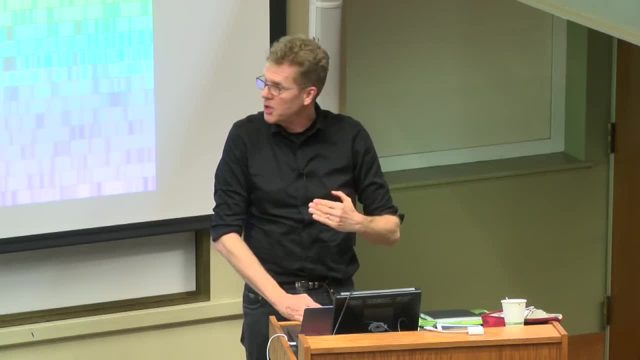 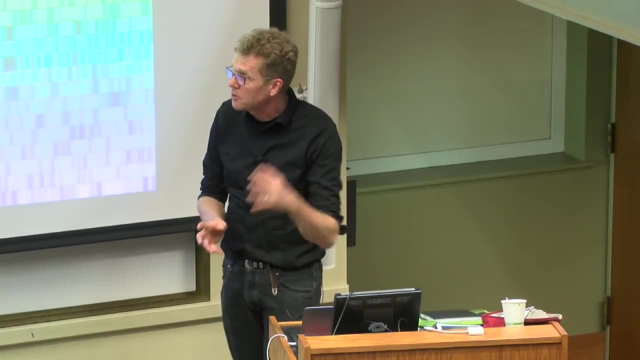 Whenever one learns something new, say, there's a new generation of ab initio models. you re-calibrate abundances, you propagate it through the next million spectra and you're done right. So you have a fast way of propagating that. 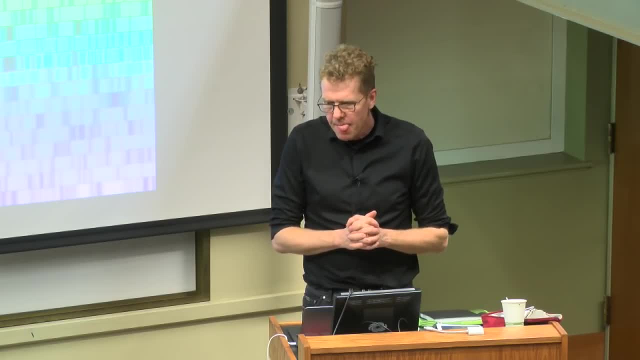 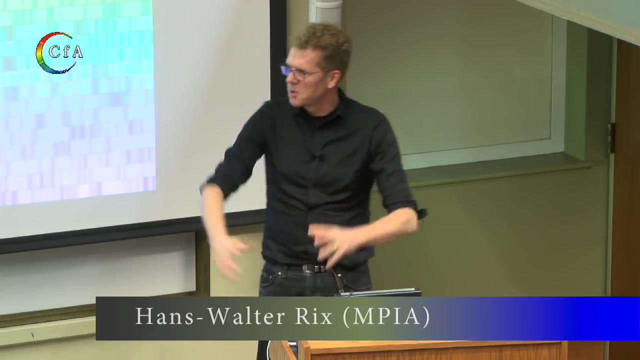 But um, I do think, um. I mean I don't have a particularly informed sense of One of my colleagues. Carol Lind also ties very much into the atomic physics, folks right, She works on one element. she says: 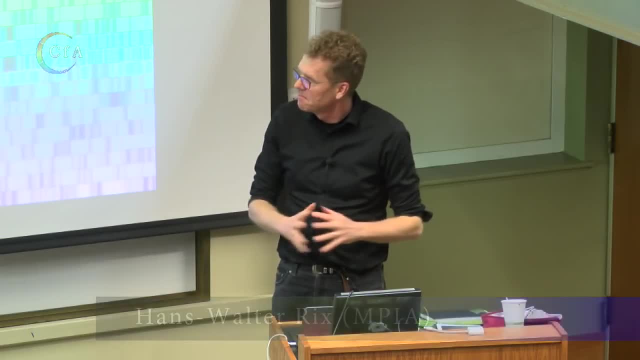 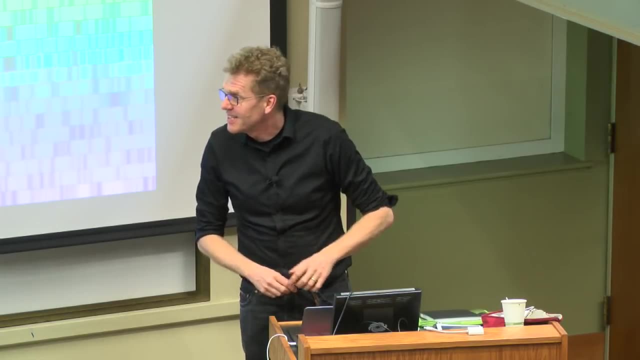 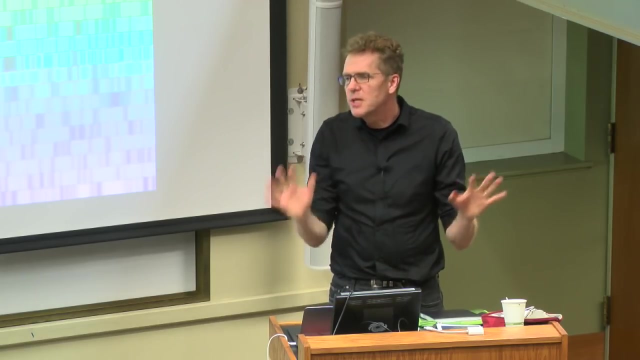 next three years and once I got that, you know she's going to turn to the next one. I think that's A lot of elements. I would say That's the kind of jokes that make her cringe. So I think the question when it comes to individual elements. 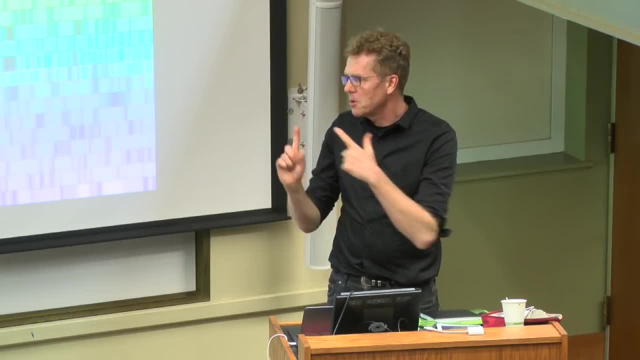 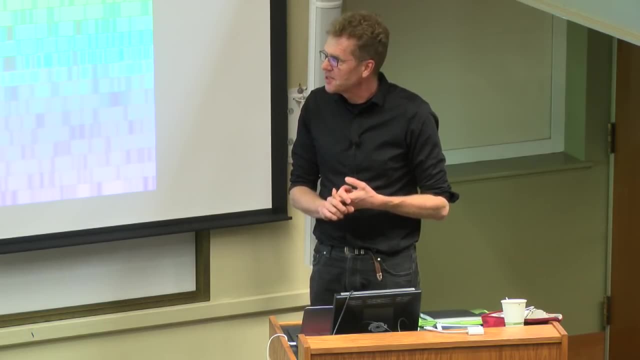 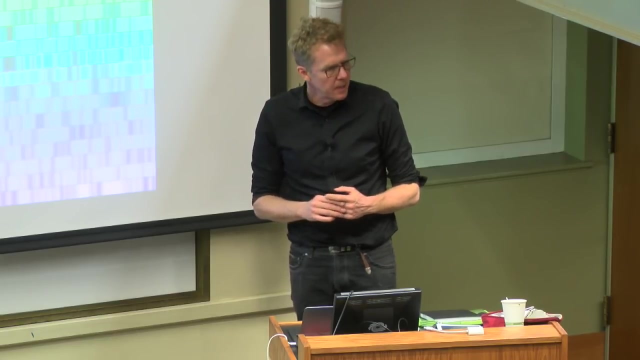 there's a question of: I wanted to know ages, I want to have tracers of the four or five main nucleosynthetic channels. So I think it's It's one that we have to go back and ask to actually care about each element. 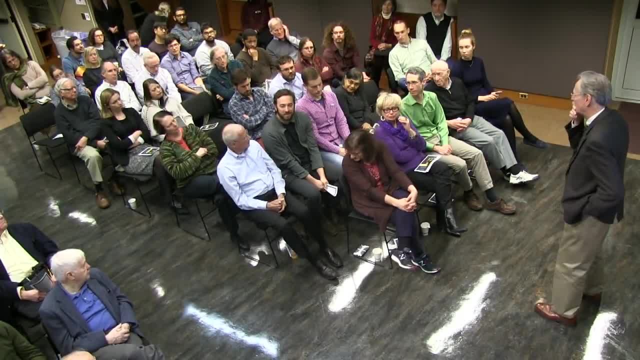 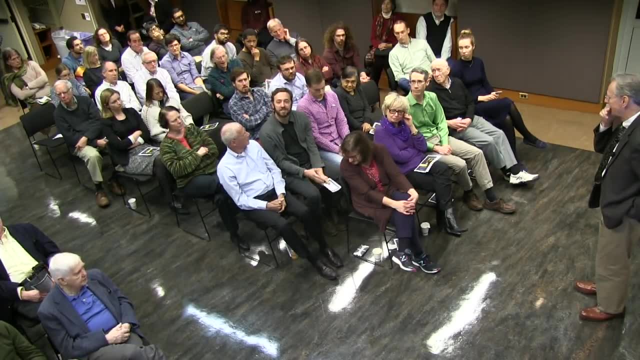 Yeah, so, um, all these machine learning tools are all based around the fact that you have a training set, and it's only as good as your training set. And one thing you said is that you trained a cannon, for instance, on astro-sizing stars. 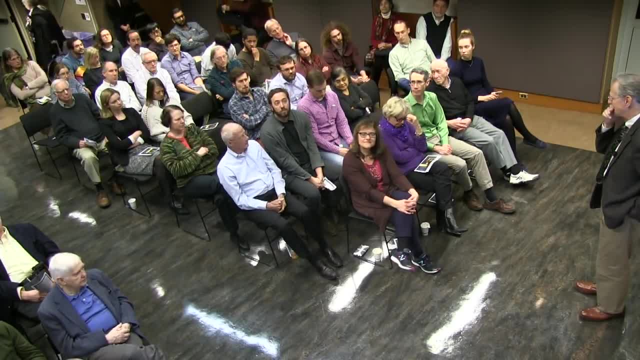 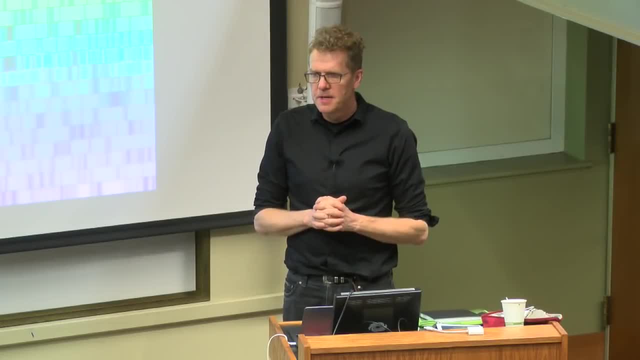 which from Kepler, and they're all giants. Yep, Does that mean that? What do you do about dwarfs And Ah, So I think, I think it is true that building this model, as soon as you apply the model to a part of 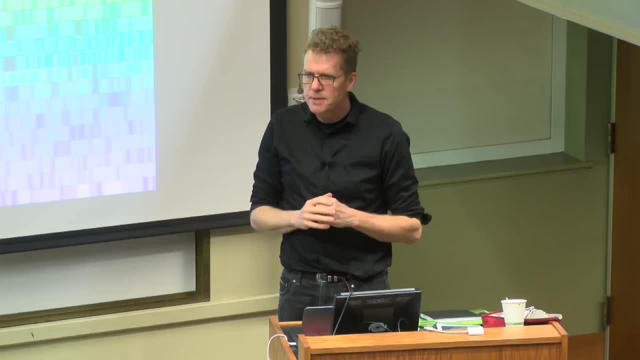 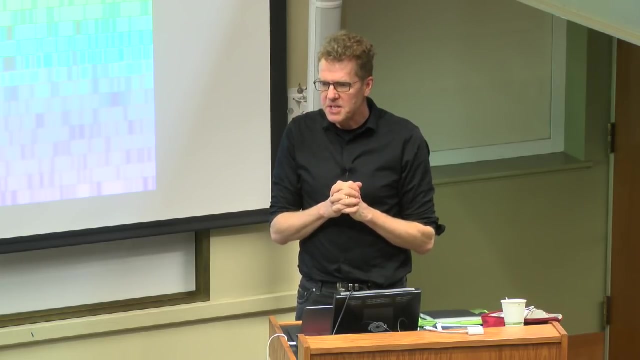 label space well beyond the training set. it actually is an extrapolation, and extrapolations tend to be irresponsible, So this is why this has to be used responsibly. I think it is true that you know, as the astro-seismic data in metallicity and other. 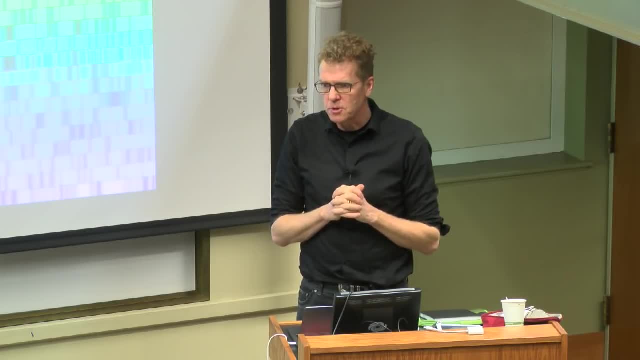 things build up. That is, That is a useful thing to do. So I think the This whole thing is limited by the ground truth, You know, unsurprisingly so, And so It's the same thing. the question is, how good are astro-seismic masses for very metal-poor? 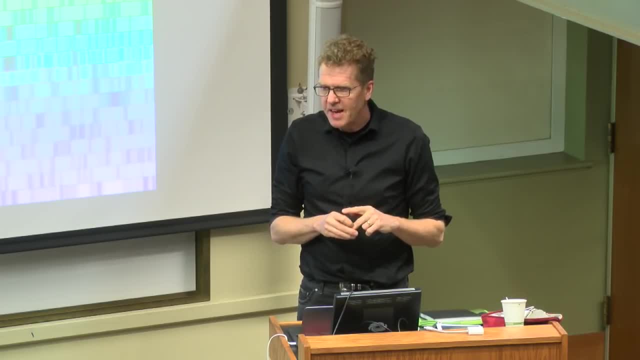 stars. Right, That's a variant because actually for metal-poor stars the ages might be particularly important. Go ahead A kind of you know related question. So how do you, How do you, How do you? 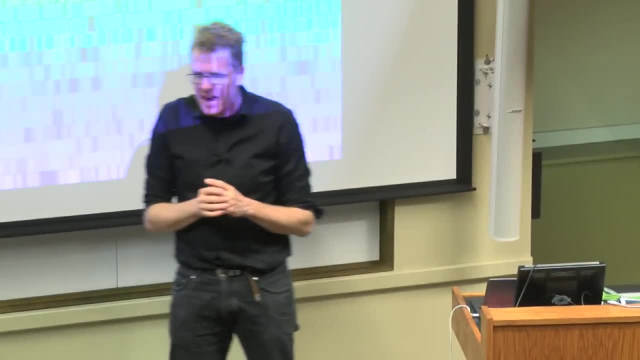 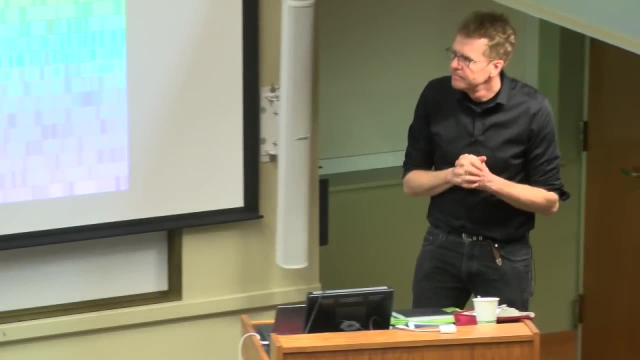 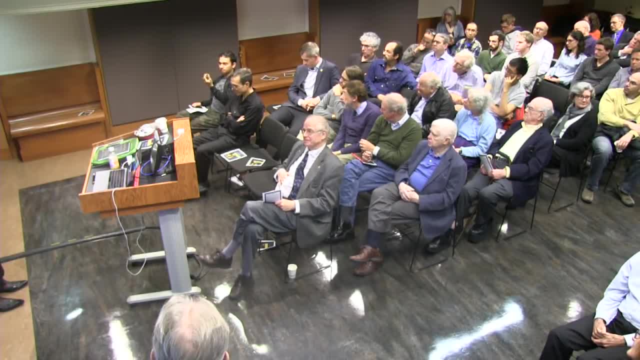 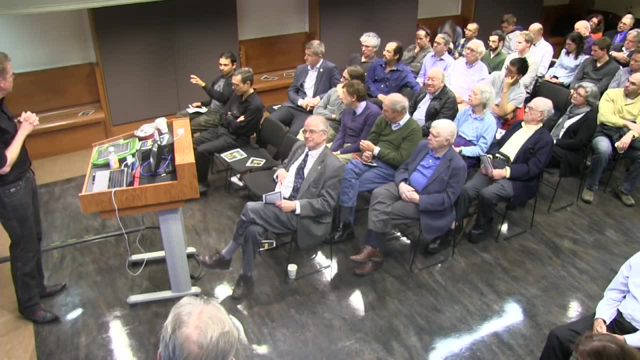 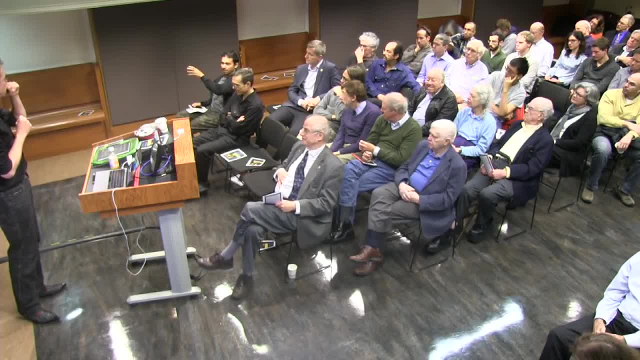 See Deals with, let's say, degeneracy. So in number 1, some, as you said, I start with the same labels. I mean I, I made that suspect a. But imagine another star that, for instance, has different. 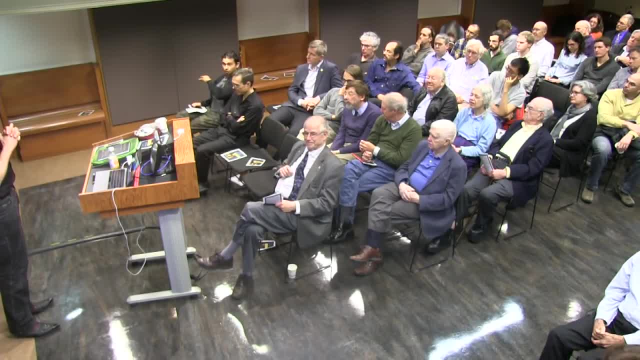 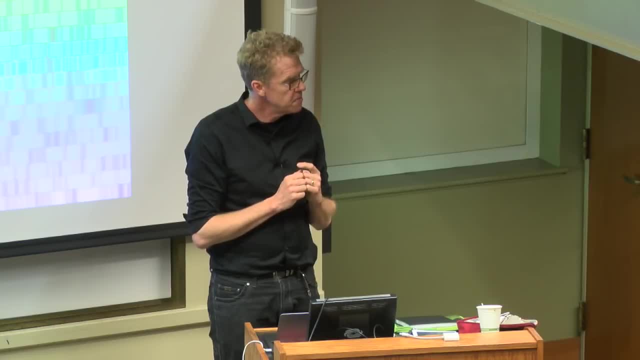 They doing like that, Can you a very strong in their field. This would change your spectra and then all the other parameters are exactly the same. So in a formal sense, if labels that I specify are covariant and then I specify: 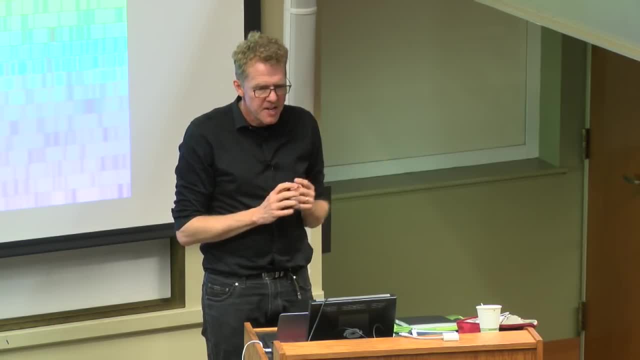 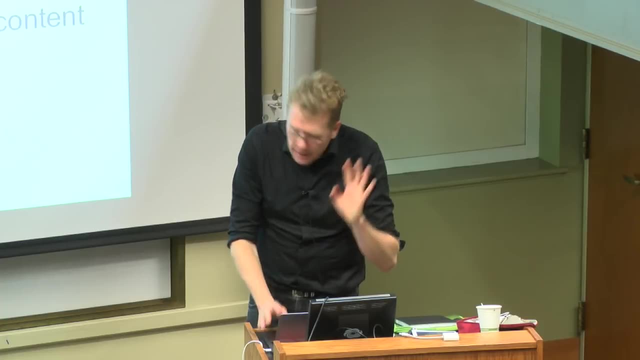 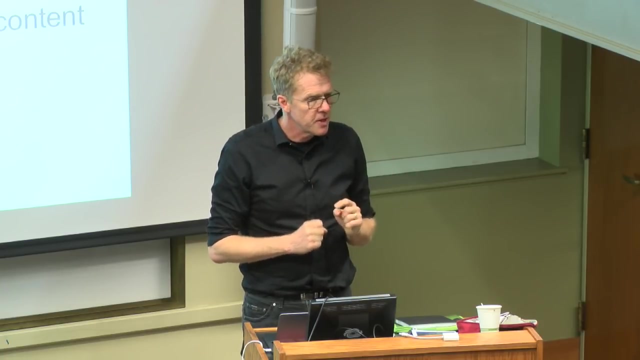 In the optimization out comes the covariance. The question is, if you know, what I kind of skirted is all of this spectra with the same labels have, or stars with the same labels have the same spectra- comma, if the label set is complete, right. 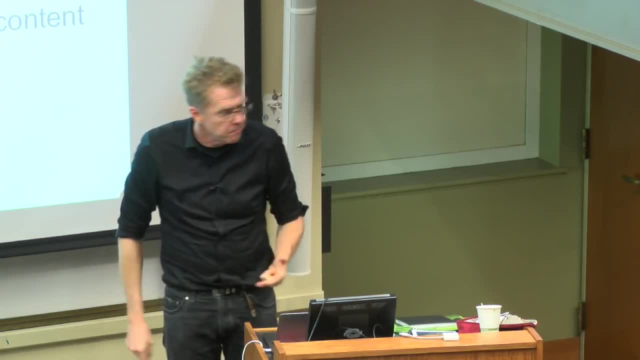 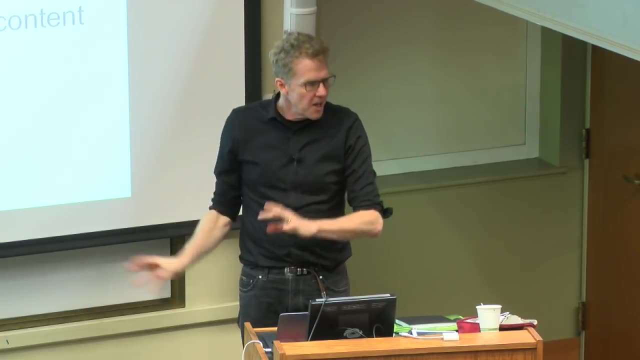 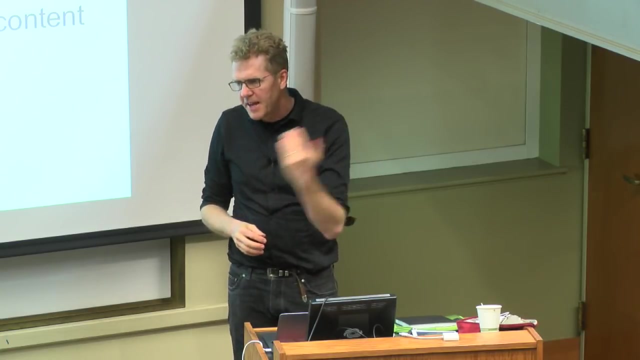 So if I only specify log gt- effective metallicity- but not alpha enhancement, then you can differ by that. So that's correct. So I think this is. you know, this is not a panacea that you can apply blindly. It is just a convenient tool that actually helps in the regimes that I described. 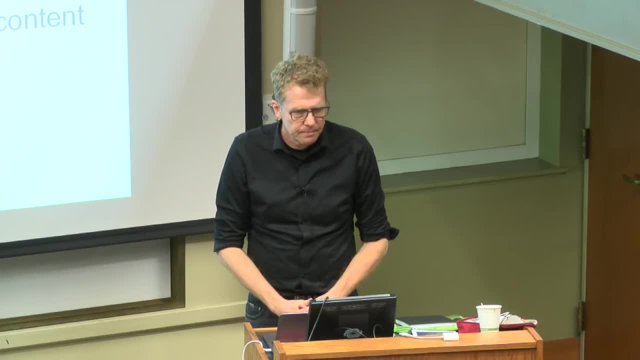 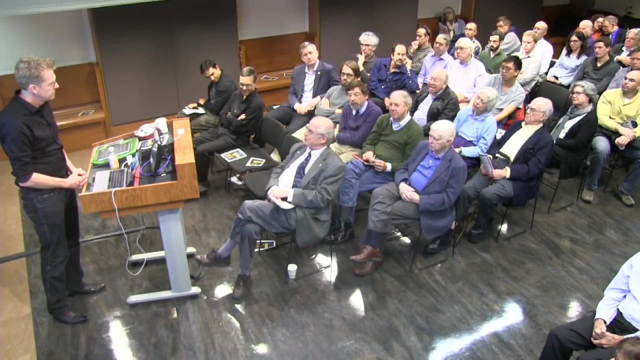 I couldn't help but notice that you mentioned tests, And I'm wondering if it's possible that the most important result from tests will be astroseismology for 10 or 20,000.. 10,000 giants all over the sky instead of planets. 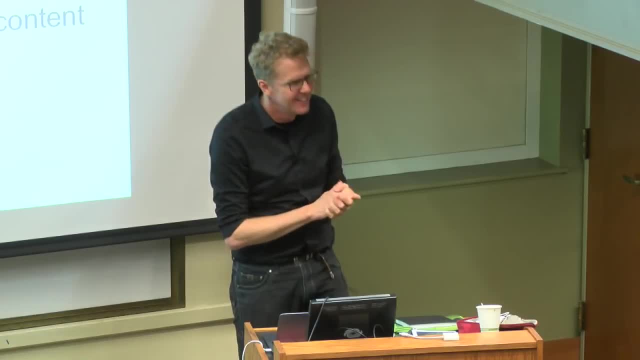 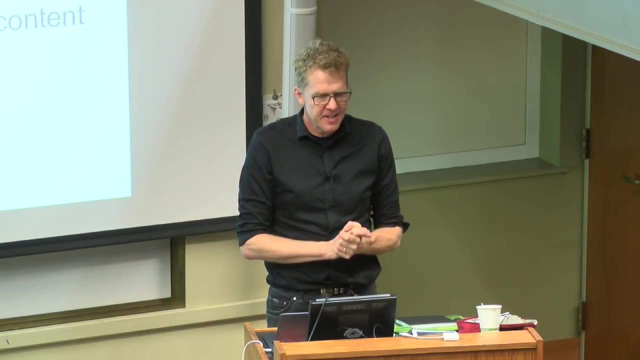 So this is being recorded. So what I'd like to say is that I, no, I, I. so let me just say that I actually do think that the astroseismology that will come from tests in the relatively near future will be: 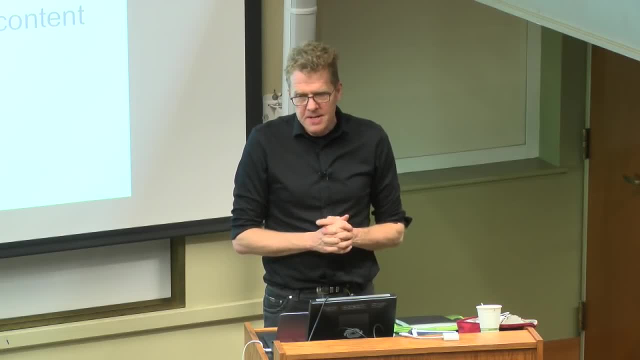 a blessing for exactly life. The other part. you know because there, let me just dwell on that for one second- Why. you know, even in the limit of infinite signal-to-noise we cannot in the spectra reproduce the astroseismic masses to better than point. you know point-modex mass. 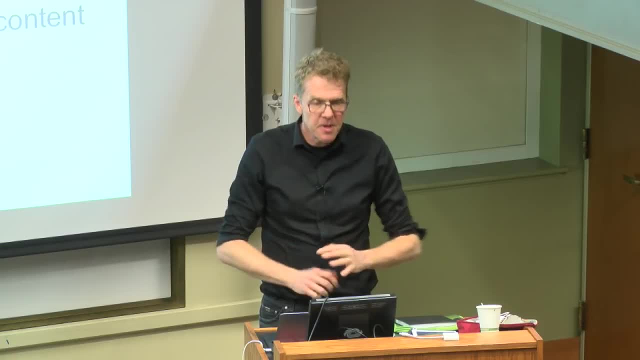 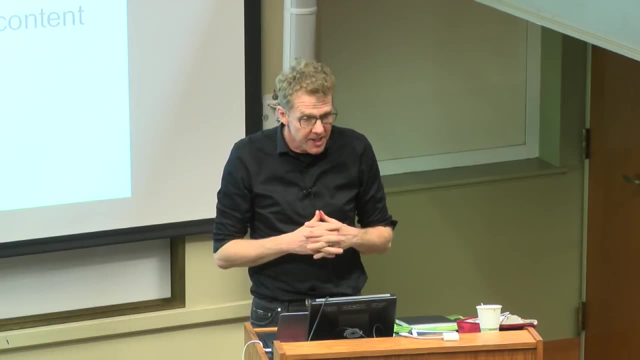 Is it because really there is a stochastic component that dredge up? Is it rotation involved, et cetera? right, I mean, I would actually like to develop an even better spectroscopic age indicator for giants. So there it will. 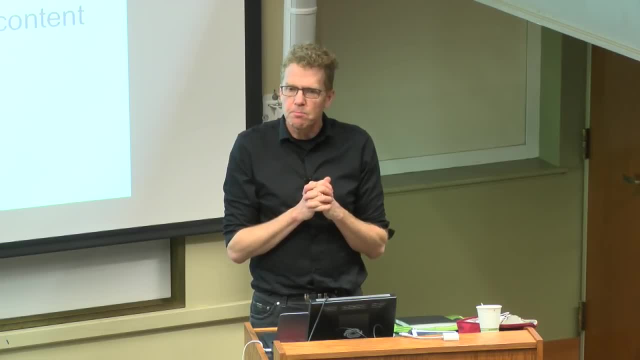 No, I do think both. by what? by citation, by the public perception. I am convinced that the transit from tests will be the most important result, and I actually think there's some also from a, you know, in moving forward. 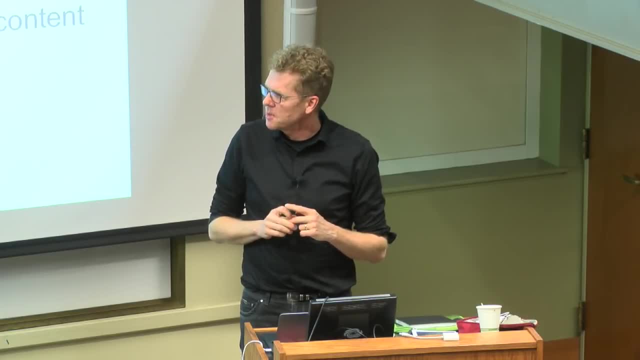 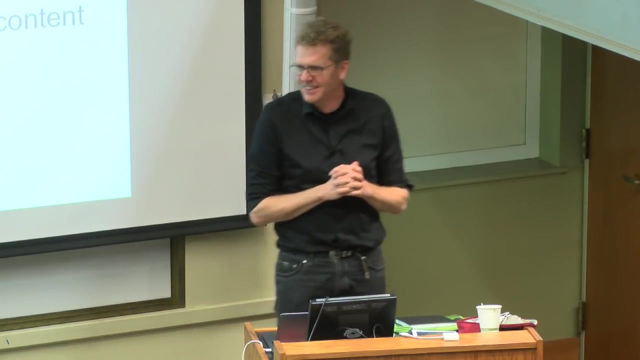 But I do think, in addition to stellar spectroscopy, astroseismology is a, I find, a very important and fascinating field that should have more fans on this continent. So I think, with that very gracious and thoughtful answer, I'd just like to thank our speaker again.